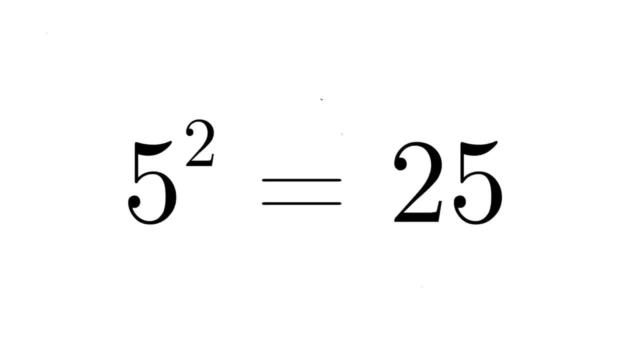 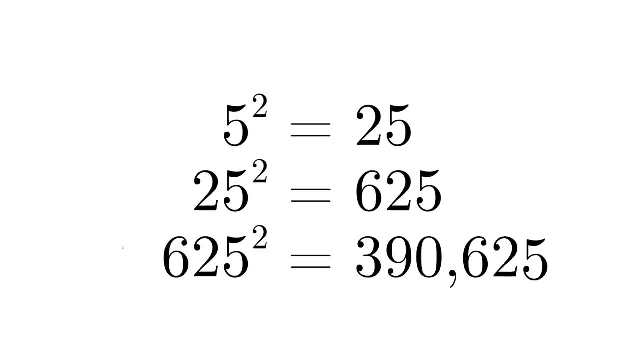 Take the number 5 and square it, You get 25.. Now take 25 and square it, You get 625.. Square 625 and you get 390,625.. Do you see the pattern? 5 squared ends in a 5,. 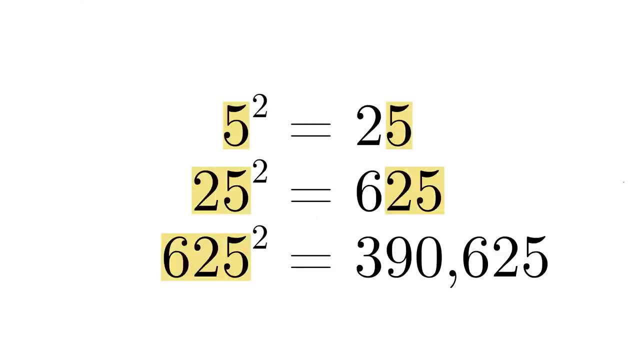 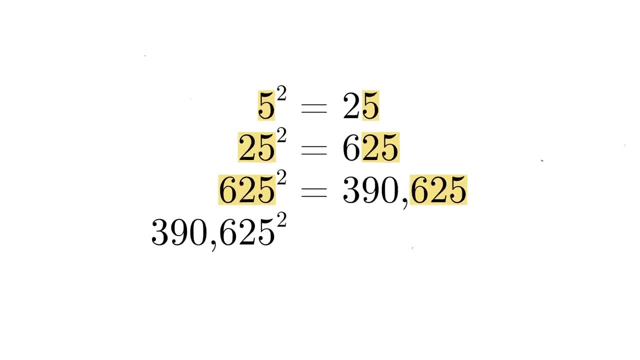 25 squared ends in 25, and 625 squared ends in 625.. So does this pattern continue? Well, let's try squaring 390,625.. It doesn't quite end in itself, but the last 5 digits match. 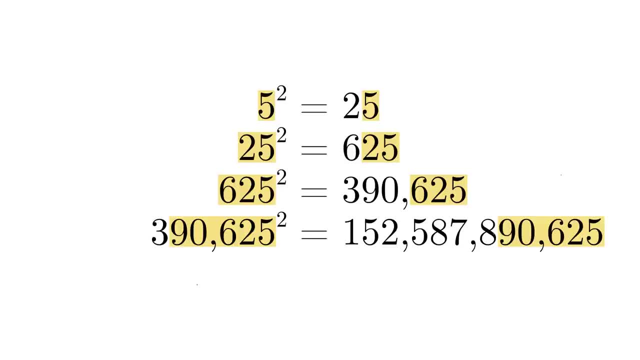 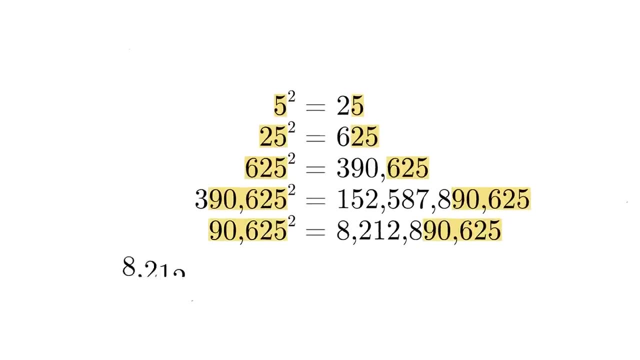 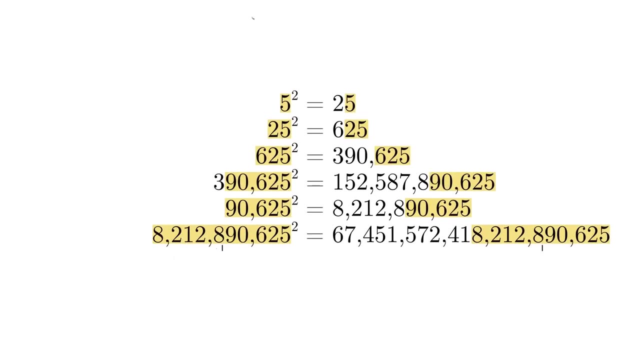 so it extends the pattern by a few places. So let's try squaring just that part: 90,625.. That does end in itself, And if we square that whole number it also ends in itself. And now we're up to 10 digits, And you can keep doing this. 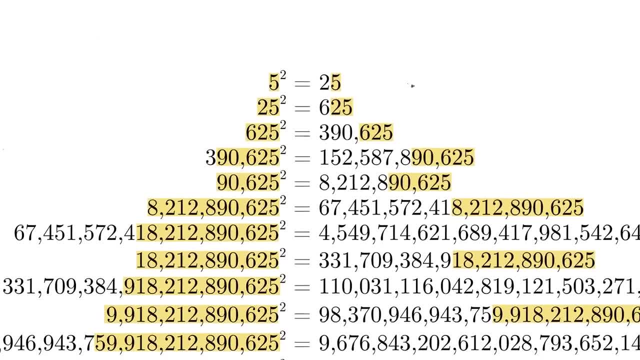 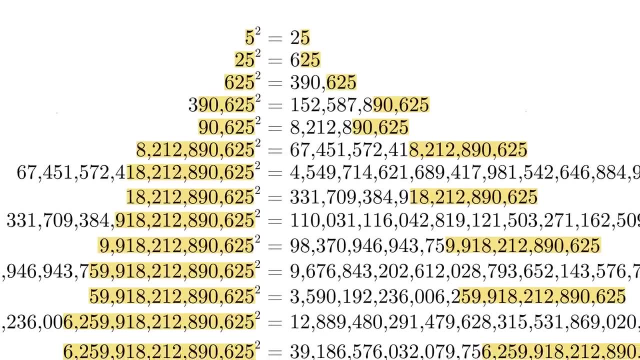 squaring the part of the answer that matches the previous number and including the part that matches the previous number By increasing the number of digits they share in common. it's as though we are converging on a number, But not in the usual sense of convergence. This number will have infinite digits, And if you 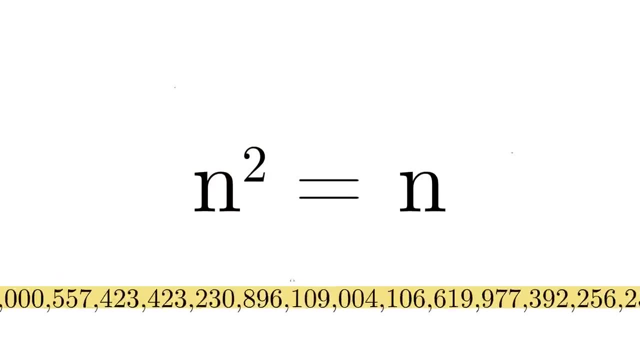 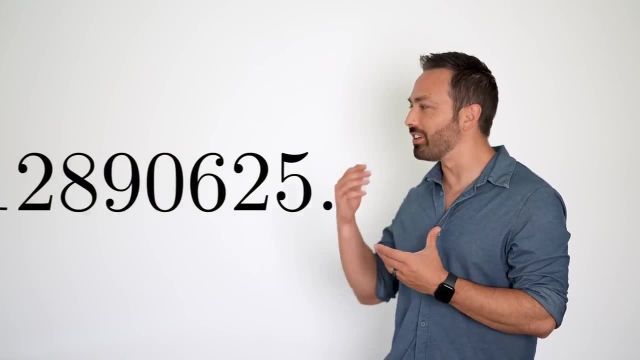 square it, you'll get back that same number. The number is its own square. Now I bet you're thinking: does it even make sense to talk about numbers that have infinite digits going off to the left of the decimal point? I mean, isn't that just infinity In this video? 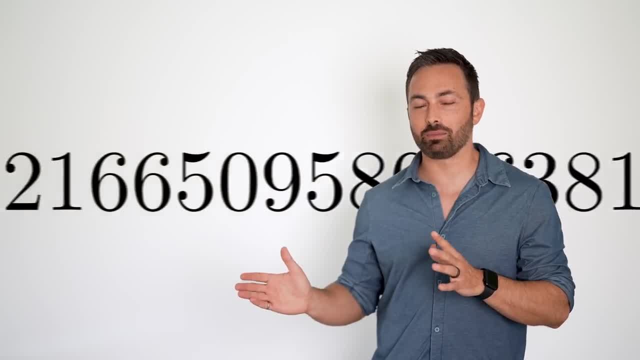 my goal is to give you an idea of how to do that. If you're interested in learning more about these numbers. I want to convince you that such numbers do make sense. They just belong to a number system that works very differently from the one we're used to And that allows these numbers. 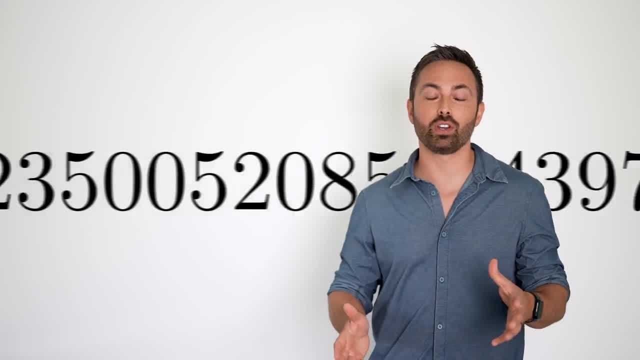 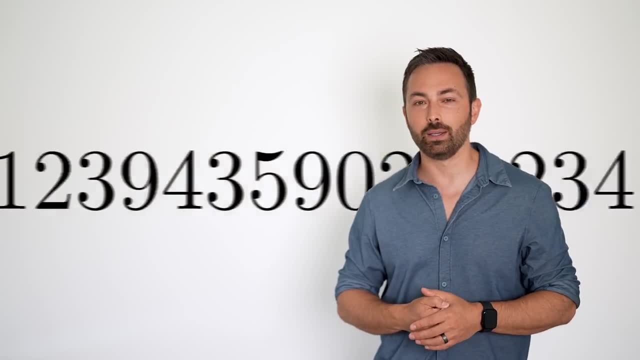 to solve problems that are impenetrable using ordinary numbers, which is why they are a fundamental tool in cutting edge research today in number theory, algebraic geometry and beyond. So let's start by looking at the properties of the number system that includes the number we just 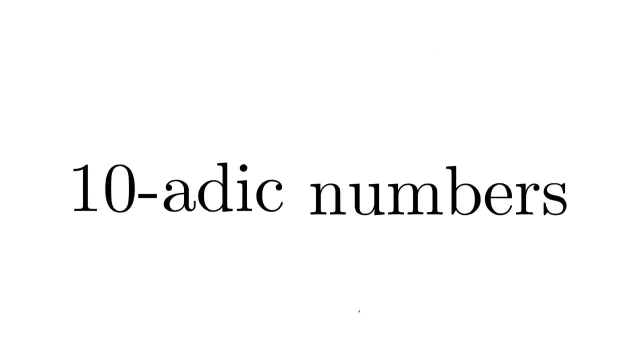 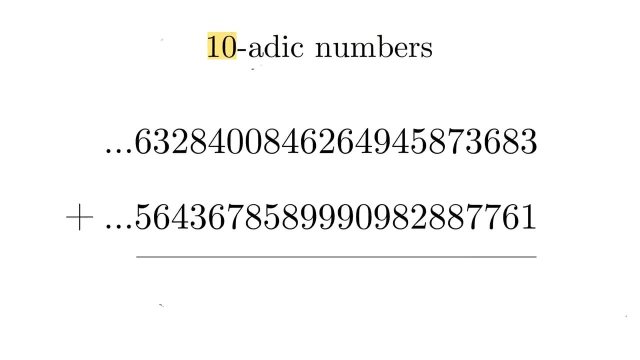 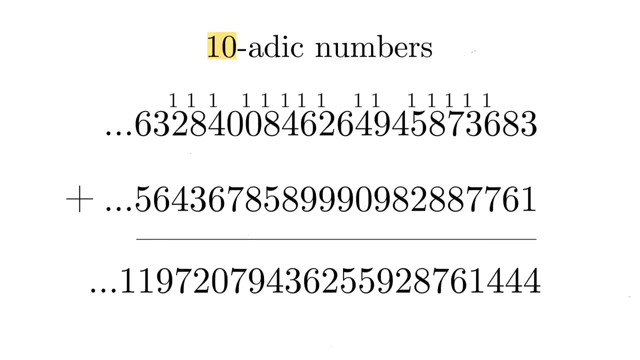 found. We'll call these 10-adic numbers because they're written with the same number. So if you have two 10-adic numbers, can you add them together? Sure, You just go digit by digit from the right to the left, adding them up as usual. Addition is not a problem. What about multiplication? 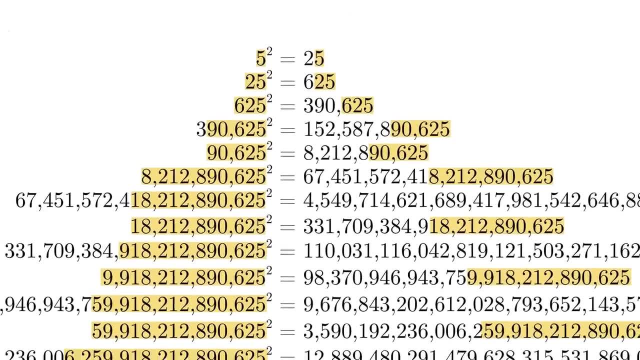 the number of digits they share in common. It's as though we are converging on a number, but not in the usual sense of convergence. This number will have infinite digits, And if you square it, you'll get back that same number. 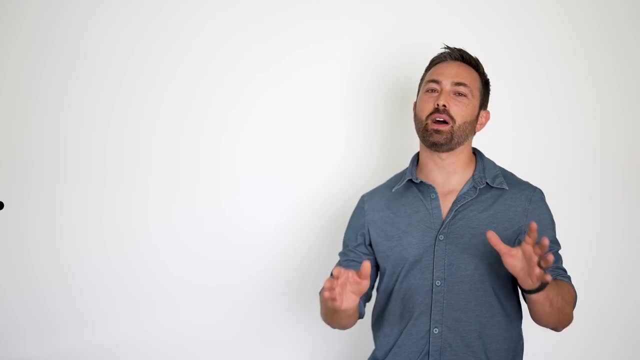 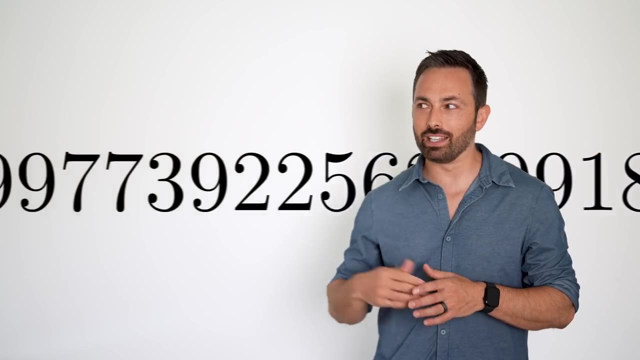 The number is its own square. Now I bet you're thinking: does it even make sense to talk about numbers that have infinite digits going off to the left of the decimal point? I mean, isn't that just infinity? In this video, my goal is to convince you. 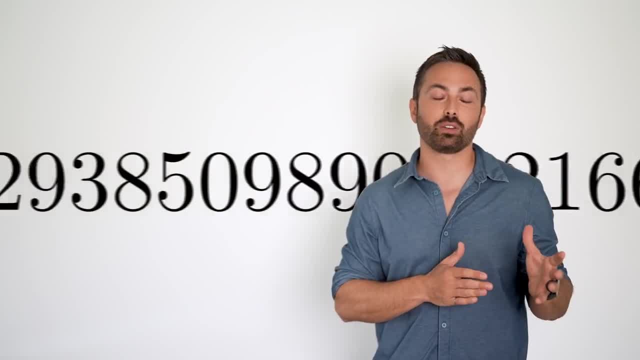 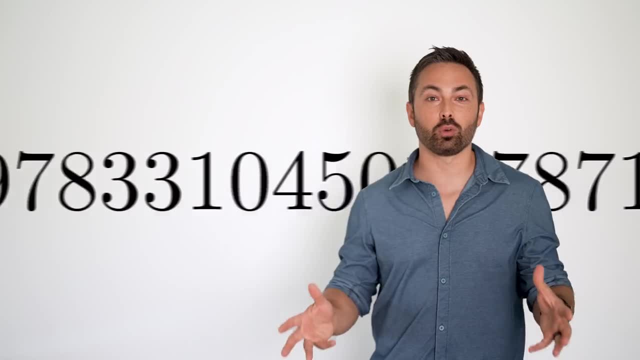 that such numbers do make sense. They just belong to a number system that works very differently from the one we're used to And that allows these numbers to solve problems that are impenetrable using ordinary numbers, which is why they are a fundamental tool. 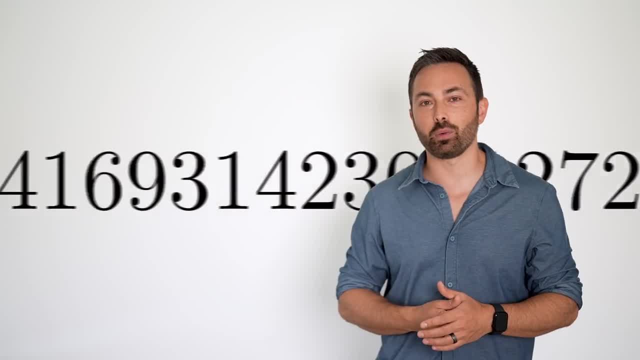 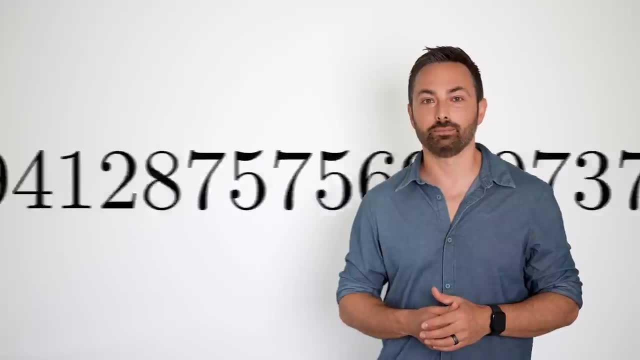 in cutting-edge research today in number theory, algebraic geometry and beyond. So let's start by looking at the properties of the number system that includes the number we just found. We'll call these 10-adic numbers Because they're written in base 10.. 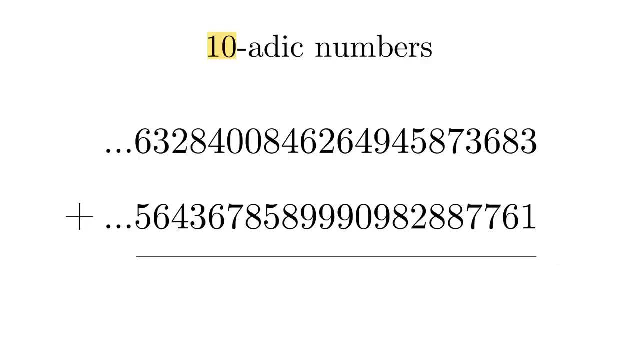 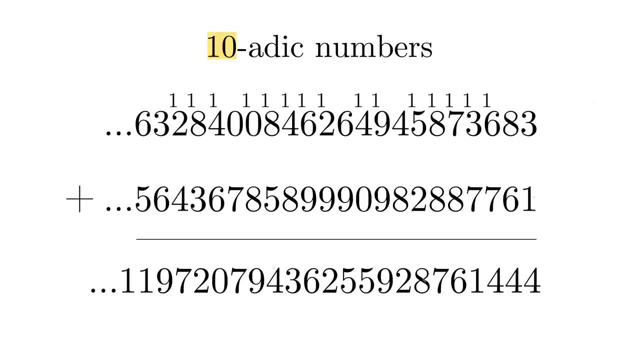 If you have two 10-adic numbers, can you add them together? Sure, You just go digit by digit from the right to the left, adding them up as usual. Addition is not a problem. What about multiplication? Well, again, you can take any two 10-adic numbers. 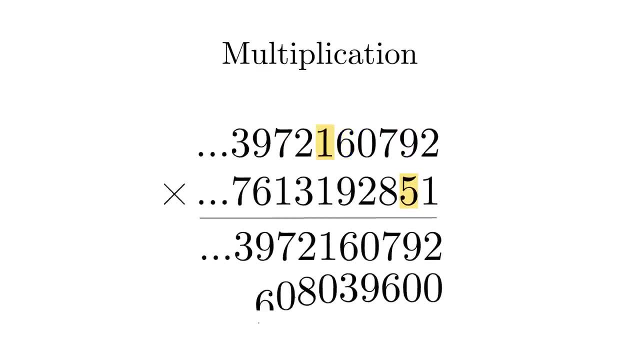 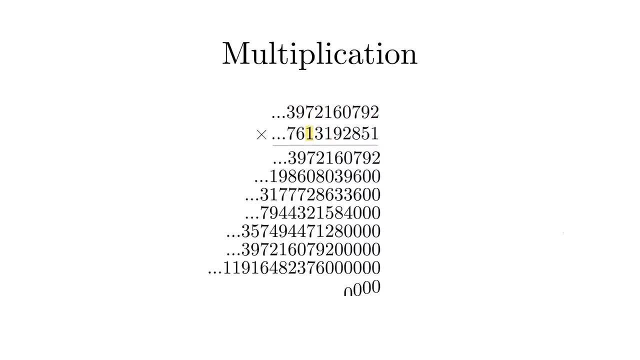 and multiply them out. This works because the last digit of the answer depends only on the last digits of the 10-adic numbers, And subsequent digits depend only on the numbers to their right. So it might take a lot of work, but you can keep going for as many digits as you like. 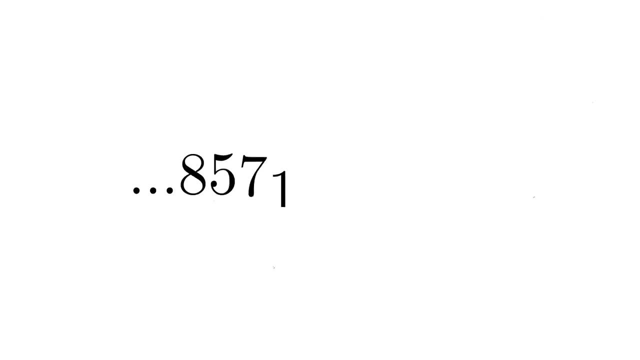 Let's take one 10-adic number ending in 857142857143 and multiply it by seven. So seven times three is 21,. carry the two. Seven times four is 28,. plus two makes 30,. carry the three. 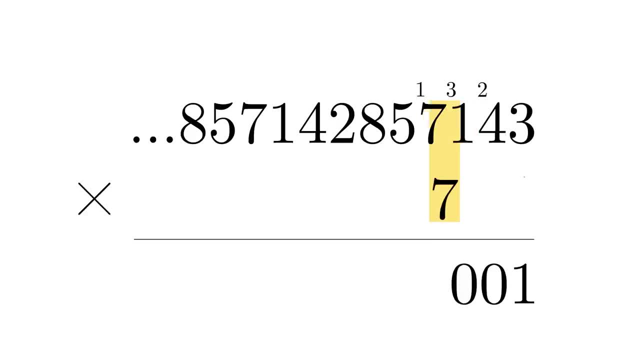 Seven times one is seven. plus three makes 10,. carry the one Seven times seven is 48, plus three makes 10,. carry the one Seven times four is 49, plus one is 50,. carry the five Seven times five is 35, plus five is 40,. carry the four. 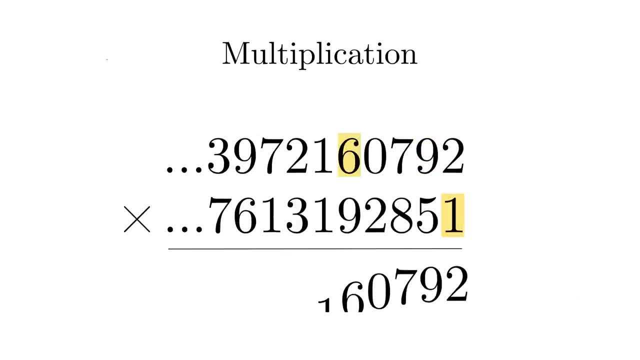 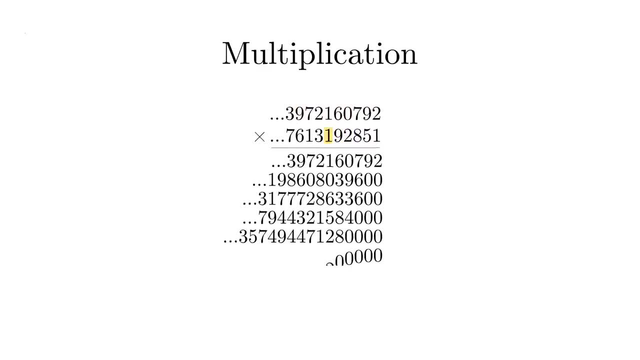 Well, again, you can take any two 10-adic numbers and multiply them out. This works because the last digit of the answer depends only on the last digits of the 10-adic numbers and subsequent digits depend only on the numbers to their right. So it's not a problem if you have two 10-adic numbers. 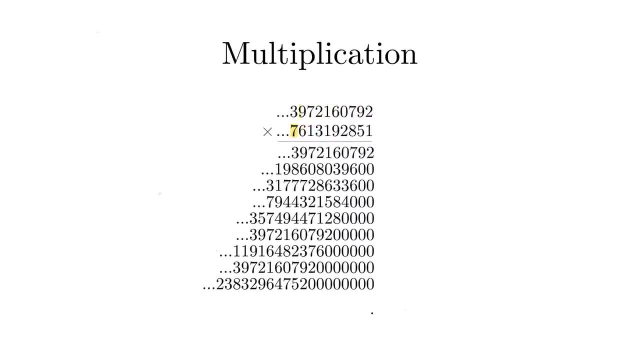 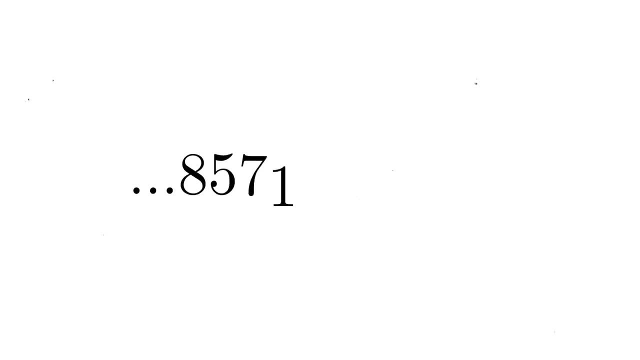 so it might take a lot of work, but you can keep going for as many digits as you like. Let's take one 10-adic number ending in 857142857143 and multiply it by 7. So 7 times 3 is 21,. 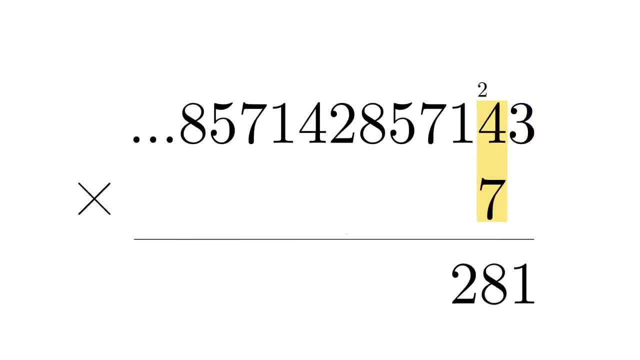 carry the 2.. 7 times 4 is 28, plus 2 makes 30,. carry the 3.. 7 times 1 is 7, plus 3 makes 10,. carry the 1.. 7 times 7 is 49, plus 1,. 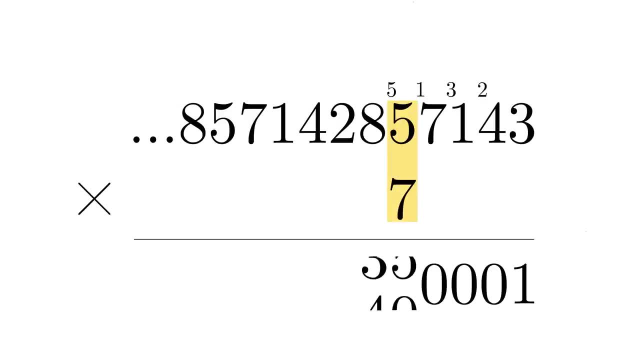 is 50,. carry the 5.. 7 times 5 is 35, plus 5 is 40,. carry the 4.. And you can keep going forever and you'll find all the other digits are 0. So this number times 7 equals 1,. 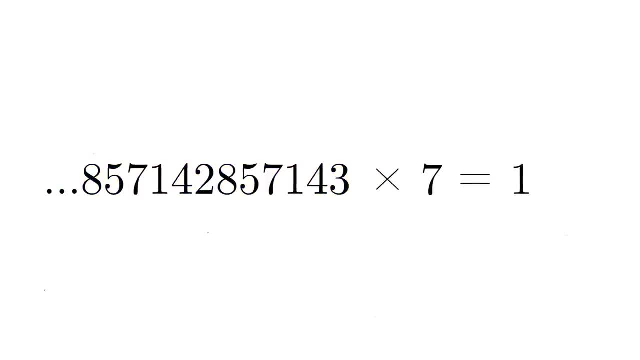 which means this 10-adic number must be equal to 1- 7th. What we have just found is that there are rational numbers, fractions, in the 10-adic numbers, without having to use the divided by numbers. So we can just multiply them by 7, which means that there are rational numbers fractions. 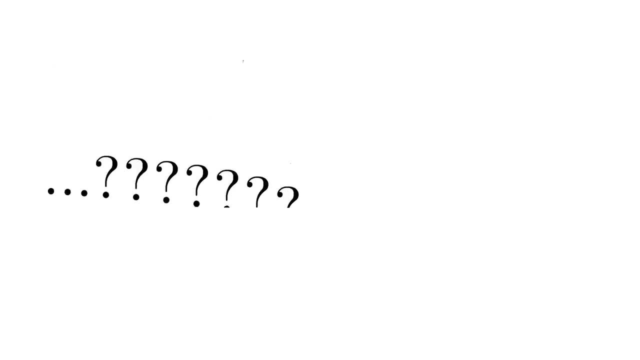 in the 10-adic numbers without having to use the divided by numbers. So we can just multiply them by 7, which means that there are rational numbers, fractions, in the 10-adic numbers without having to use the divided by symbol. Say, you want to find the 10-adic number that equals a third. How would you do it? 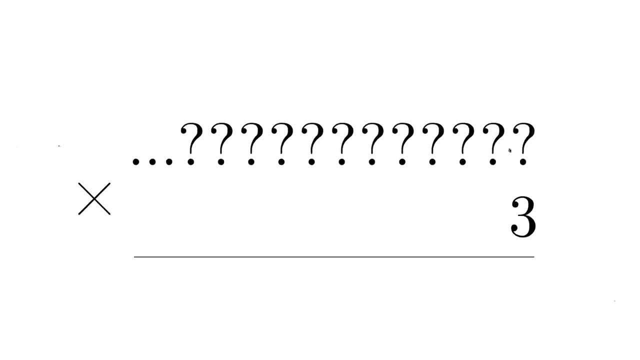 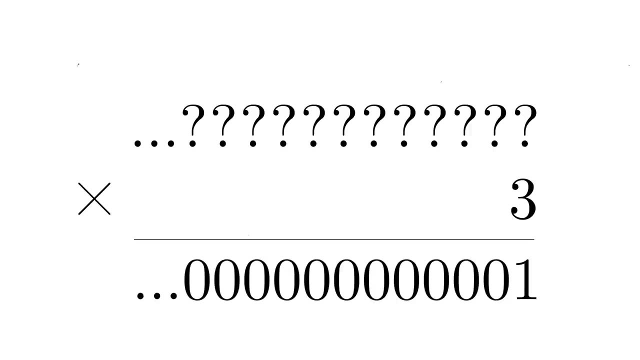 Well, let's imagine we have an infinite string of digits and when we multiply them by 3, we get 1.. This implies that all the digits to the left of the 1 must be 0. So what do we multiply 3 by to get a 1 in the units place? Well, 3 times 7 is 21,, so that gives us the 1, and then we carry. 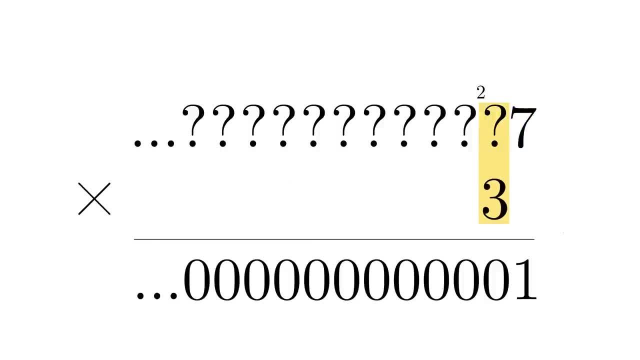 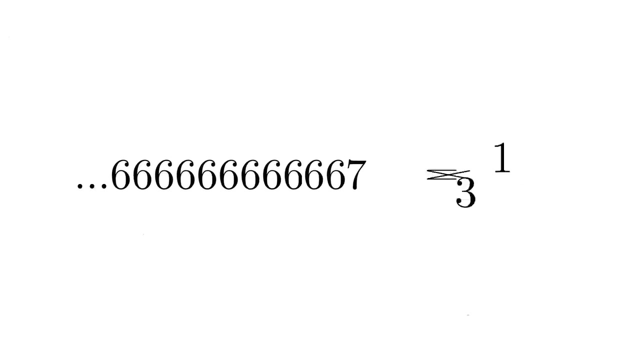 the 2.. Now, what times 3 plus 2?? Well, 3 times 7 is 21,. so that gives us the 1, and then we carry the 2.. Now, what times 3 plus 2 gives us a 0? 6.. 3 times 6 equals 18, plus 2 equals 20, so we have a 0, and we carry the 2.. Put another 6 there and we get another 20 again. So if we put a string of 6s all the way to the left, they will all multiply to make 0. So an infinite string of 6s, and 1- 7 is equal to 1. 3rd, 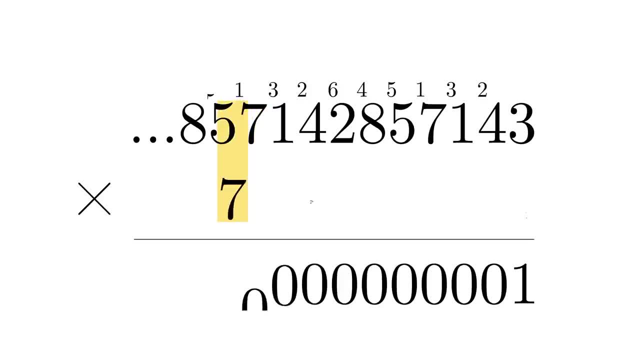 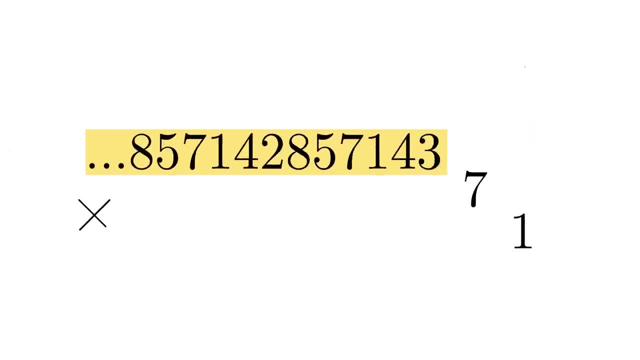 And you can keep going forever and you'll find all the other digits are zero. So this number times seven equals one, which means this 10-adic number must be equal to 1: 7th. What we have just found is that there are rational numbers. 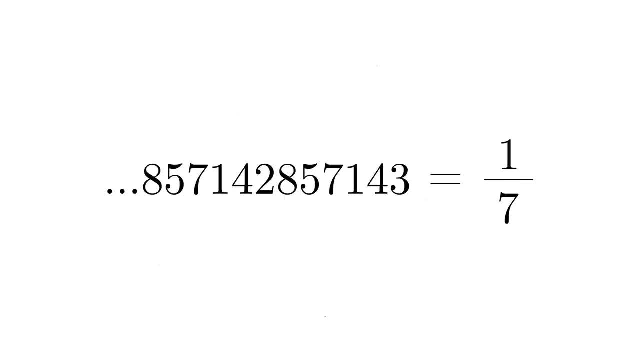 fractions in the 10-adic numbers without having to use the divided by symbol. Say you want to find the 10-adic number that equals a third. How would you do it? Well, let's imagine we have an infinite string of digits. 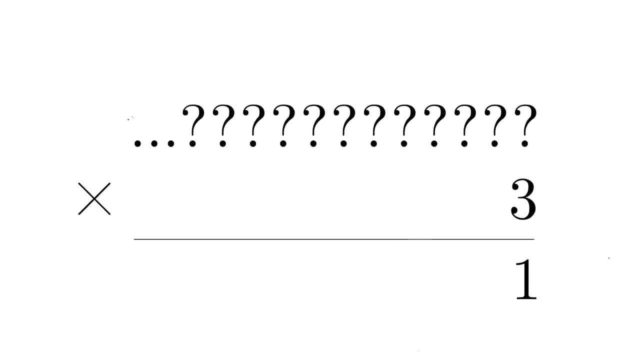 and when we multiply them by three, we get one. This implies that all the digits to the left of the one must be zero. So what do we multiply three by to get a one in the units place? Well, three times seven is 21,. so that gives us the one. 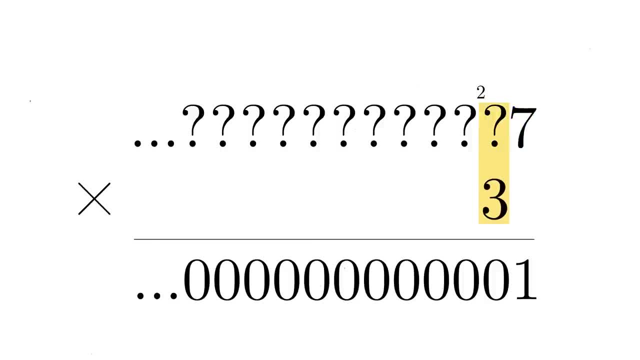 and then we carry the two. Now what times three plus two gives us a zero, Six. Three times six equals 18, plus two equals 20, so we have a zero and we carry the two. Put another six there and we get another 20 again. 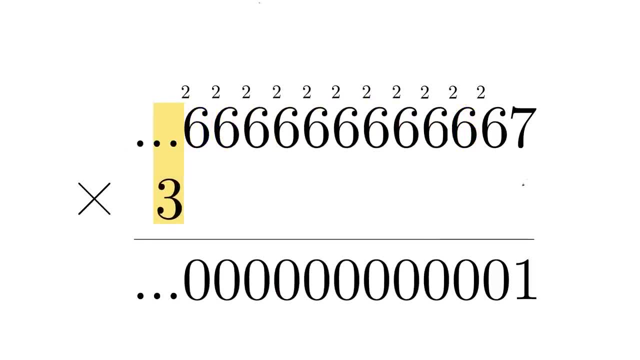 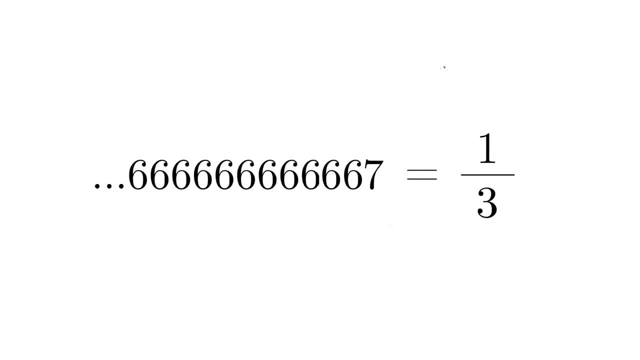 So if we put a string of sixes all the way to the left, they will all multiply to make zero. So an infinite string of sixes and one seven is equal to 1- 3rd. This looks similar to the infinite digits we're used to going off to the right side of that grid. 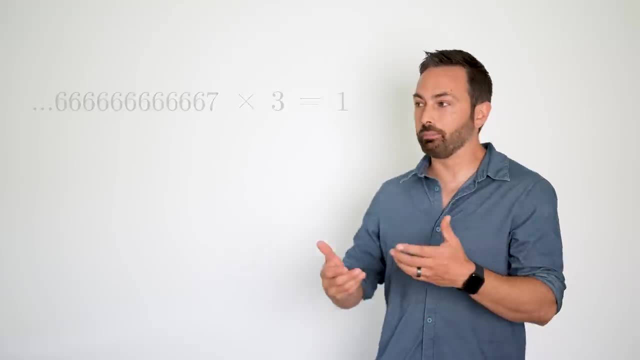 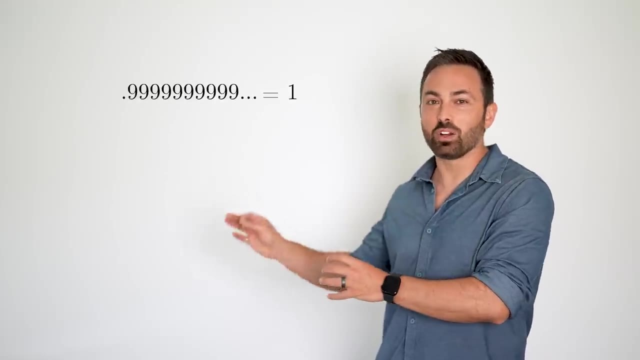 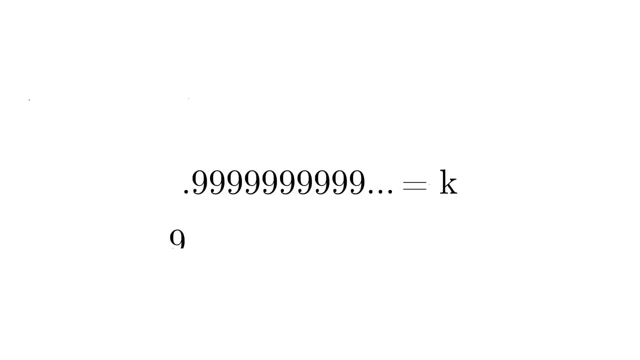 看 ключ Yoo of the decimal point like point nine, nine, nine, nine, nine, nine, nine, repeating: what does this equal? well, I'll claim that it's exactly equal to one. but how do we prove it? let's call this number K and then multiply both sides by 10. so 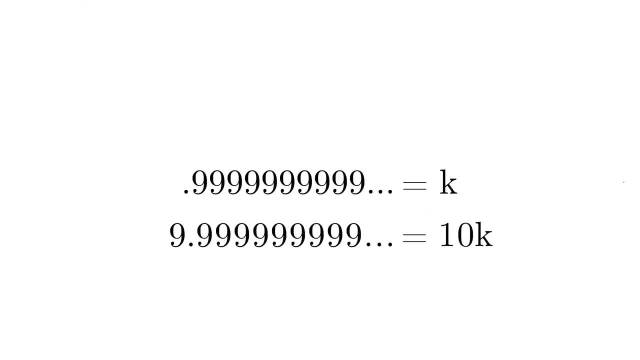 now we've got nine point nine. nine, nine repeating equals 10 K. now subtract the top equation from the bottom one to get 9 equals 9 K. so K equals 1. this is a fairly standard argument for why point nine, nine, nine repeating must be exactly. 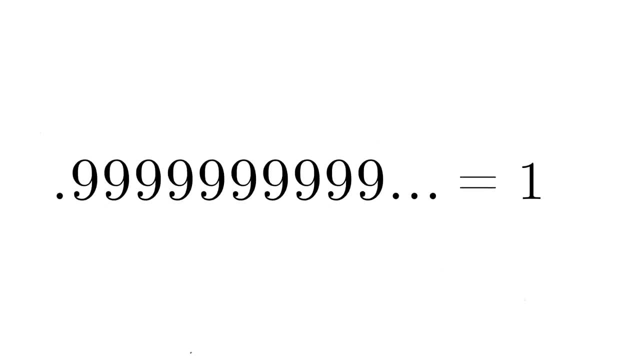 equal to one. but what if, instead of going to the right of the decimal place, the nines went to the left of the decimal place? that is a tenadic number of all nines. what does this number equal? well, we can do the same thing: set it. 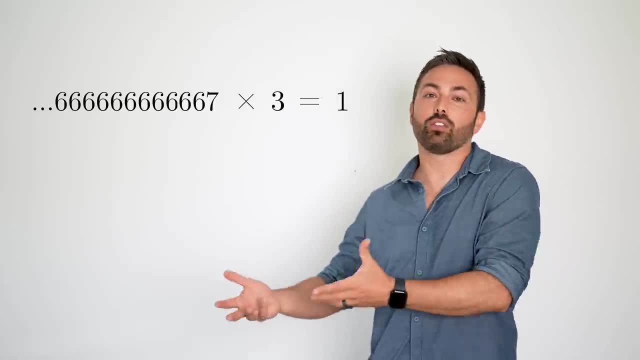 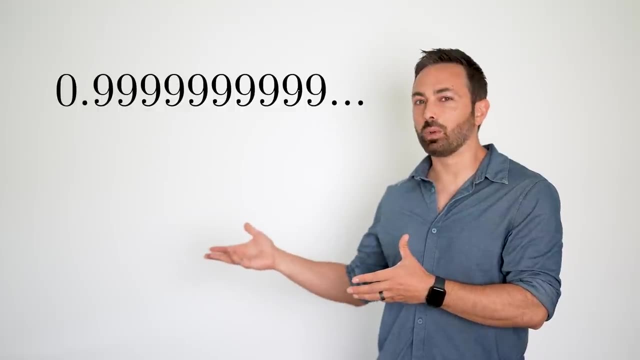 This looks similar to the infinite digits we're used to going off to the right of the decimal point, Like 0.99999999. repeating: What does this equal? Well, I'll claim that it's exactly equal to 1, but how do we prove it? 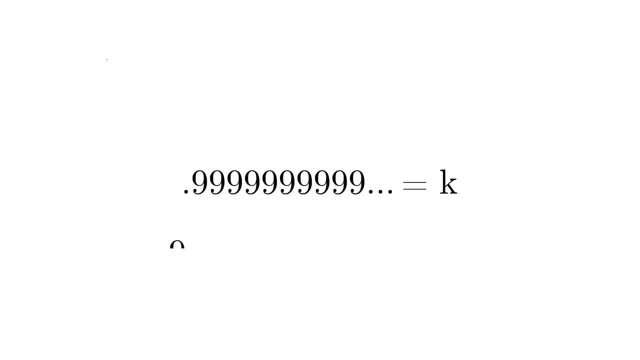 Let's call this number k and then multiply both sides by 10.. So now we've got 9.9999. repeating equals 10k. Now subtract the top equation from the bottom one to get 9 equals 9k. 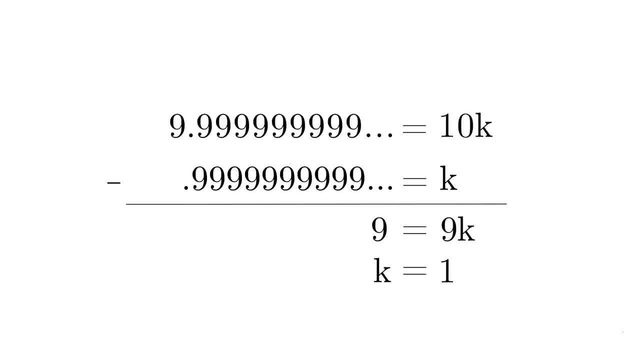 So k equals 1.. This is a fairly standard argument for why 0.999 repeating must be exactly equal to one. But what if, instead of going to the right of the decimal place, the 9s went to the left of the decimal place? 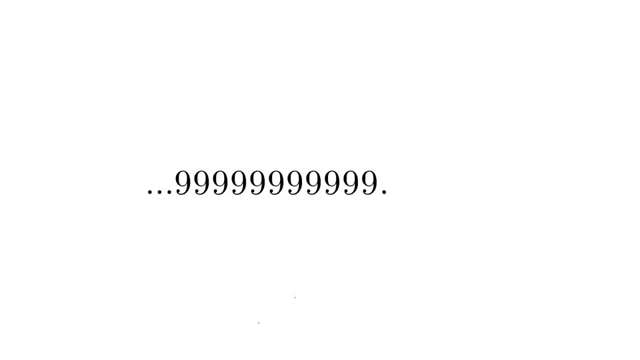 That is a 10adic number of all 9s. What does this number equal? Well, we can do the same thing. Set it equal to say m, and then multiply both sides by 10.. So we have 999999990 equals 10m. 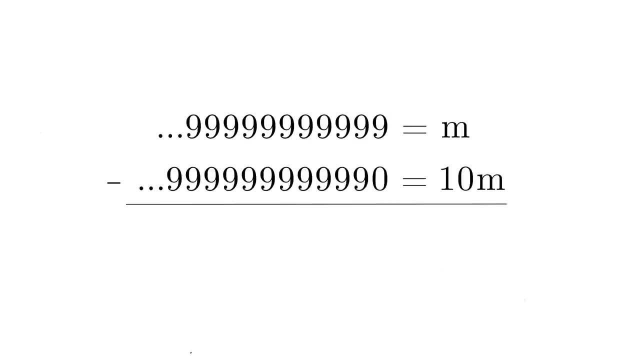 Now subtract this equation from the first one, first one, and we get: 9 equals negative 9m, meaning m equals negative 1.. So this tenadic string of all 9s is actually negative 1.. Now I know that seems weird, so let's try adding 1 to it. 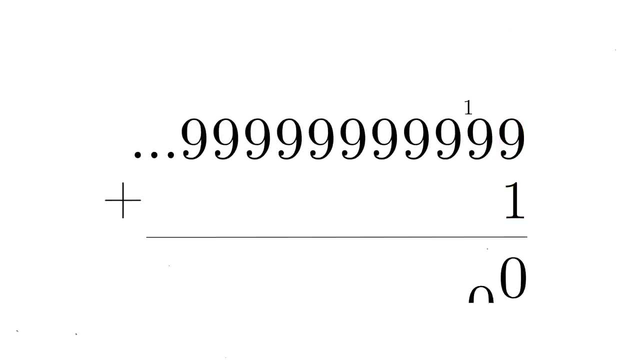 Well, 9 plus 1 is 10,, carry the 1,. 9 plus 1 is 10,, carry the 1, and you just keep doing this all the way down the line and every digit becomes 0.. I know, it seems like at some point you're going to end up with a 1 all the way down. 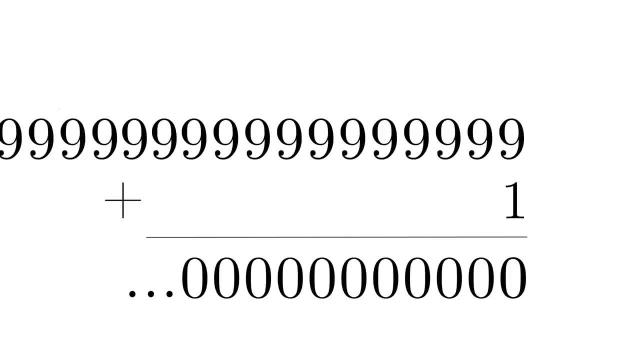 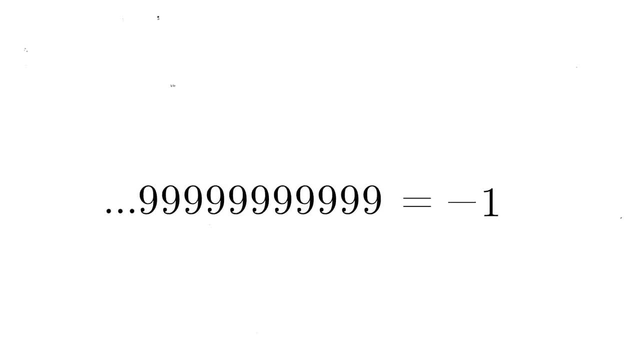 on the left, but this never happens because the 9s go on forever. All 9s plus 1 equals 0, therefore all 9s must be equal to negative 1.. This also means that all 9s and then say a 3 equals negative 7.. 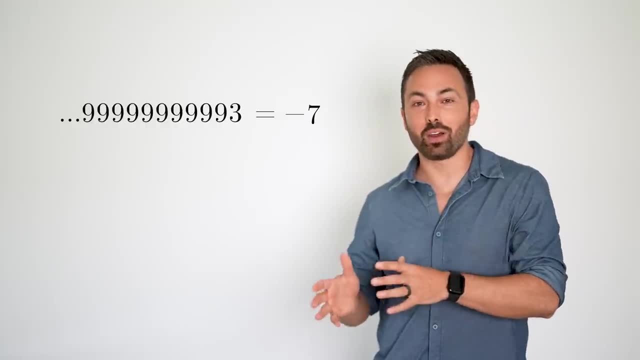 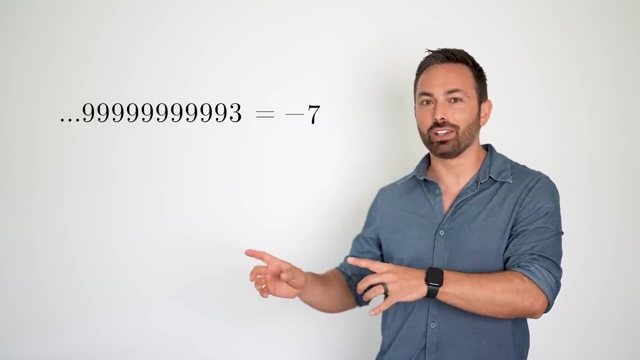 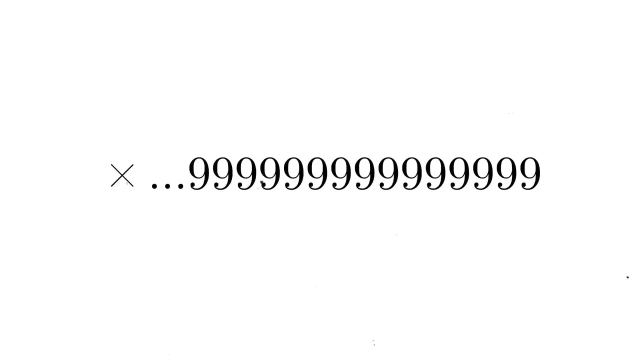 What we have just discovered is that the tenadics contain negative numbers as well. You don't need a negative sign By the structure of these numbers alone. negatives are impossible To do subtraction, you just add the negative of that number. To find the negative of any tenadic number, you could multiply by all 9s or just perform. 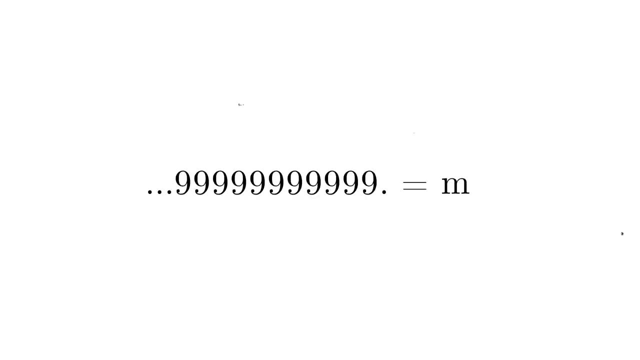 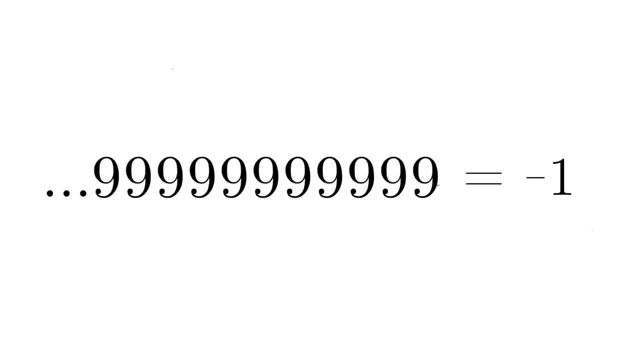 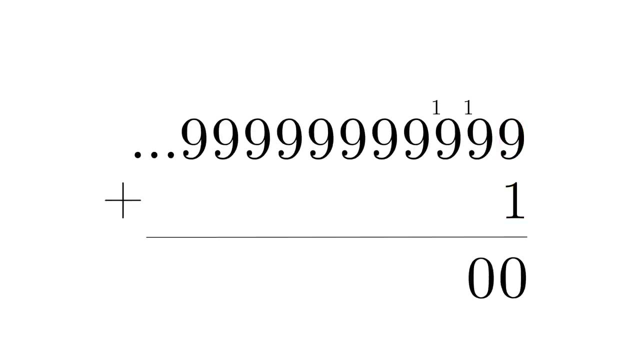 negative 1. now I know that seems weird, so let's try adding 1 to it. well, 9 plus 1 is 10. carry the 1. 9 plus 1 is 10, carry the 1. and you just keep doing this all the way down the line and every digit becomes zero. 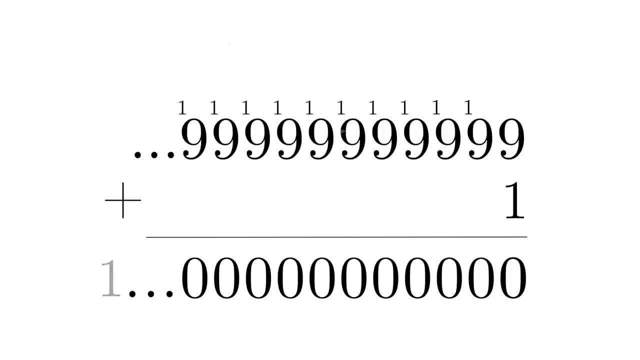 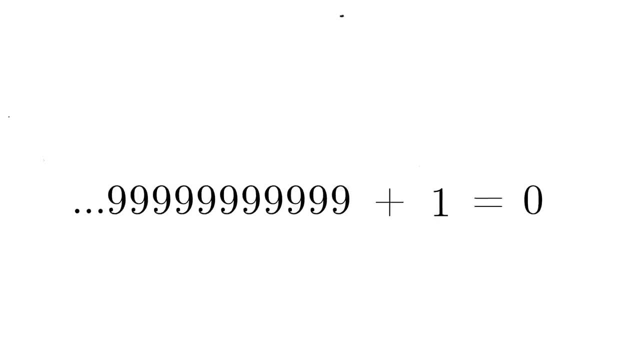 you know, it seems like at some point you're gonna end up with a 1 all the way down on the left, but this never happens because the nines go on forever. all nines plus 1 equals 0. therefore, all nines must be equal to negative 1. this also means: 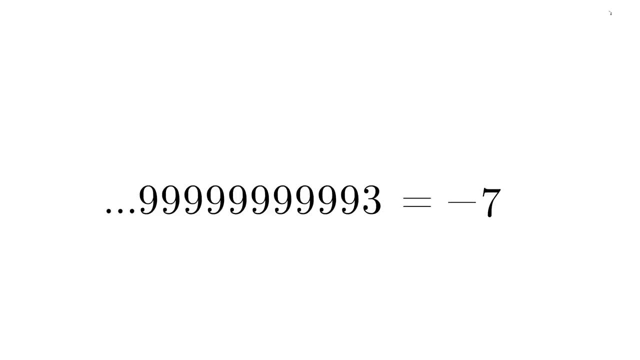 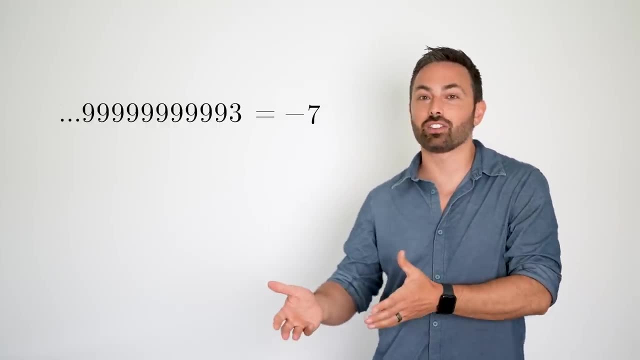 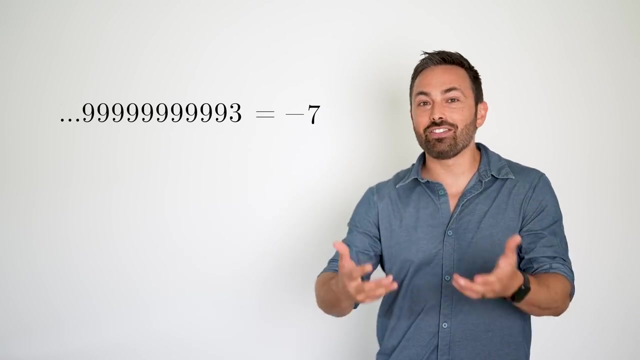 that all nines and then say a 3 equals negative 7. what we have just discovered is that the ten addicts contain negative numbers as well. you don't need a negative sign by the structure of these numbers alone. negatives are included. to do subtraction, you just add the negative of that number to find the 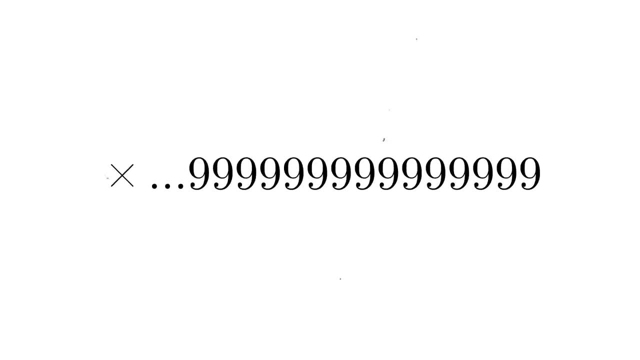 negative of any ten addict number. you could multiply by all nines or just perform these two steps: first take the nines complement, that is the difference between each digit and 9, and then add 1. so if this number is 1, 7th, then negative. 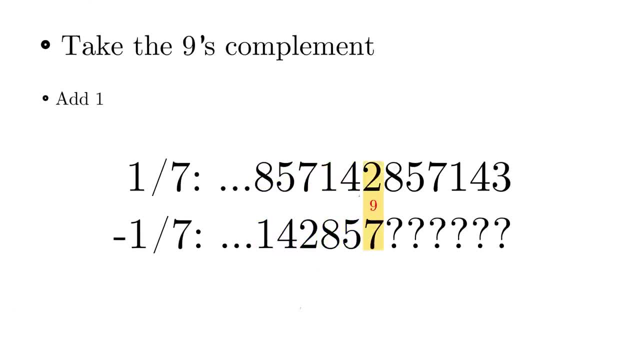 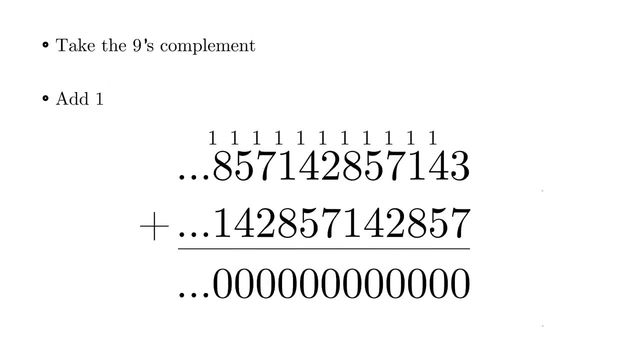 a 7th is 1, 4, 2, 8, 5, 7, 1, 4, 2, 8, 5, 6 plus 1, and we can verify that this is indeed negative a 7th by adding it to positive 1 7th and finding that these numbers annihilate each other to 0. so to sum up, 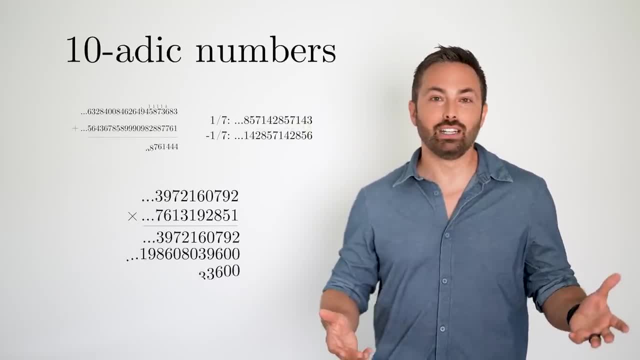 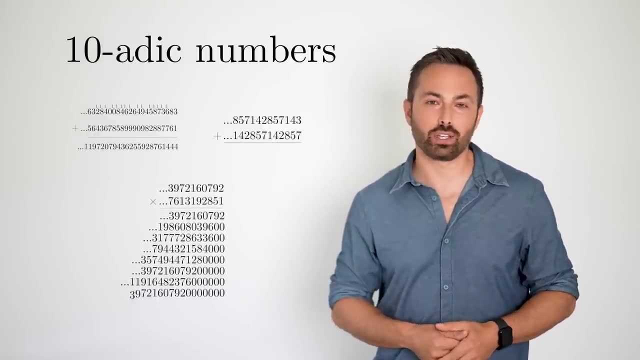 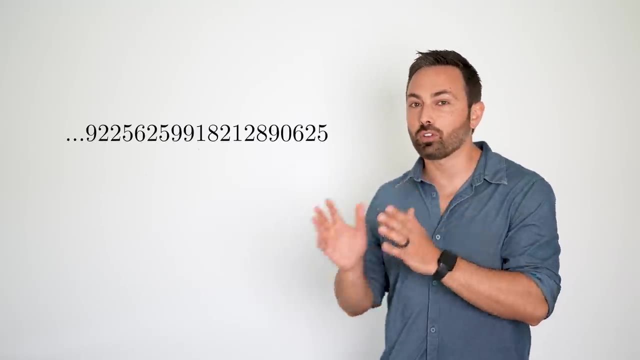 ten addict numbers can be added, subtracted, multiplied and they work exactly as you'd expect. plus, they contain fractions and negative numbers without having to use additional symbols. there is just one big problem, and you can see it with the first ten addict number we found. remember, if you multiply. 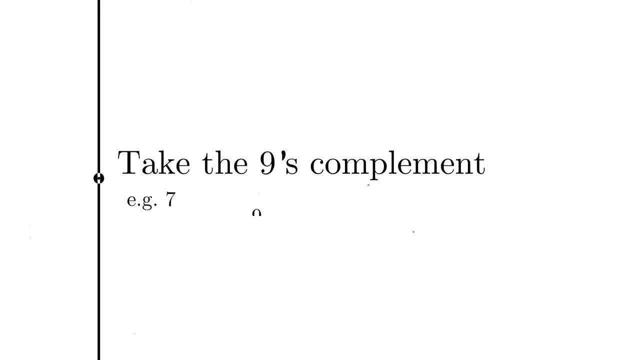 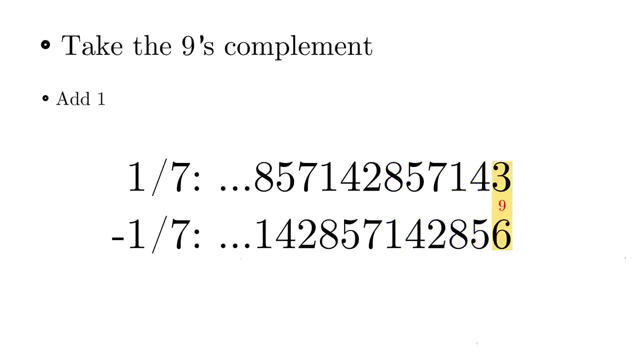 these two steps: First take the 9s complement, that is the difference between each digit and 9, and then add 1.. So if this number is 1 seventh, then negative a seventh is 1, 4, 2, 8, 5, 7, 1, 4, 2, 8, 5, 6 plus. 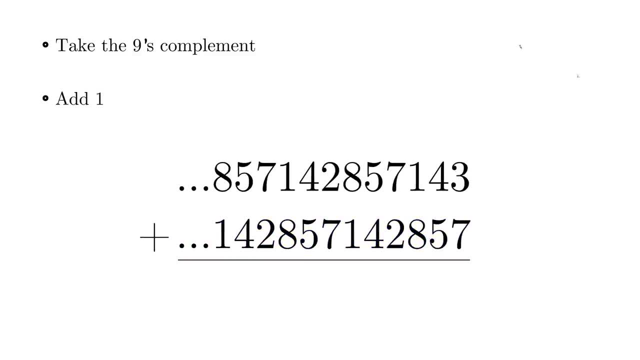 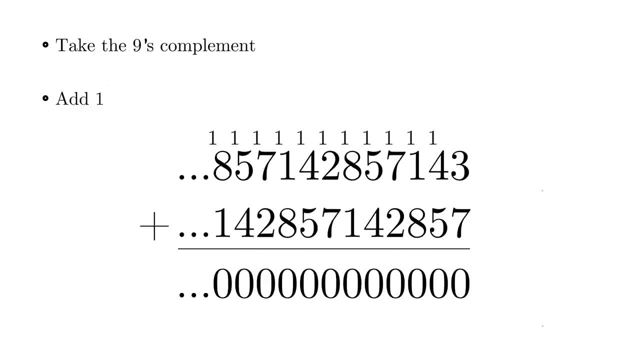 1. And we can verify that this is indeed negative a seventh by adding it to positive 1 seventh and finding that these numbers annihilate each other to zero. So to sum up, tenadic numbers can be added, subtracted, multiplied and they work exactly. 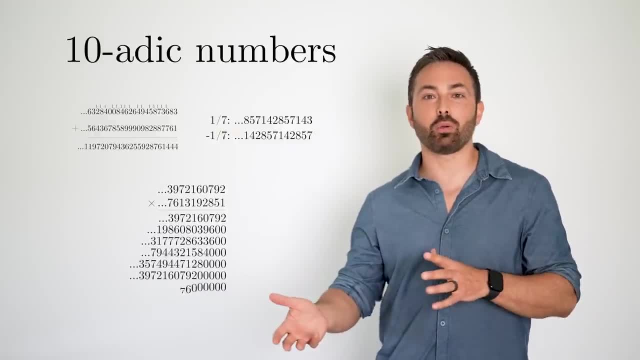 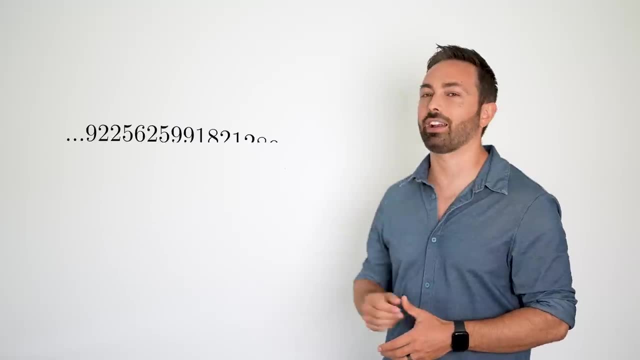 as you'd expect. Plus, they contain fractions and negative numbers without having to use additional symbols. There is just one big problem, and you can see it with the first tenadic number we found. Remember, If you multiply this number by itself, you get back that same number. 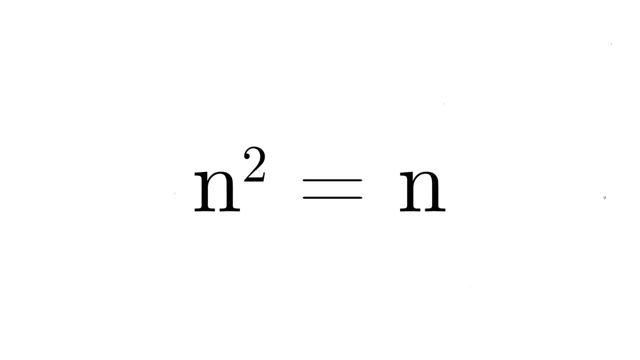 This number is its own square And that's a problem which you can see. if we move the n to the left hand side and factor it Well, then we have n times n minus 1 equals 0. The numbers 0 or 1 would satisfy this equation, but our tenadic number is not 0 or 1.. 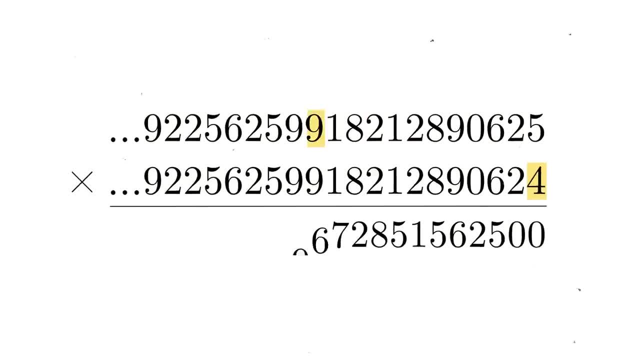 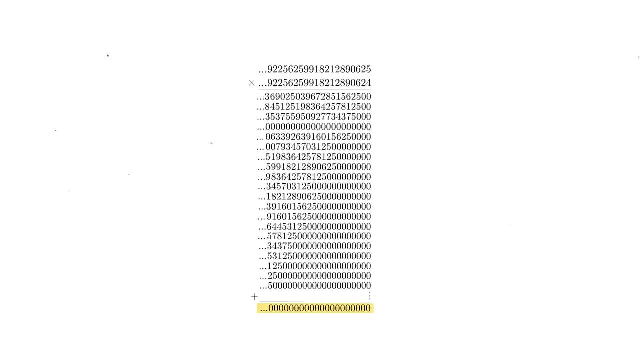 You can even verify by multiplying it out. this number, n times n minus 1, really does work out to 0.. This breaks one of the tools mathematicians rely on to solve equations. Have you ever thought about why, when faced with some complicated equation, we move all? 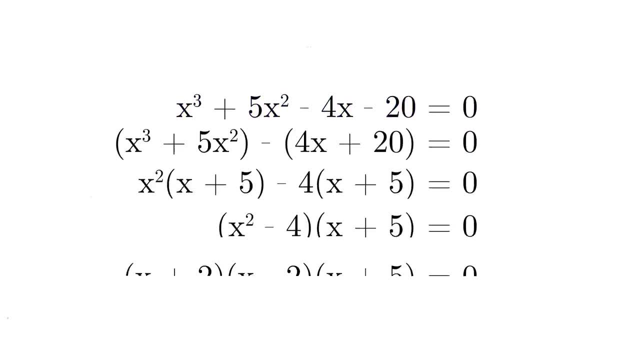 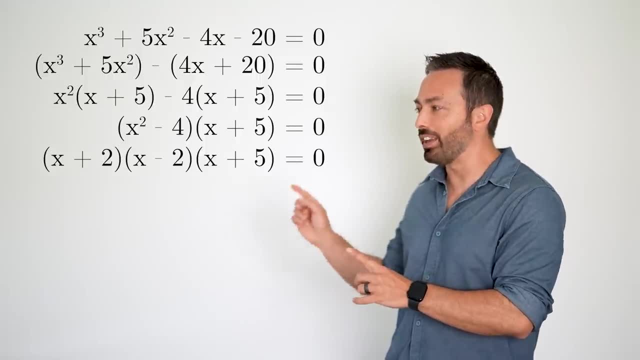 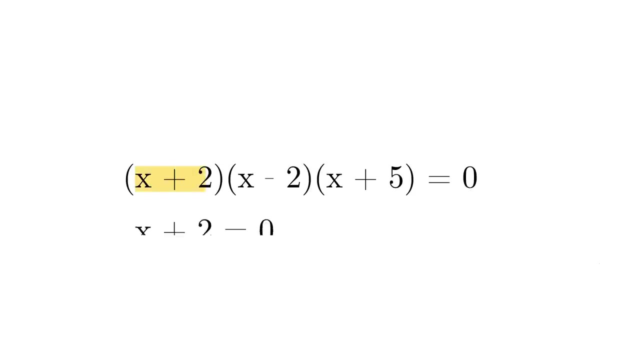 the terms to one side, set them equal to 0, and then factor them. Well, I certainly haven't before making this video, But there is a good reason, And it comes down to the special property of 0. If several terms multiplied together equal 0,, then you know at least one of those terms. 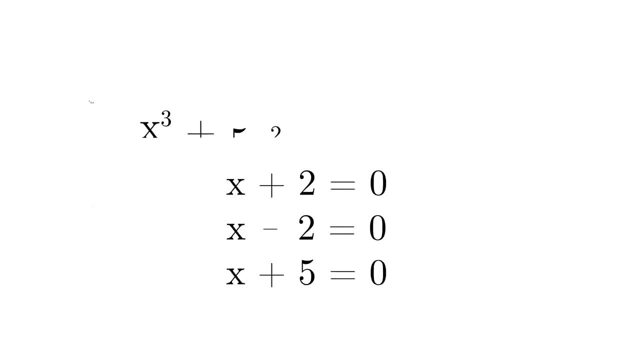 must be 0. And this allows us to break down complicated higher order equations into a set of smaller, simpler equations and solve. But this won't work with the tenadics And fundamentally the reason is because we're working in base 10.. 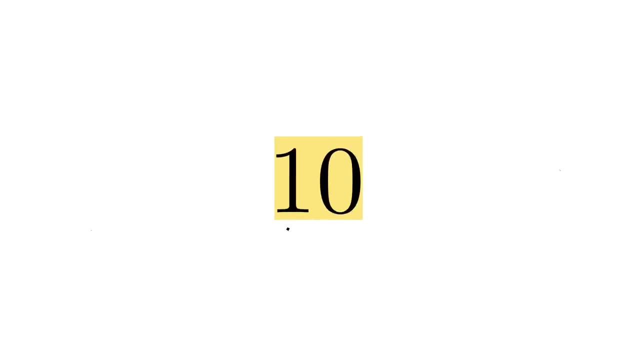 And 10 is a composite number. It's not a prime, It's 5 times 2.. Say you want to find two tenadic numbers that multiply to 0. Then, to start off, you know that the last digit must be 0.. 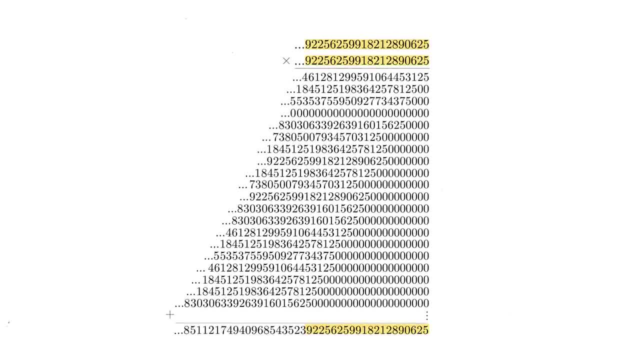 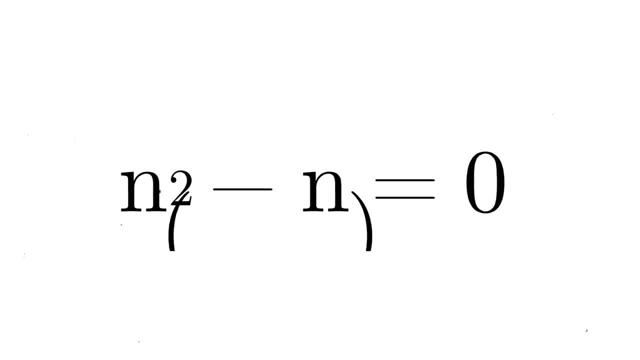 this number by itself, you get back that same number. this number is its own square and that's a problem which you can see. if we move the end to the left hand side and factor it well, then we have n times n minus 1 equals 0, the 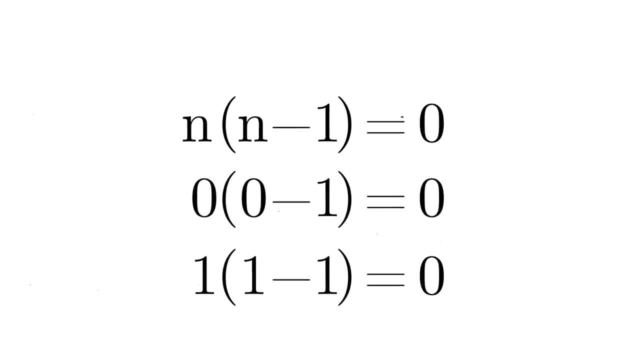 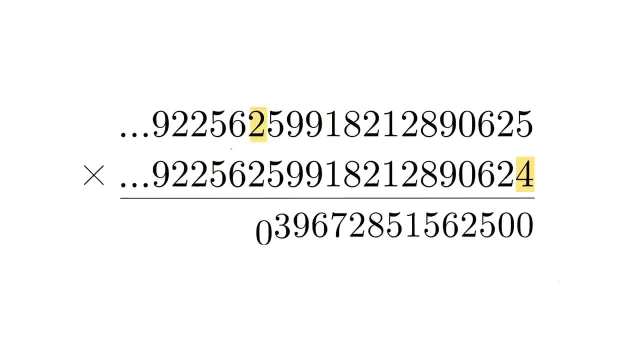 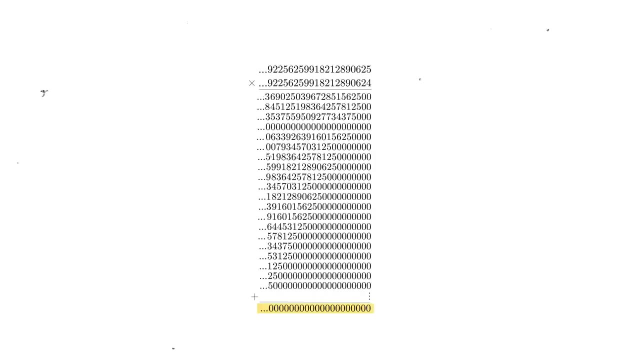 number is 0 or 1 would satisfy this equation, but our ten addict number is not 0 or 1. you can even verify by multiplying it out. this number n times n minus 1 really does work out to 0. this breaks one of the tools mathematicians rely on to solve. 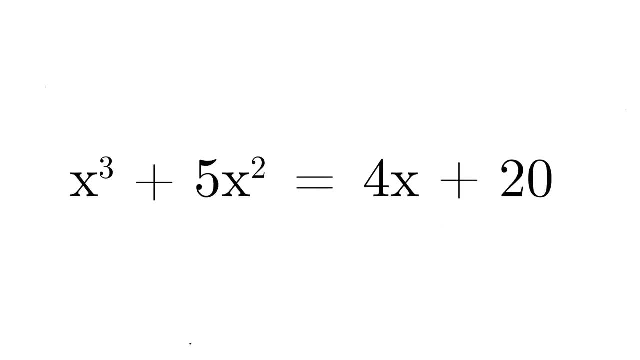 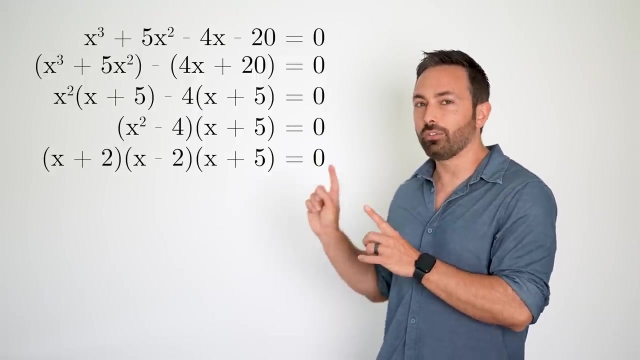 equations. I mean, have you ever thought about why, when faced with some complicated equation, we move all the terms to one side, set them equal to 0 and then factor them? well, I certainly haven't before making this video. but there is a good reason, and it comes down to the special property of 0 if several 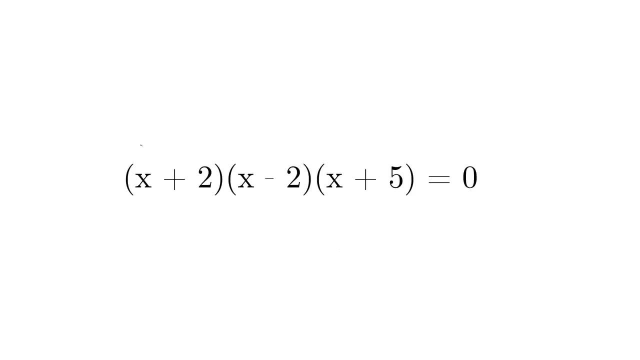 terms multiplied together equals 0, then you know, at least one of those terms must be 0 and this allows us to break down complicated, higher-order equations into a set of smaller, simpler equations and solve. but this won't work with the 10 addicts and fundamentally the reason is because we're working in base 10 and 10 is a. 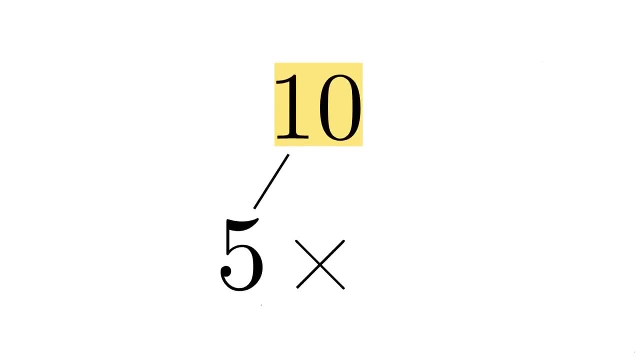 composite number. it's not a prime, it's 5 times 2. say you want to find two ten addict numbers that multiply to 0. then to start off, you know that the last digit must be 0. so which two numbers could you multiply it to get a? 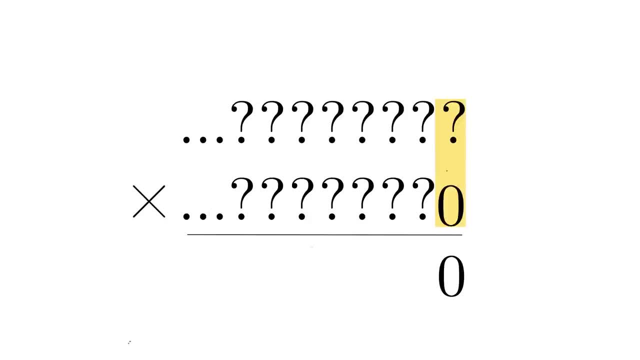 zero in the units place. well, you could multiply 0 times any number, that's no problem. but you could also multiply, say, 5 times 4 and get 20, which gives you a zero in the units place. then you can carry the 2 and find another two numbers. 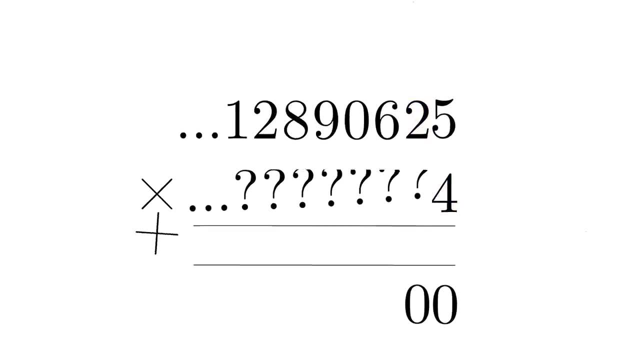 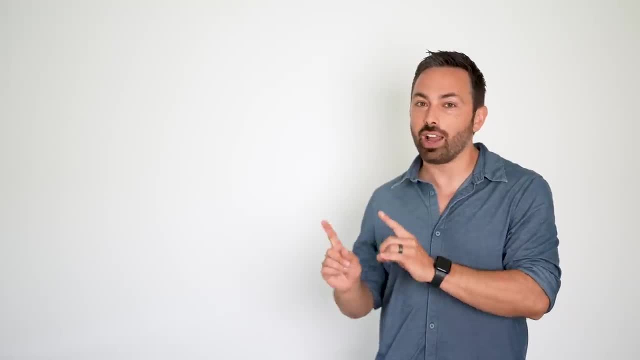 that will give you a zero in the tens place and you can keep building the numbers from there so that all the digits work out to 0. there is a way to avoid this, and that is to use a prime number base instead of base 10. it could. 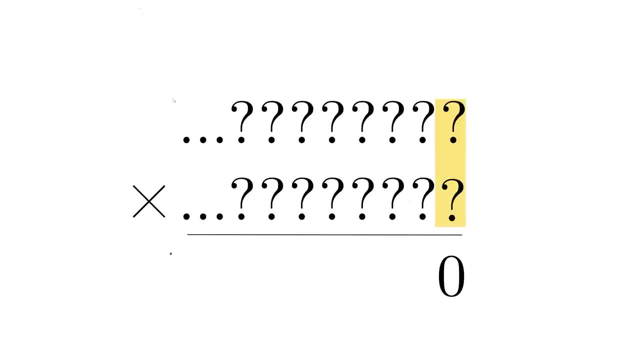 So which two numbers could you multiply to get a 0 in the units place? Well, you could multiply 0 times any number, that's no problem. But you could also multiply, say, 5 times 4, and get 20, which gives you a 0 in the units. 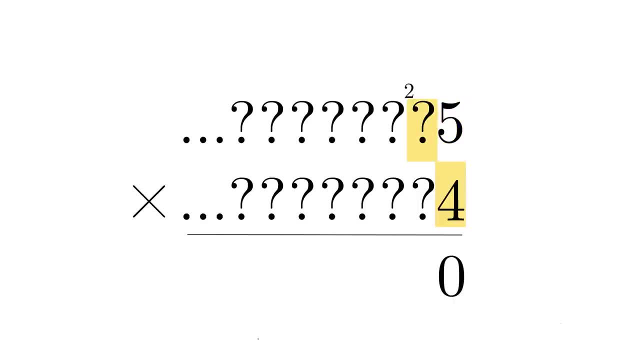 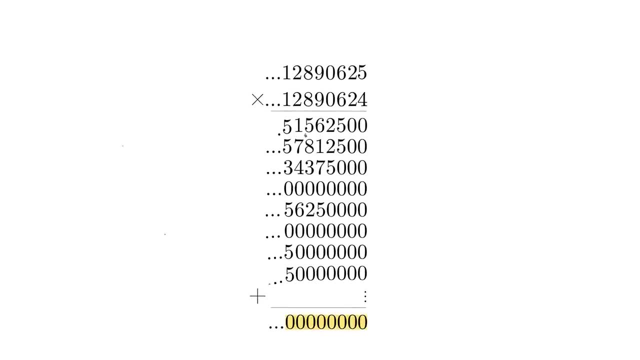 place. Then you can carry the 2 and find another two numbers. that will give you a 0 in the tens place And you can keep building the numbers from there so that all the digits work out to 0. There is a way to avoid this. 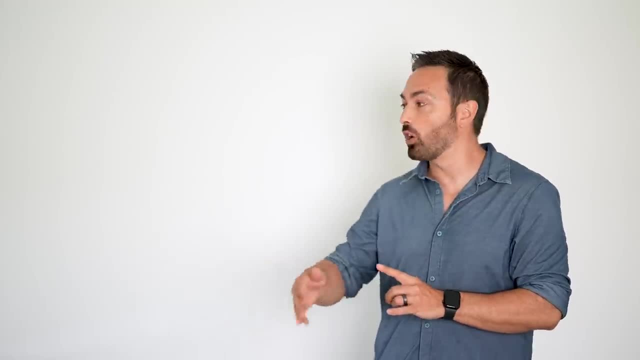 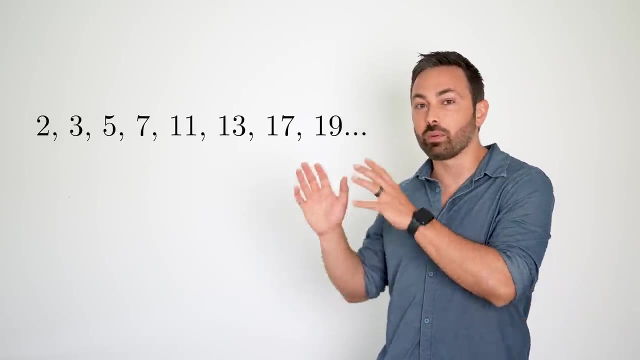 And that is to use a prime number base instead of base 10.. It could be any prime like 2,, 3,, 5,, 7, etc. As an example, let's create a threeadic number. So this is a base 3 number with infinite digits to the left of the decimal point. 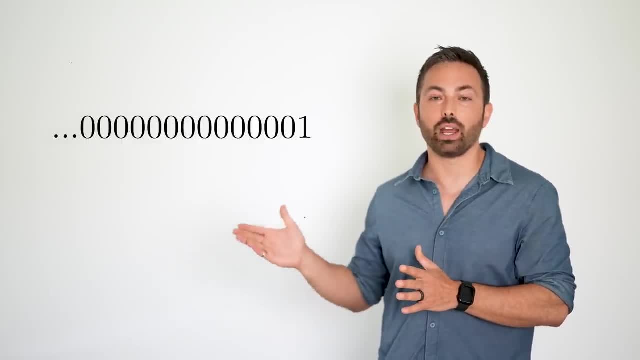 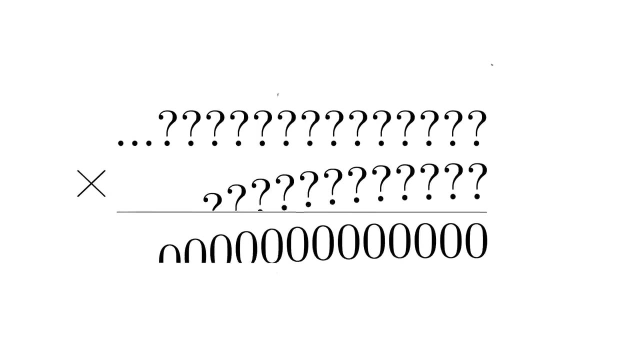 In the threeadics, the only digits we can use are 0,, 1, and 2. Because 3 is the same thing as 1, 0. Now how could you multiply two threeadic numbers to get 0?? 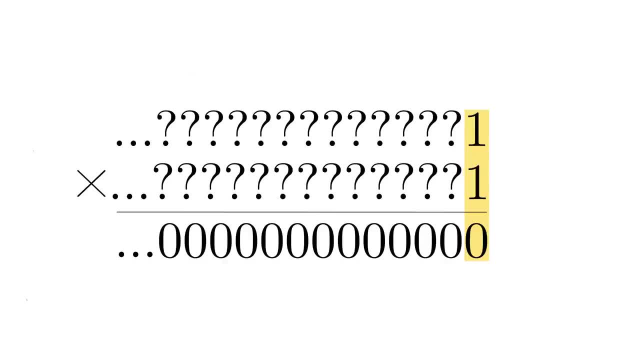 Well, again we can start by just looking at the last digit: 1 times 1 is 1.. 2 times 1 is 2.. And 2 times 2 is 4, which in base 3 is 1, 1.. 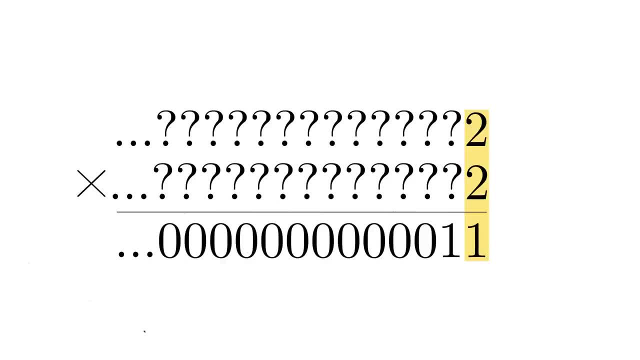 So the only way to get a 0 is if one of those threeadic digits itself is 0. And it's the same for all the digits going to the left. The only way they multiply to 0 is if one of the threeadic numbers is itself entirely. 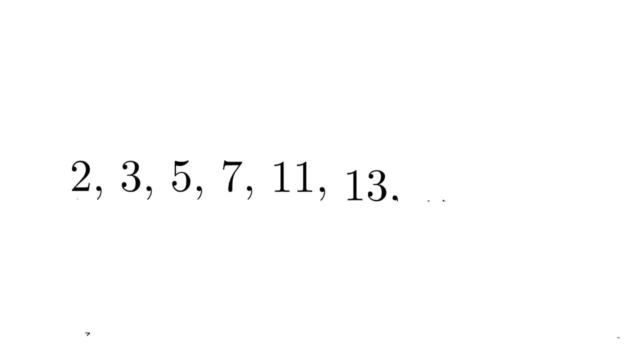 0.. And this works for any prime base and restores the useful property that the product of several numbers will only be 0 if one of those numbers is itself 0.. Here is a random threeadic number. This number means 1 times 3 to the 0,, plus 2 times 3, plus 1 times 3 squared plus 1. 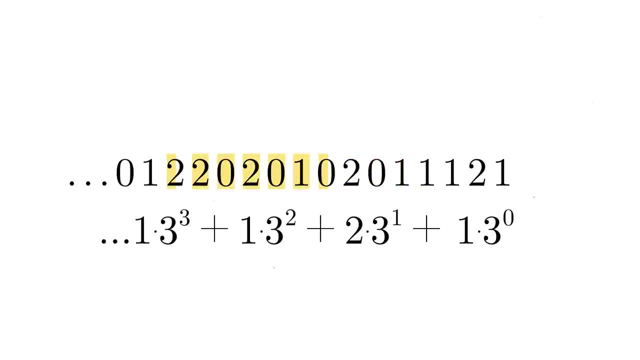 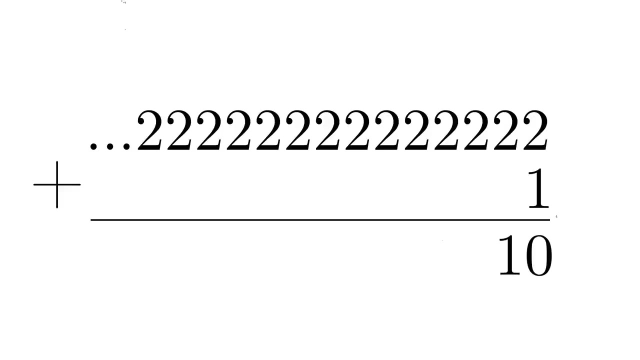 times 3 cubed and so on. So you can think of a threeadic number as an infinite expansion in powers of 3.. The threeadic integer that equals negative 1 would be an infinite string of 2s. If you add 1, then 2 plus 1 is 3, which in base 3 is 1, 0. 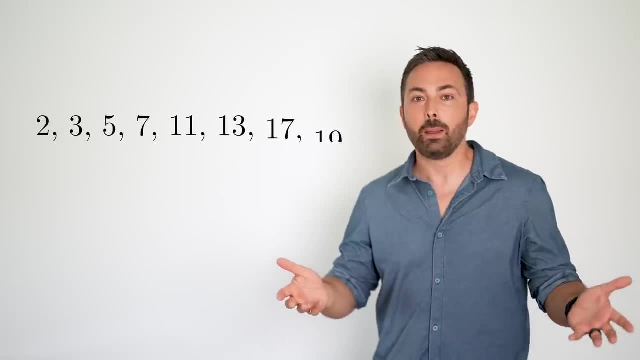 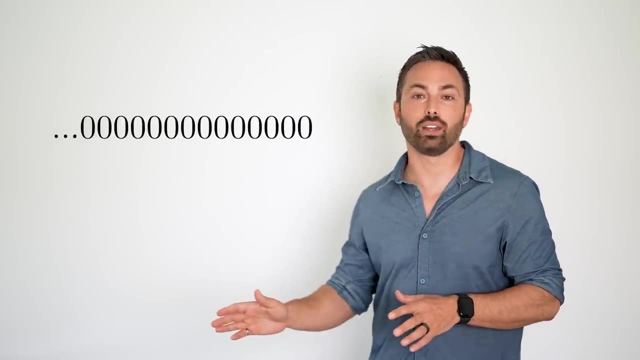 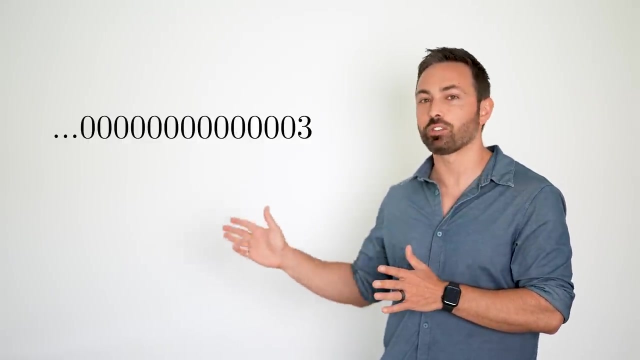 be any prime like 2, 3, 5, 7, etc. as an example, let's create a three addict number. so this is a base three number with infinite digits to the left of the decimal point in the three addicts. the only digits we can use are 0, 1 & 2, because 3 is the same thing as 1- 0. 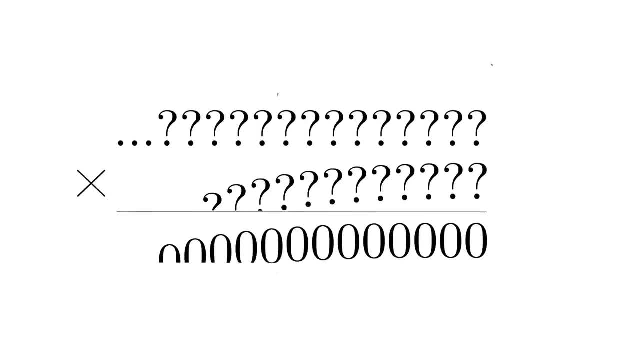 now, how could you multiply two, three addict numbers to get 0? well, again, we can start by just looking at the last digit: 1 times 1 is 1, 2 times 1 is 2 and 2 times 2 is 4, which in base 3 is 1- 1. so the only way to get a 0 is if one of those three. 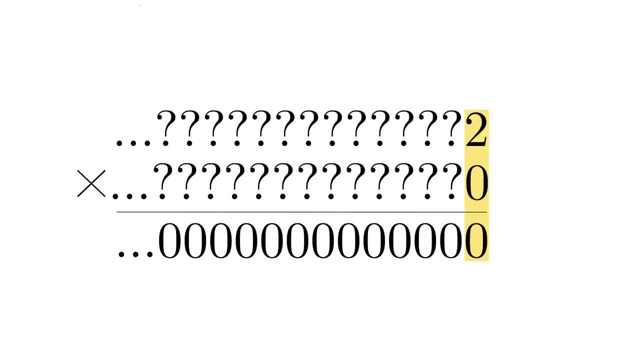 addict digits itself is 0, and it's the same for all the digits going to the left. the only way they multiply to 0 is if one of the three addict numbers is itself entirely 0, and this works for any prime base and restores the useful. 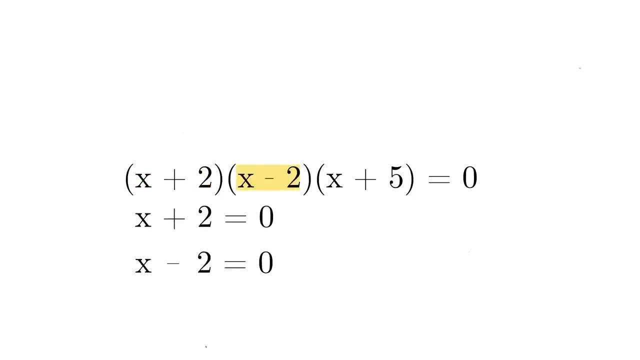 property that the product of several numbers will only be 0 if one of those numbers is itself 0. here is a random three addict number. this number means 1 times 3 to the 0 plus 2 times 3 plus 1 times 3 squared, plus 1 times 3 cubed, and so on. so you: 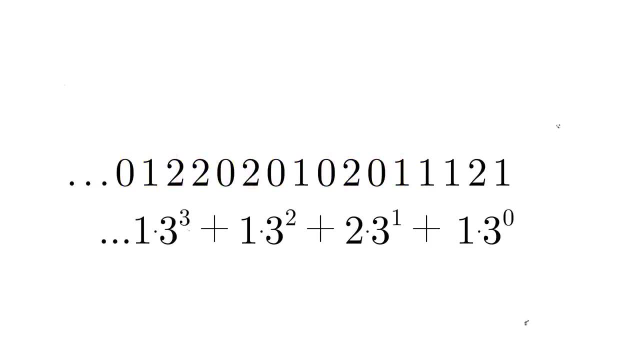 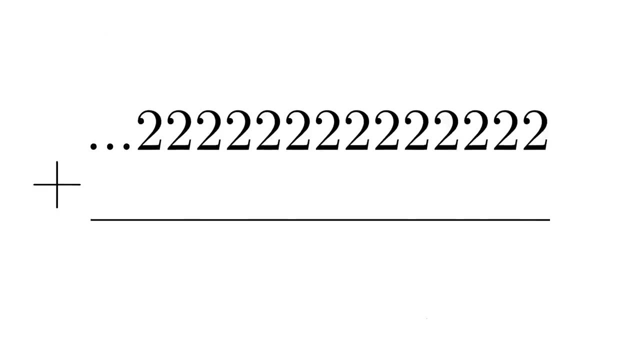 can think of a three addict number as an infinite expansion in powers of 3, the three addict integer that equals negative 1 would be an infinite string of twos. if you add 1, then 2 plus 1 is 3, which in base 3 is 1: 0. so you leave the 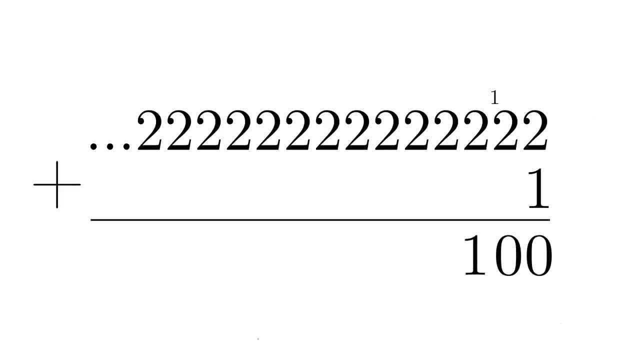 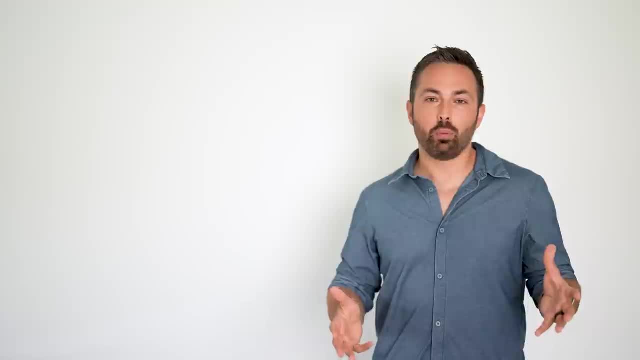 0 carry the 1, and 2 plus 1 is again 1: 0. so you carry the 1 and you keep going on like that forever. P addicts have all the same properties as the 10 addicts, but in addition, you will never find a number that is its own square besides 0 and 1, nor will you find 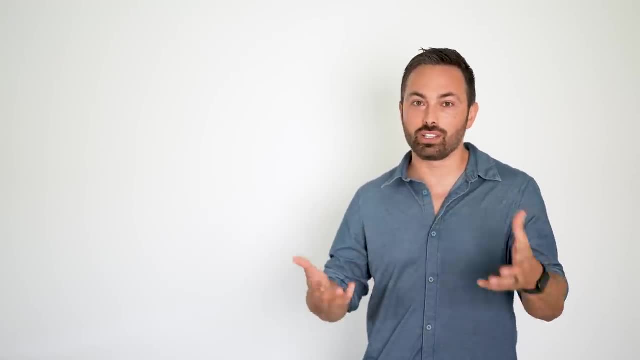 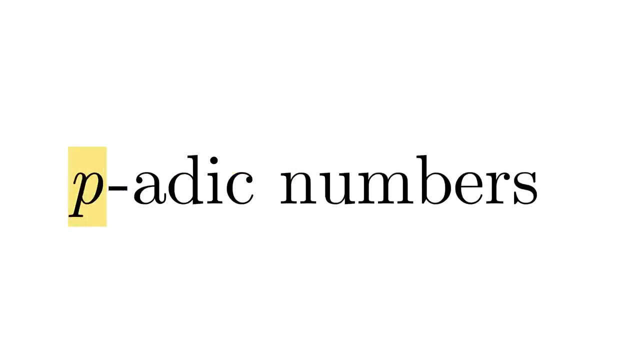 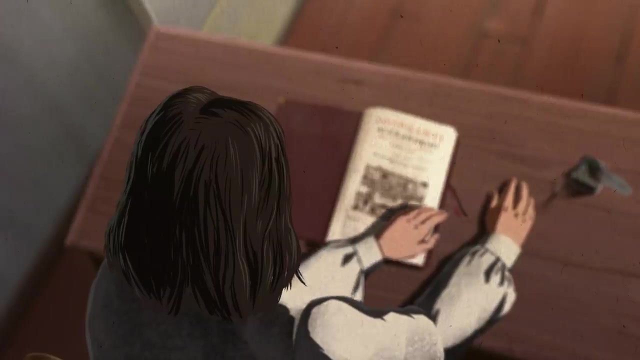 one nonzero number times another nonzero number being equal to 0, and this is why professional mathematicians work with P addicts, where the P stands for prime rather than say the 10 addicts. P addicts are the real tool. they have been used in the work of over a dozen recent Fields medalists. they were 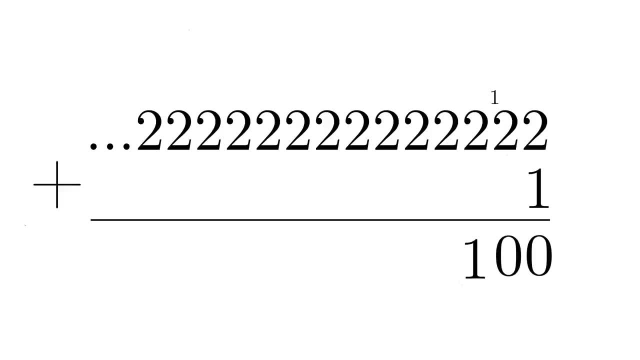 So you leave the 0,, carry the 1,, and 2 plus 1 is again 1, 0. So you carry the 1, and you keep going on like that forever. P-addicts have all the same properties as the 10-addicts. 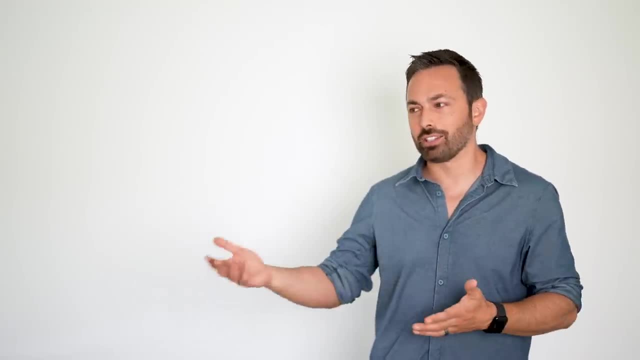 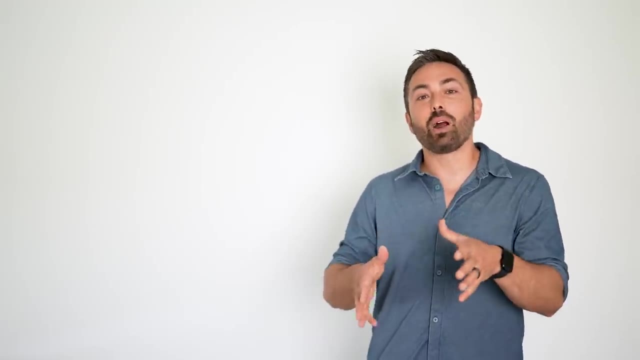 But, in addition, you will never find a number that is its own square besides 0 and 1.. Nor will you find one non-zero number times another non-zero number being equal to 0.. And this is why professional mathematicians work with p-addicts. 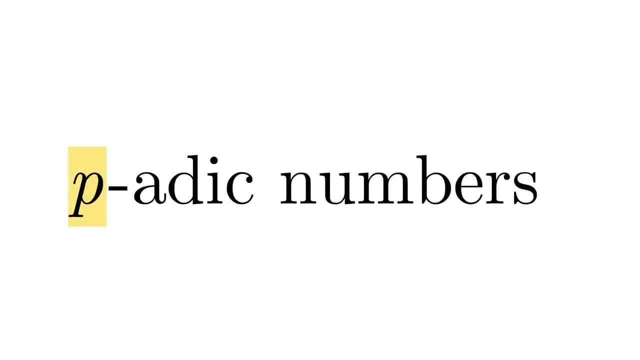 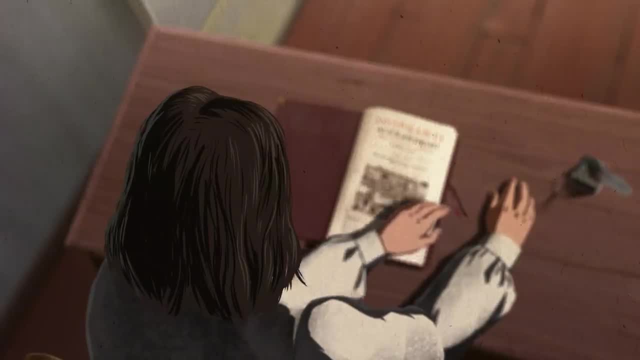 Where the p stands for prime, rather than say the 10-addicts. P-addicts are the real tool. They have been used in the work of over a dozen recent Fields Medalists. They were even involved in cracking one of the most legendary math problems of all time. 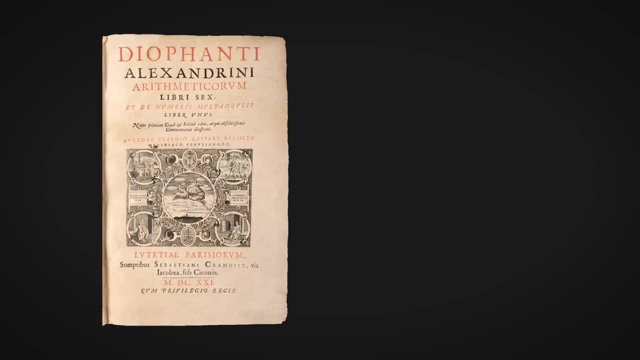 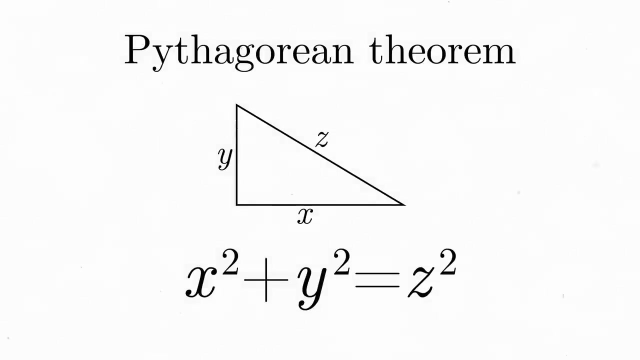 In 1637, Pierre de Fermat was reading the book Arithmetica by the ancient Greek mathematician Diophantus. Diophantus was interested in the solutions to polynomial equations phrased in geometric terms. For a right triangle, x squared plus y squared equals z squared. 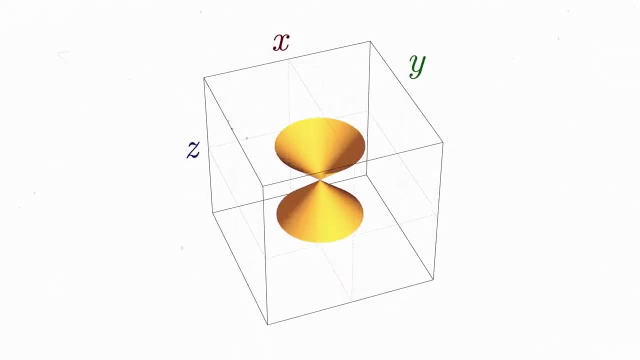 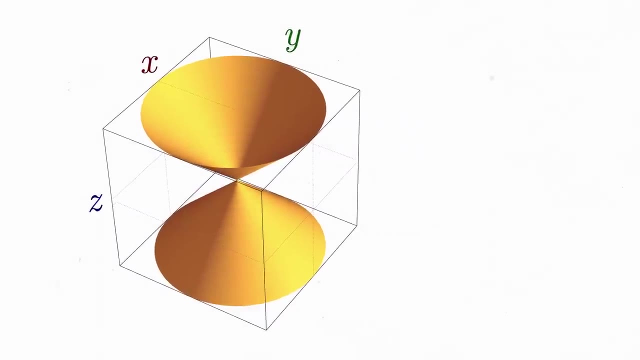 The set of solutions to this equation in the real numbers is pretty easy to find- It's just an infinite cone. But Diophantus wanted to find solutions that were whole numbers or fractions Like 3,, 4, 5, and 5,, 12, 13.. 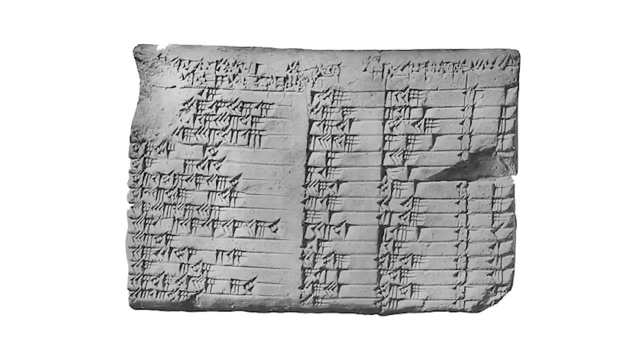 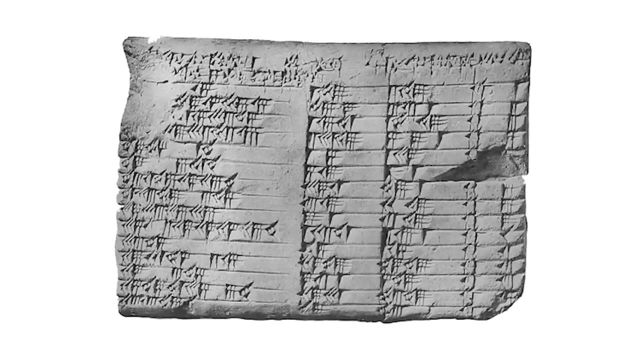 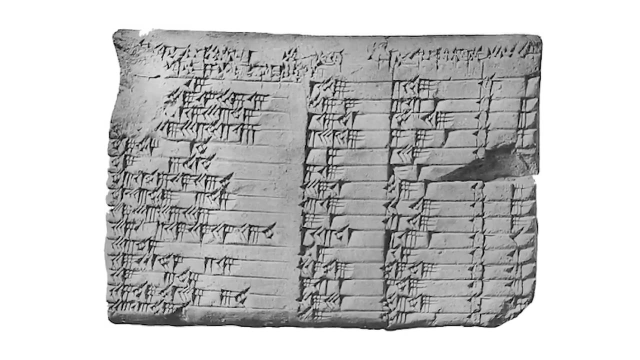 And he wasn't the first. Here is an ancient Babylonian clay tablet from about 2000 BC with a huge list of these examples. By the way, this list predates Pythagoras by more than a millennium. Right next to Diophantus' discussion of the Pythagorean Theorem, Fermat writes a statement. 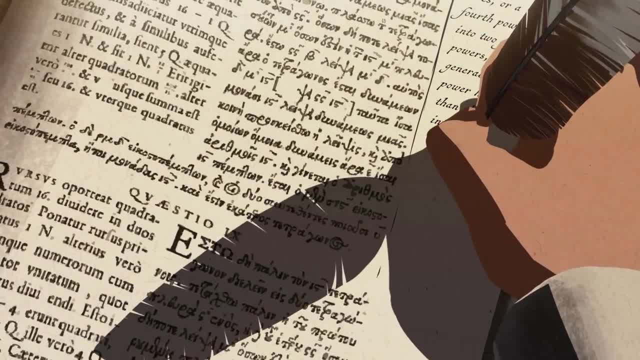 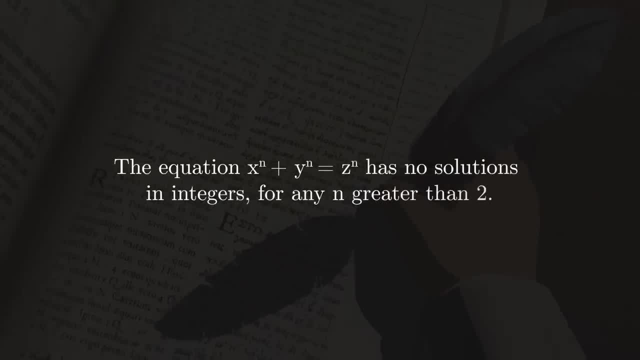 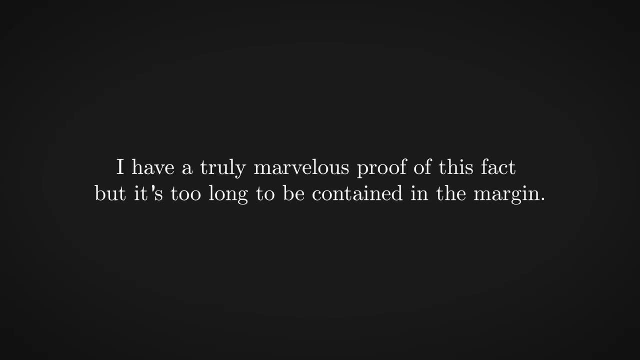 that will go down in history as one of the most infamous of all time. The equation x to the n plus y to the n equals z to the n has no solutions in integers for any n greater than 2.. I have a truly marvelous proof of this fact, but it's too long to be contained in the margin. 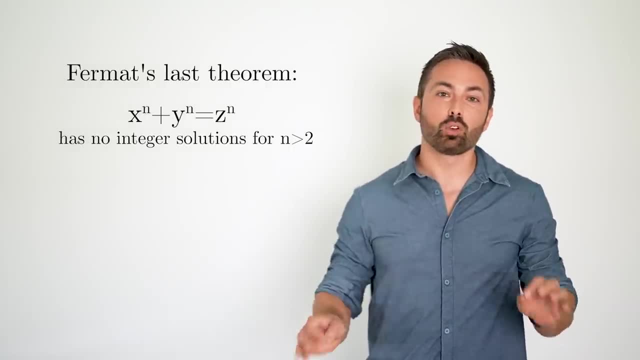 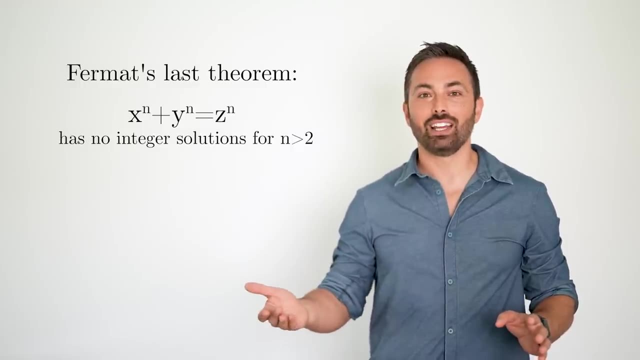 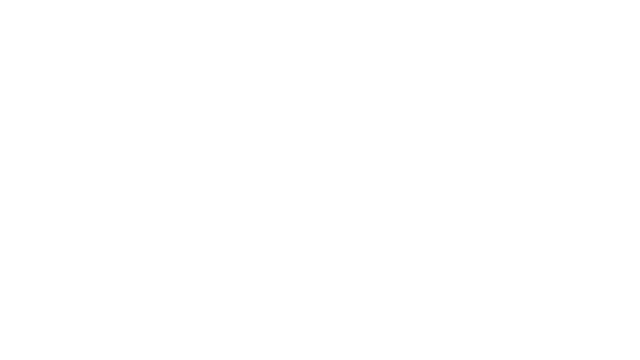 Fermat's Last Theorem. The theorem, as this became known, would go unproven for 358 years. In fact, to solve it, new numbers had to be invented, the Piatics, And these provide a systematic method for solving other problems in Diophantus' Arithmetica. 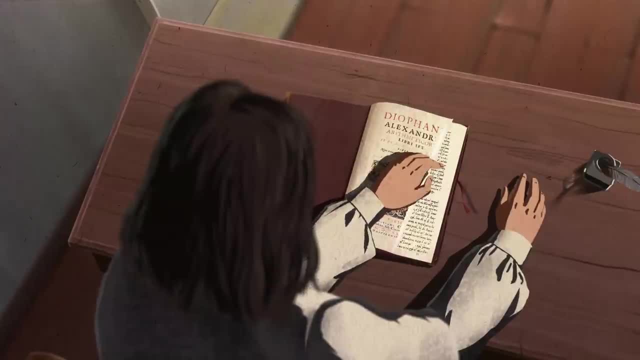 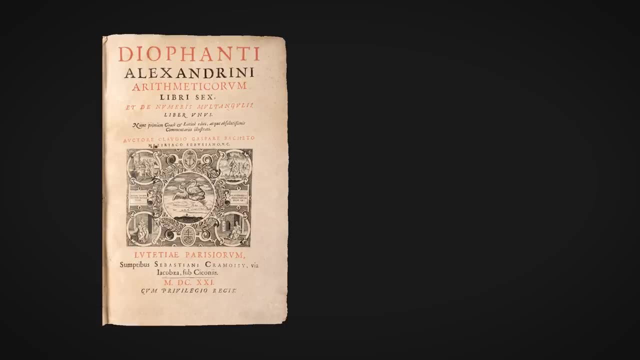 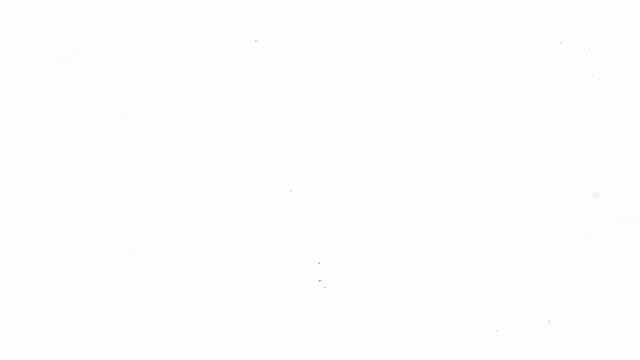 even involved in cracking one of the most legendary math problems of all time. in 1637, Pierre de Fermat was reading the book Arithmetica by the ancient Greek mathematician Diophantus. Diophantus was interested in the solutions to polynomial equations phrased in geometric terms, like the Pythagorean. 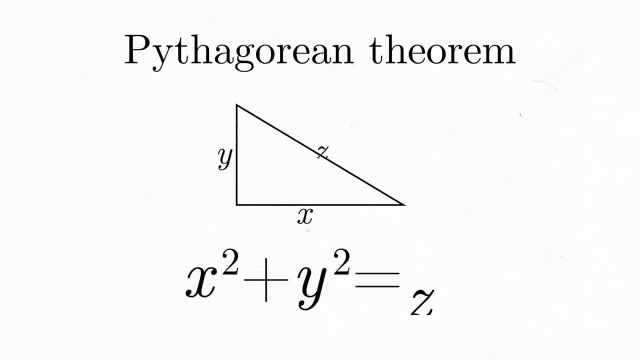 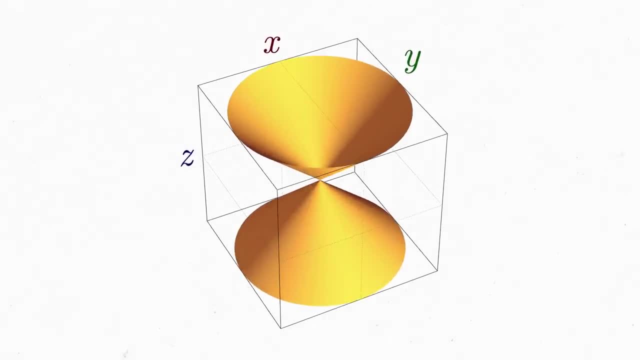 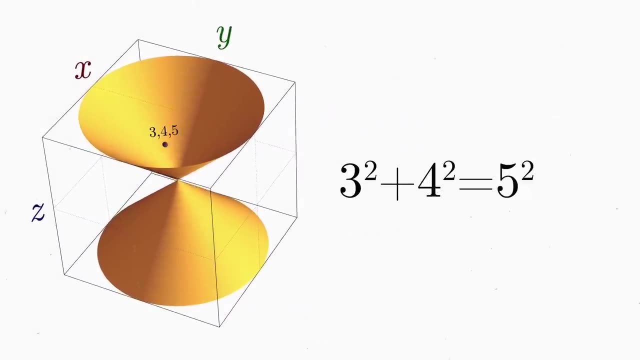 theorem: for a right triangle, x squared plus y squared equals z squared. the set of equations to this equation in the real numbers is pretty easy to find. it's just an infinite cone. but Diophantus wanted to find solutions that were whole numbers or fractions like 3, 4, 5 and 5, 12, 13.. and he wasn't the first. here is an. 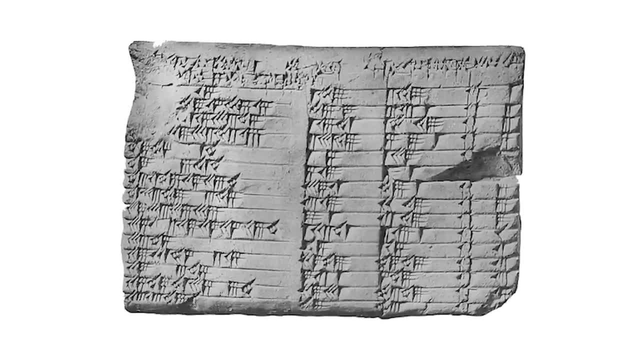 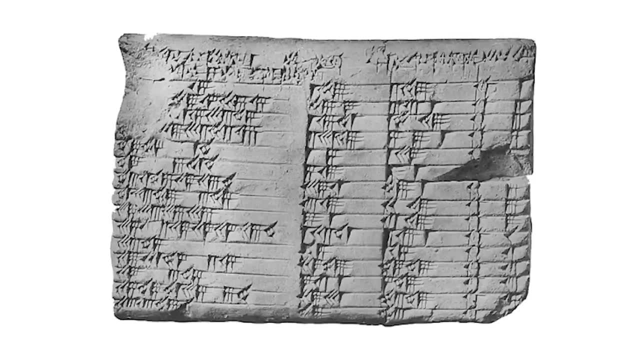 ancient Babylonian clay tablet from about 2000 BC with a huge list of these Pythagorean triples. by the way, this list predates Pythagoras by more than a millennium. right next to Diophantus's discussion of the Pythagorean theorem, Fermat writes a statement that will: 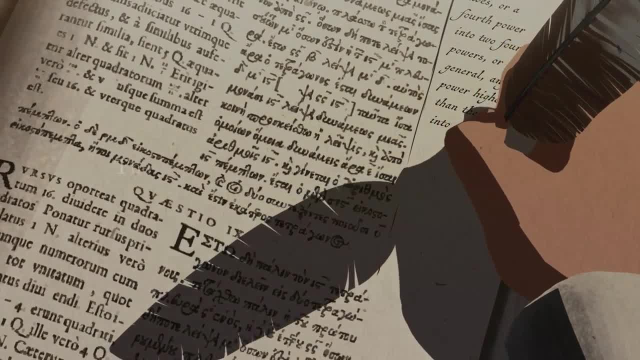 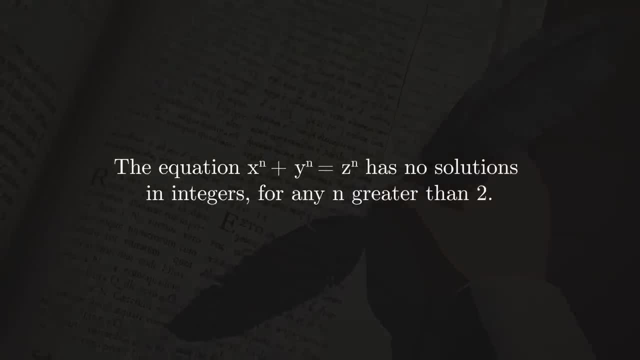 go down in history as one of the most infamous of all time. the equation x to the n plus y to the n equals z to the n. has no solutions in integers for any n greater than two. I have a truly marvelous proof of this fact, but it's too long to be contained in the margin. 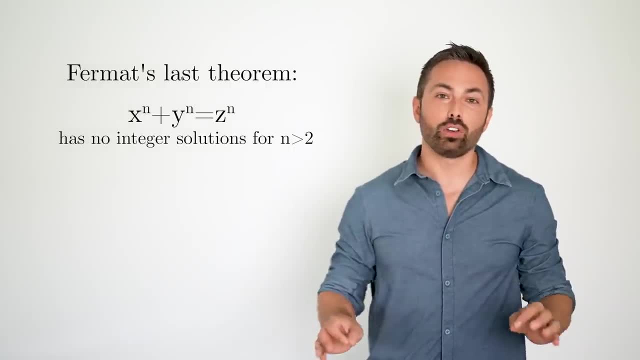 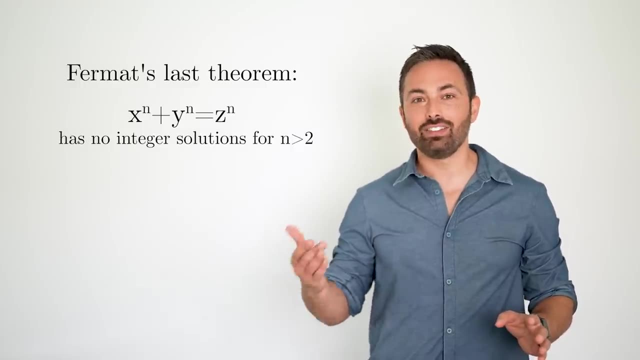 Fermat's last theorem, as this became known, would go unproven for 358 years. in fact, to solve it, New numbers had to be invented, the piatics, and these provide a systematic method for solving other problems in Diophantus's Arithmetica. 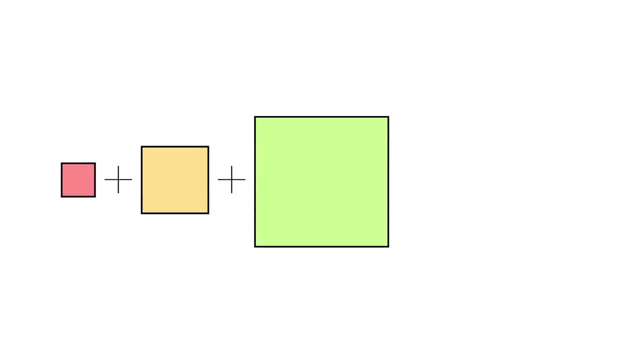 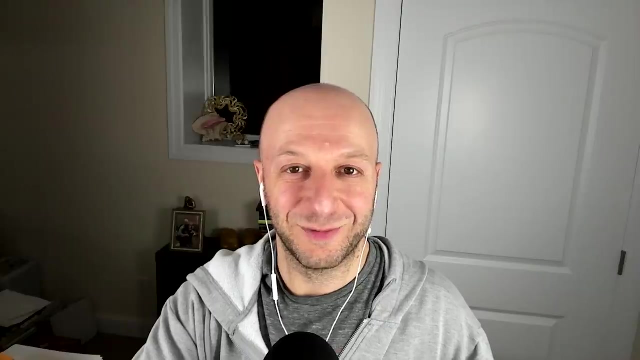 for example, find three squares whose areas add to create a bigger square, and the area of the first square is the side length of the second square and the area of the second square is the side length of the third square. he's really giving the the first instance of Algebra many 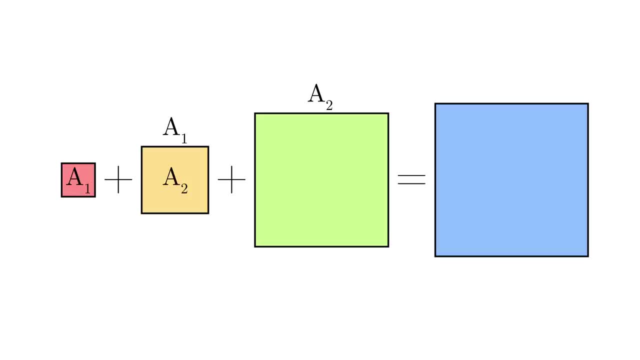 many centuries before, uh, algebra. So if we set the side of the first square to be x, then its area is x squared. This is the side length of the second square, which therefore has an area of x to the 4.. This is then the side length of the third square, which has an area of x to the 8.. 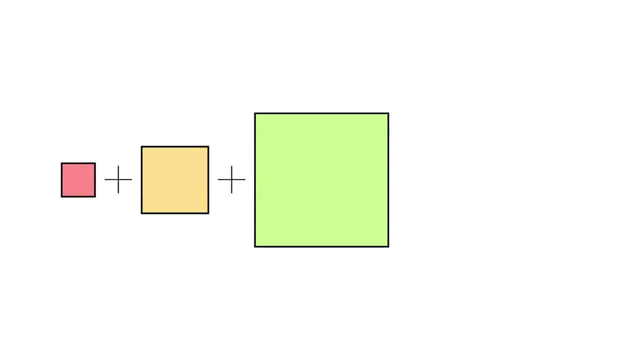 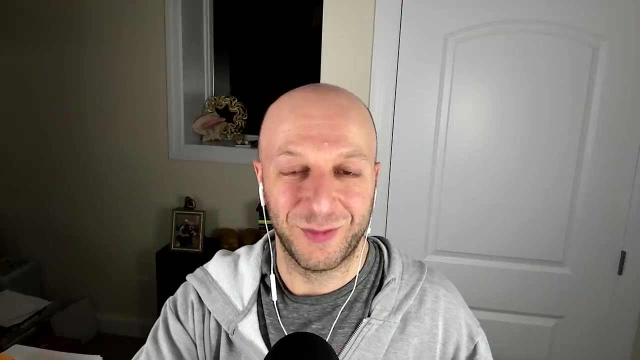 For example, find three squares whose areas add to create a bigger square, And the area of the first square is the side length of the second square And the area of the second square is the side length of the third square. He's really giving the first instance of algebra many, many centuries before algebra. 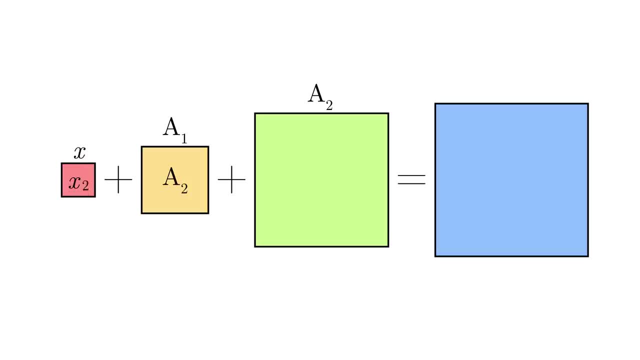 So if we set the side of the first square to be x, then its area is x squared. This is the side length of the second square, which therefore has an area of x to the 4.. This is then the side length of the third square, which has an area of x to the 8.. 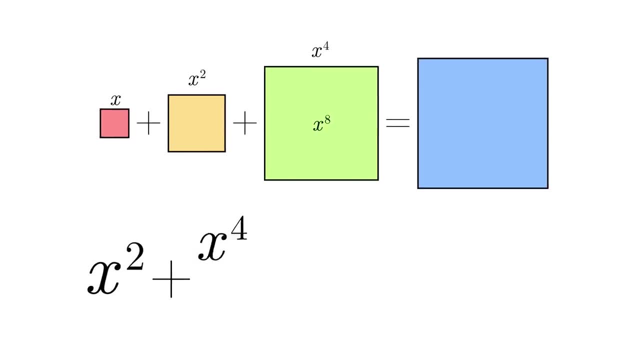 And we want these three areas- x squared plus x to the 4 plus x to the 8, to add, to make a new square. So let's call its area 1. Y squared. So x squared plus x to the 4 plus x to the 8 equals y squared. 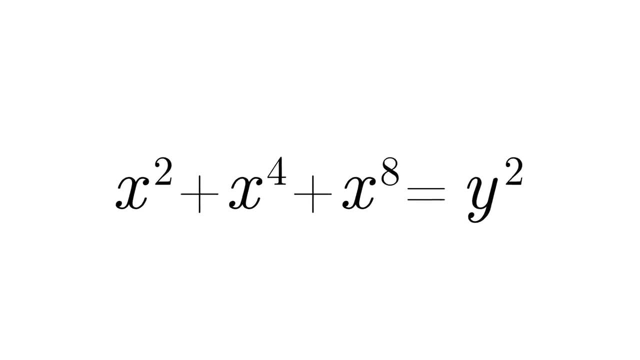 Now it's not hard to find solutions to this equation in the real numbers. For example, set x equal to 1, and you find y is root 3.. In fact, we can make a plot of all the real number solutions to this equation. 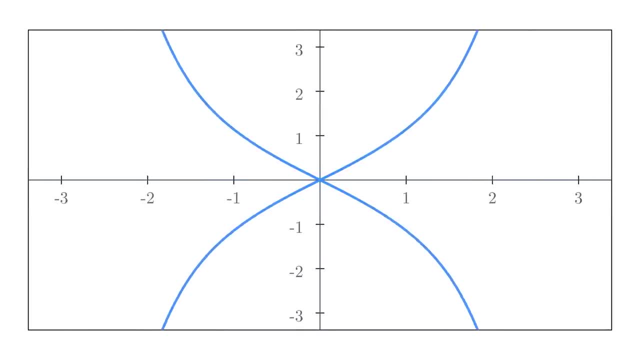 But Diophantus wasn't interested in real solutions. he wanted rational solutions, Solutions that are whole numbers or fractions. These are much harder to find. Where would you even start? And we're totally stuck, Like: what do you do? 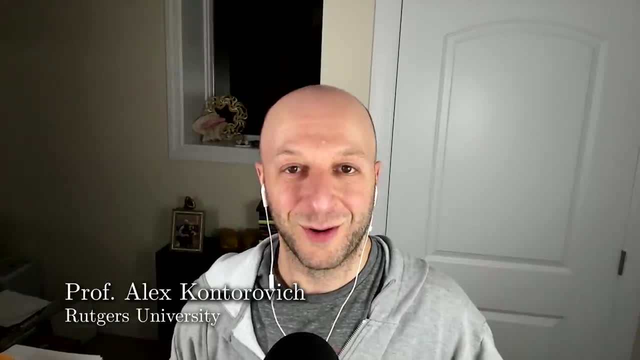 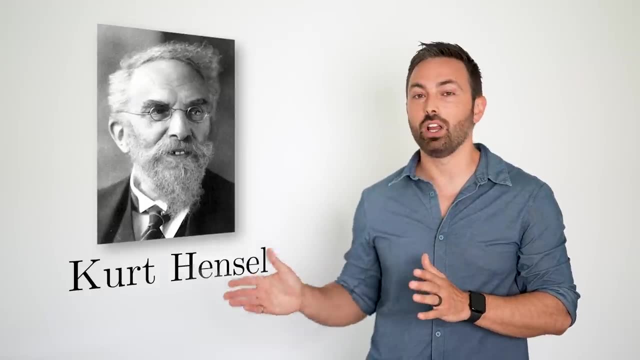 You know you have this cliff and you're looking for anywhere to grab a hold of, And there's nothing in sight. Well, in the late 1800s, a mathematician named Kurt Hensel tried to find solutions to equations. 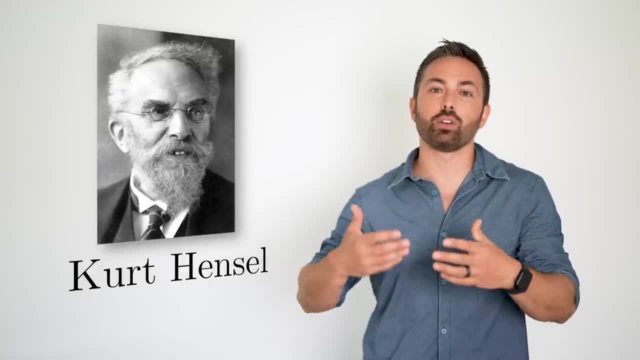 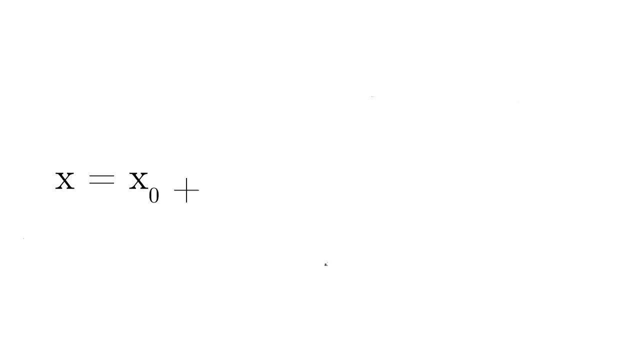 like this one in the form of an expansion of increasing powers of primes. So, working with the prime 3, the solutions would take the form of x equals x naught, plus x1 times 3.. Plus x2 times 3 squared, plus x3 times 3 cubed, and so on. 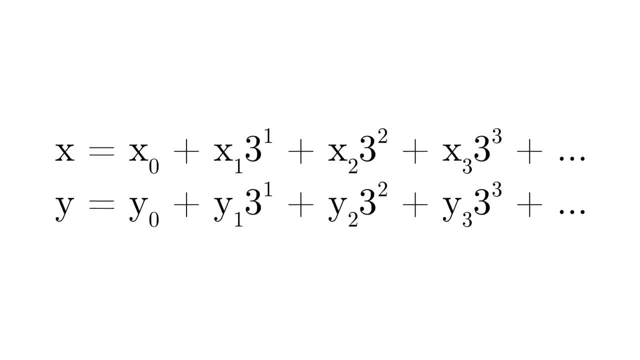 And y would also be a similar expansion in powers of 3.. Each of the coefficients would be either 0,, 1, or 2.. Now imagine inserting these expressions into our equation for x and y And you can see it's going to get messy real fast. 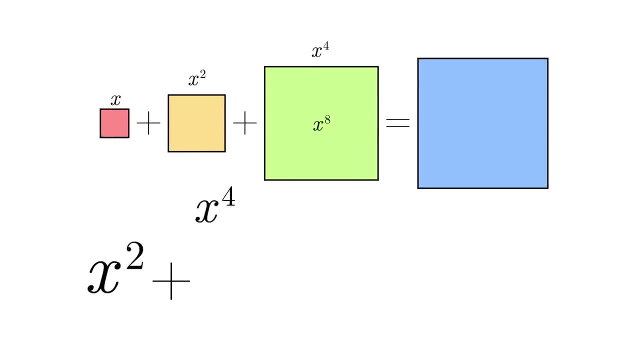 And we want these three areas- x squared plus x to the 4 plus x to the 8, to add, to make a new square. So let's call its area y squared. So x squared plus x to the 4 plus x to the 8 equals y squared. 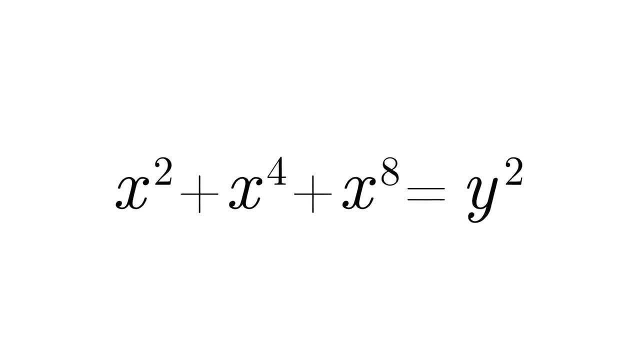 Now it's not hard to find solutions to this equation in the real numbers. For example, set x equal to 1, and you find y is root 3.. In fact, we can make a plot of all the real number solutions to this equation. 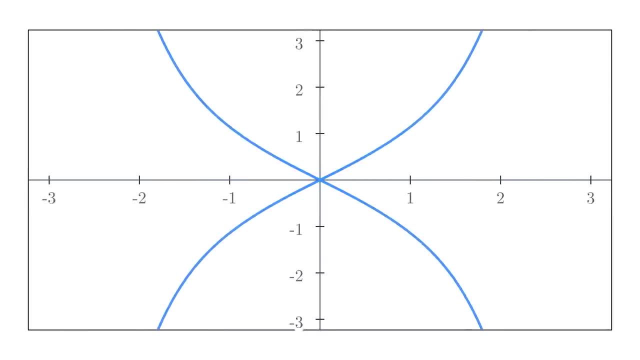 But Diophantus wasn't interested in real solutions. He wanted rational solutions, solutions that are whole numbers or fractions. These are much harder to find. I mean, where would you even start? And we're totally stuck, Like: what do you do? 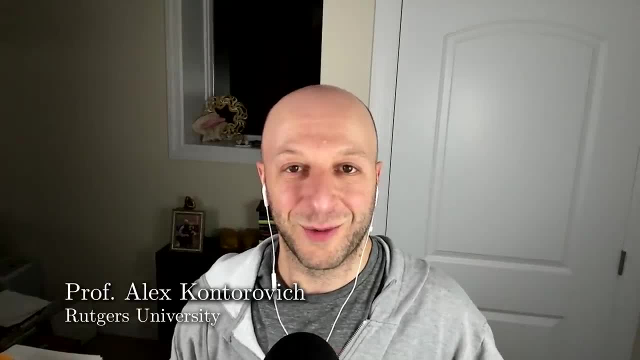 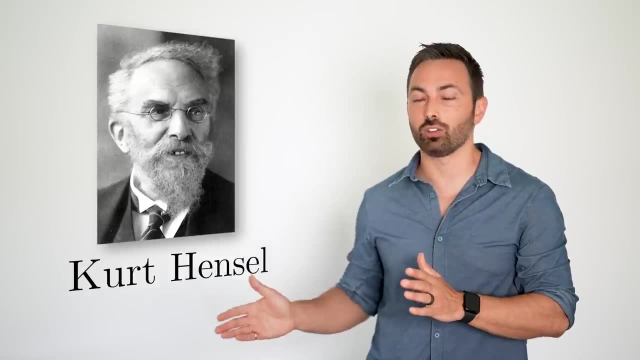 You know you have this cliff And you're looking for anywhere to grab a hold of, And there's nothing in sight. Well, in the late 1800s, a mathematician named Kurt Hensel tried to find solutions to equations like this one. 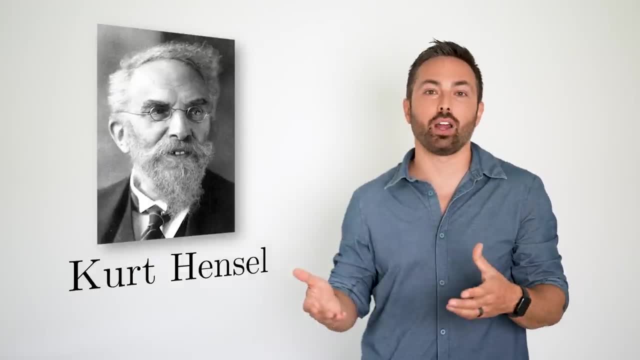 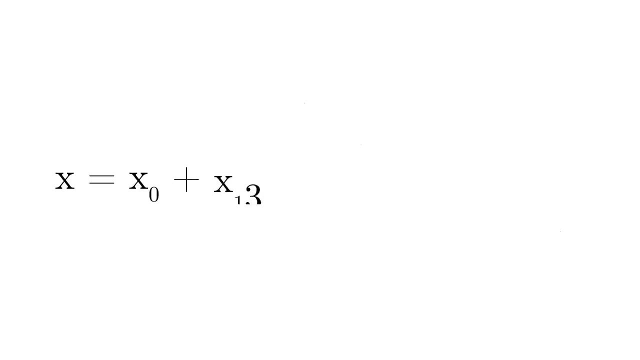 in the form of an expansion of increasing powers of primes. So, working with the prime 3, the solutions would take the form of x equals x naught, plus x1 times 3, plus x2 times 3 squared, plus x3 times 3 cubed, and so on. 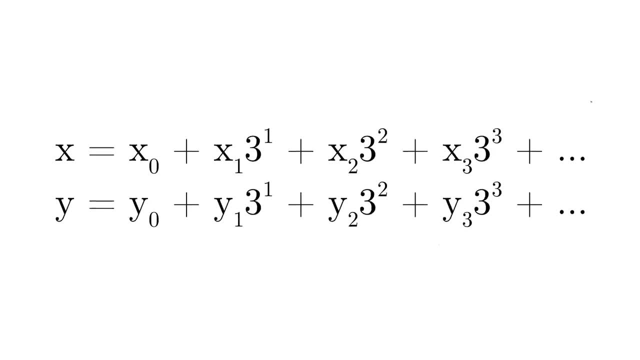 And y would also be a similar expansion in powers of 3.. Each of the coefficients would be either 0,, 1 or 2.. Now imagine inserting these expressions into our equation for x and y And you can see it's going to get messy real fast. 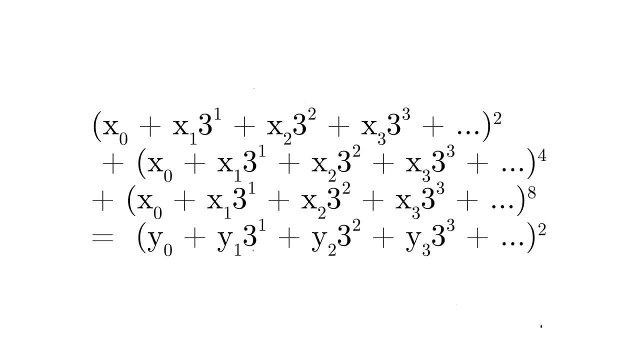 But there is a way to simplify things. Say, you wanted to write 17 in base 3.. Well, one way to do it is to divide 17 by 3 and find the remainder, which in this case is 2.. 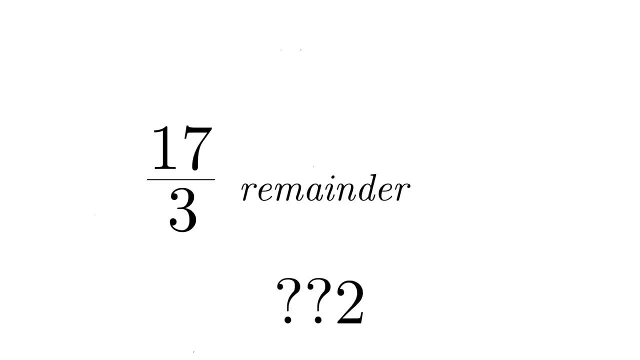 So we know the units digit of our base 3 number is 2.. Next divide 17 by 9,, the next higher power of 3, and you get a remainder of 8.. Subtract off the 2 we found before and you have 6,, which is 2 times 3.. So we know the second to last. 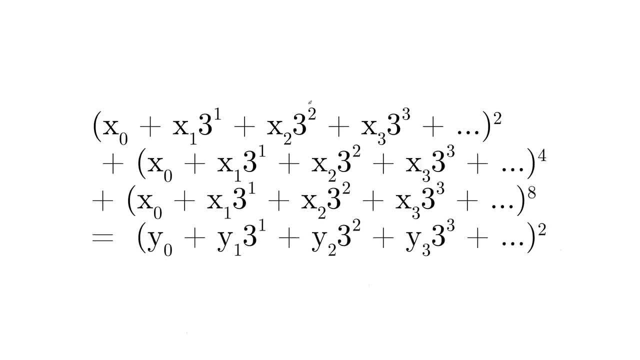 But there is a way to simplify things. Say you wanted to write 17 in base 3.. You could write 17 in base 2.. You could write 17 in base 3.. You could write 17 in base 3.. 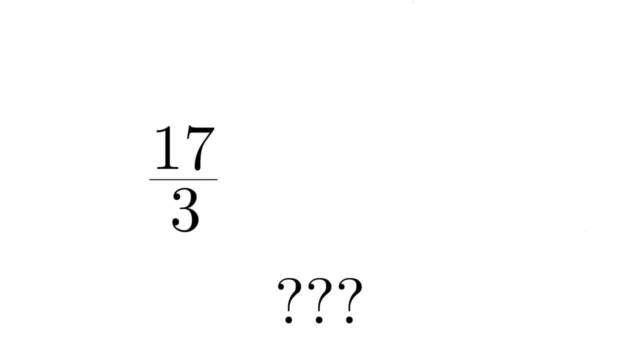 Well, one way to do it is to divide 17 by 3 and find the remainder, which in this case is 2.. So we know, the units digit of our base 3 number is 2.. Next, divide 17 by 9,, the next higher power of 3, and you get a remainder of 8.. 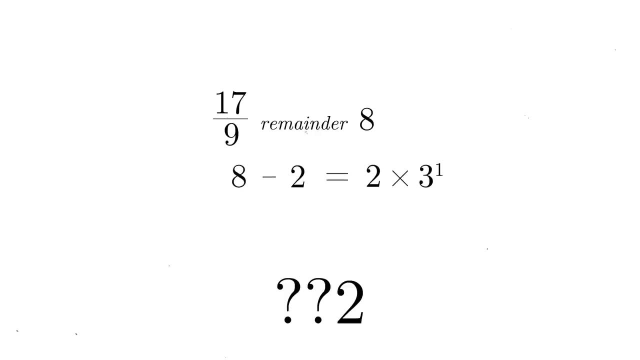 Subtract off the 2 we found before and you have 6,, which is 2 times 3.. So we know the second to last digit is 2.. Next, divide 17 by 27, and you get a remainder of 17.. 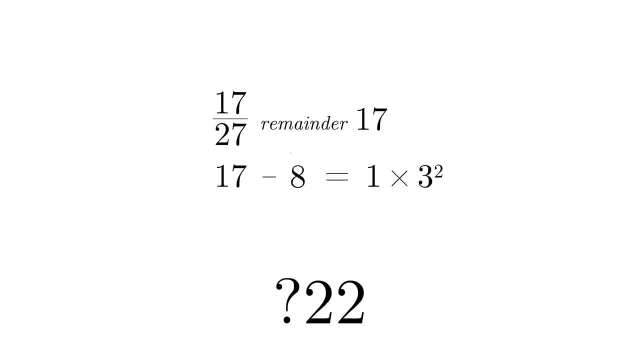 Subtract off the 8 we've already accounted for and you have 9, so the 9th digit is 1.. So 17 in base 3 is 1, 2, 2.. What we're doing here is a form of modular arithmetic. 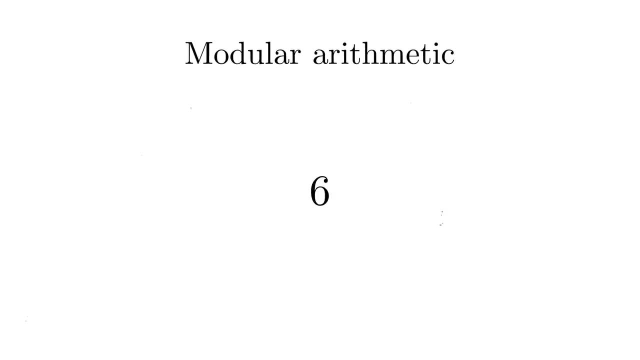 In modular arithmetic numbers reset back to 0 once they reach a certain value called the modulus. The hours on a clock work kind of like this: with a modulus of 12. The hours increase up to 11, but then 12 o'clock is the same thing as 0 o'clock. 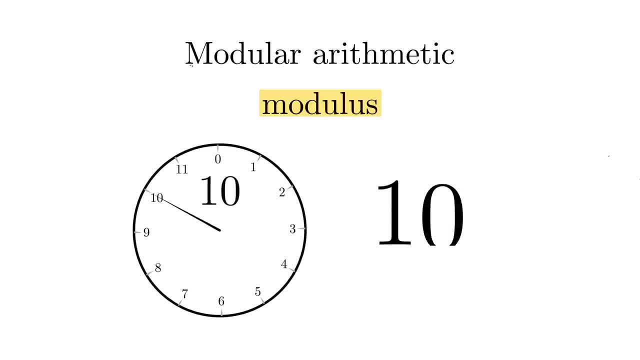 If it's 10 in the morning, say what time will it be in 4 hours You could say 14,, but usually we'd say 2pm, because 2 is 14 modulo 12.. It's 2 more than a multiple of 12.. 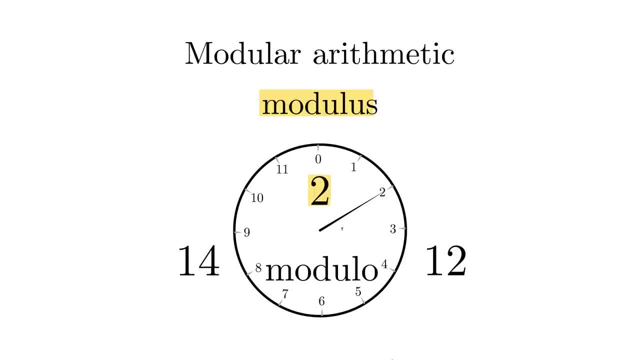 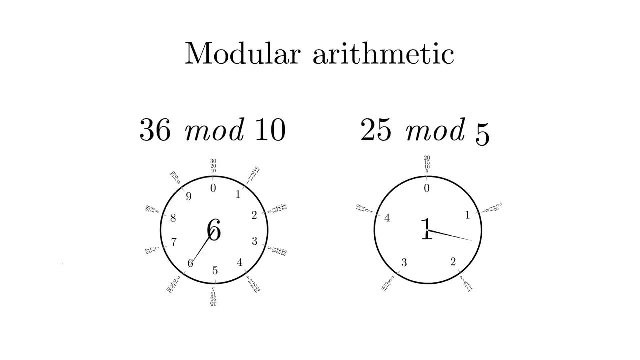 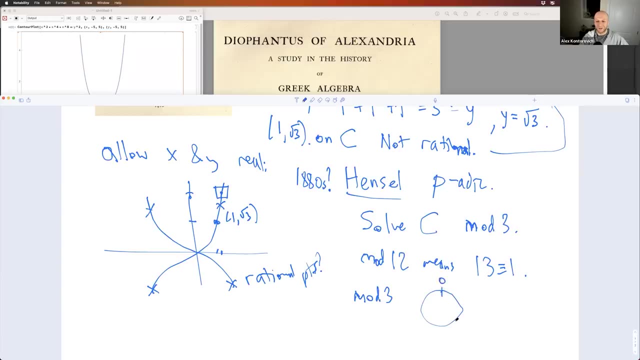 So, in other words, modular arithmetic is only about finding the remainder. 36 modulo 10, or 36 mod 10, is 6. And 25 mod 5 is 0.. Mod 3 means your clock only has 3 numbers on it: 0,, 1, and 2.. 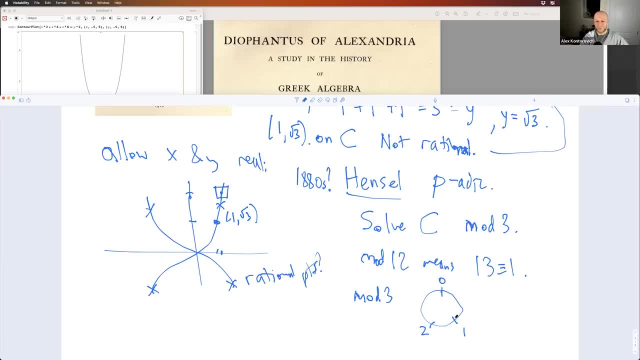 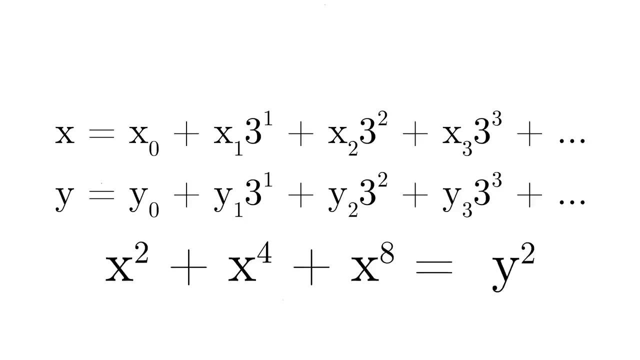 And if you multiply 2 by 2, you get 4, and 4 is the same thing as 4 o'clock is the same thing as 1 o'clock on a 3 hour clock. What's great about this approach is it allows us to work out the coefficients in our expansion. 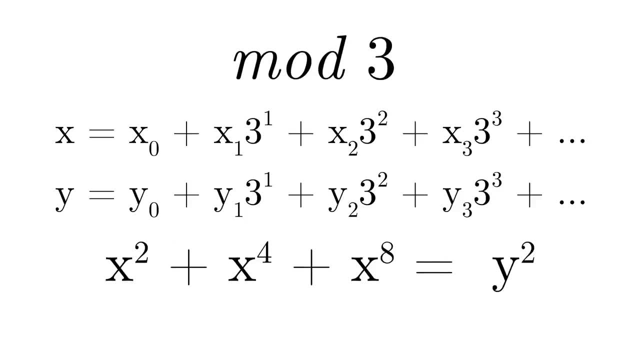 one at a time, by first solving the equation mod 3, and then mod 9, and then mod 27,, and so on. So first let's try to solve the equation mod 3.. And since all the higher terms are divisible by 3, they are all 0 if we're working mod. 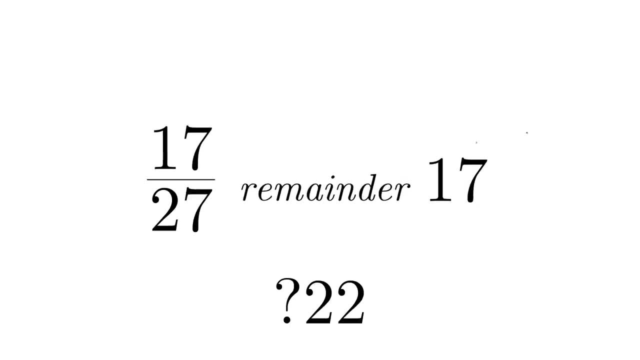 digit is 2.. Next divide 17 by 27 and you get a remainder of 17.. Subtract off the 8 we've already accounted for and you have 9.. So the 9's digit is 1.. So 17 in base 3 is 1,, 2, 2.. What we're doing here is a form of modular arithmetic In 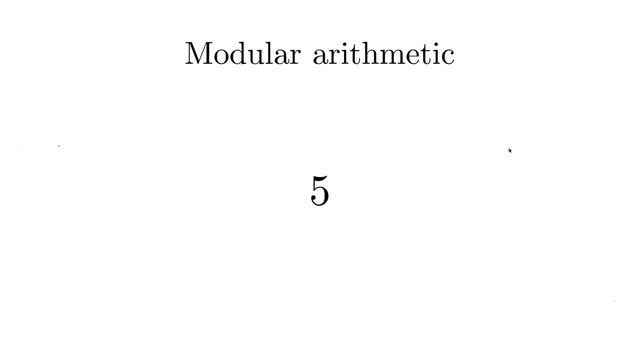 modular arithmetic numbers reset back to 0 once they reach a certain value called the modulus. The hours on a clock work kind of like this: with a modulus of 12. The hours increase up to 11, but then 12 o'clock is the same thing as 0 o'clock. 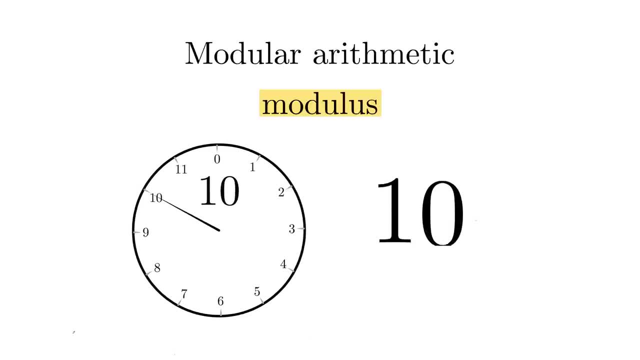 If it's 10 in the morning, say what time will it be in 4 hours? You could say 14,, but usually we'd say 2 pm, because 2 is 14 modulo 12. It's 2 more. 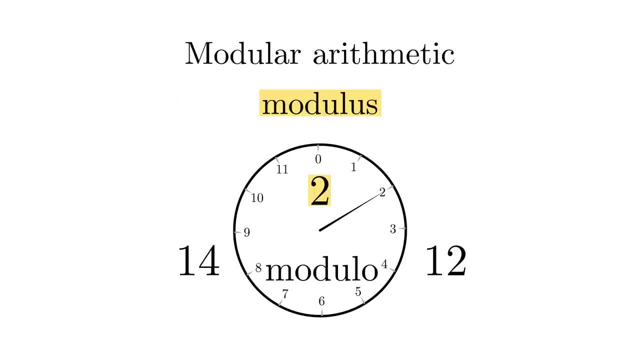 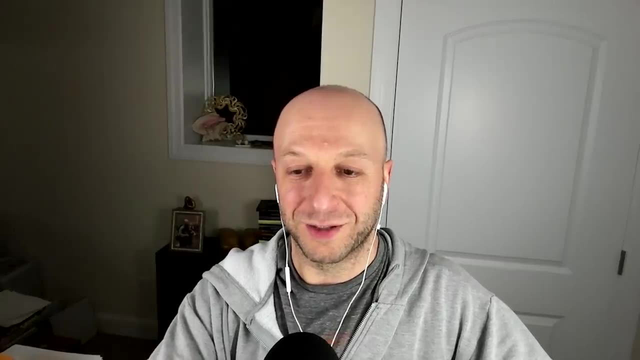 than a multiple of 12.. So, in other words, modular arithmetic is only about finding the remainder. 36 modulo 10, or 36 mod 10 is 6 and 25 mod 5 is 0.. Mod 3 means your clock only has three numbers on it: 0,, 1, and 2.. 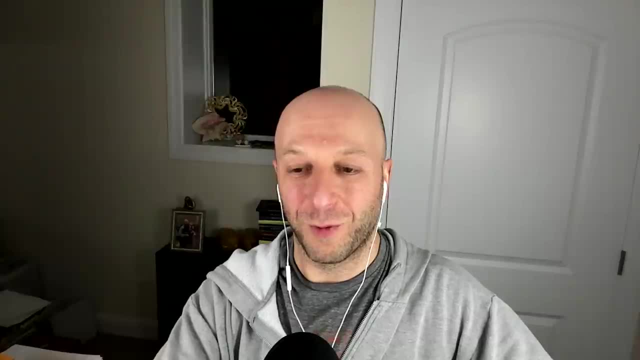 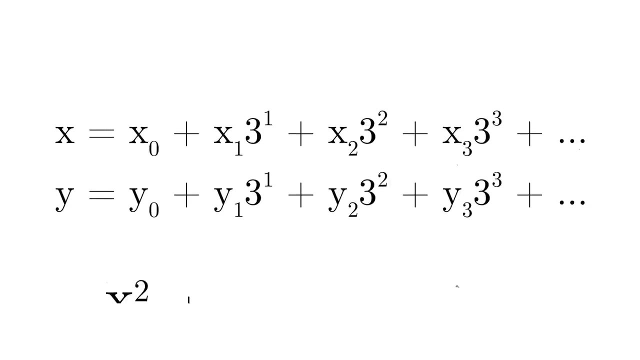 And if you multiply 2 by 2, you get 4, and 4 is the same thing as 4 o'clock, the same thing as 1 o'clock on a 3-hour clock. What's great about this approach is it allows us to. 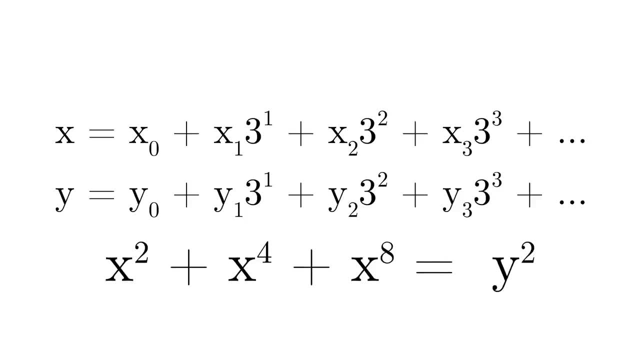 work out the coefficients in our expansion one at a time, by first solving the equation mod 3, and then mod 9, and then mod 27,, and so on. So first let's try to solve the equation mod 3.. And since all the higher terms are divisible by 3, they're all 0 if we're working mod 3.. 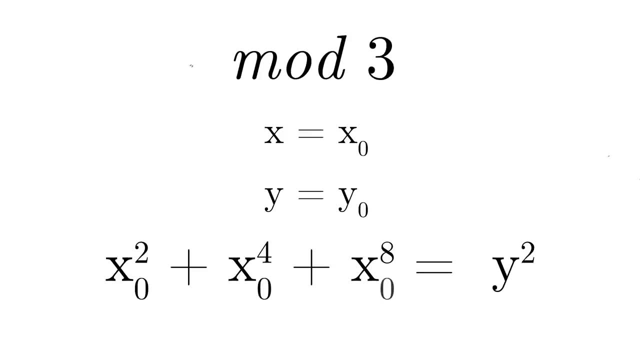 So we're left with x-naught squared, plus x-naught to the fourth, plus x-naught to the eight, equals y-naught squared, And this will allow us to find the values of x-naught and y-naught that satisfy the equation mod 3.. Now we know that x-naught can be either 0,. 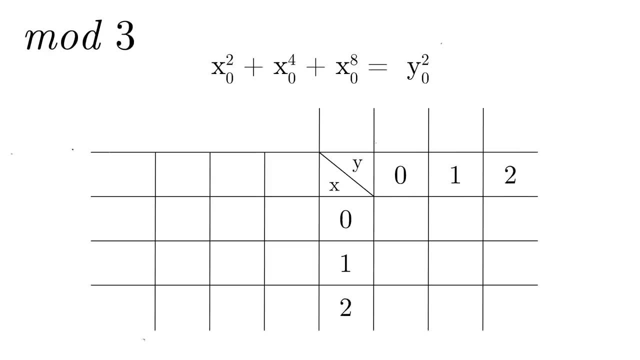 1, or 2,, and y-naught can also be either 0,, 1, or 2.. If x is 0,, then so is x squared, x to the 4, and x to the 8.. If x is 1,, then x squared is 1, and so is x to the 4 and x. 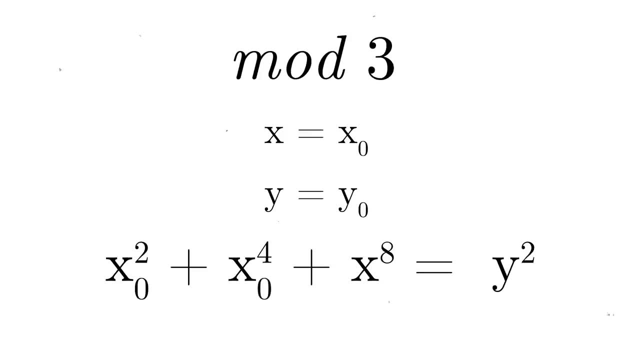 3.. So we're left with x0 squared plus x0 to the 4th, plus x0 to the 8, equals y0 squared. This will allow us to find the values of x0 and y0 that satisfy the equation mod 3.. 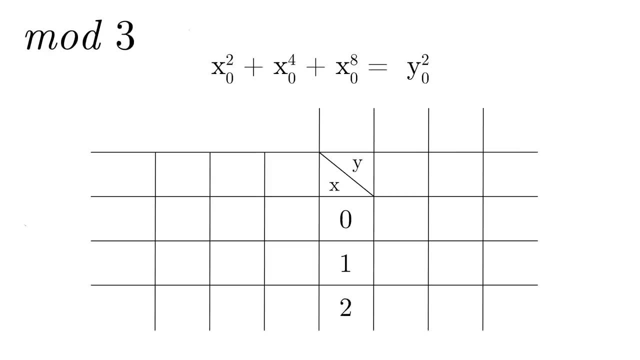 Now we know that x0 can be either 0,, 1, or 2, and y0 can also be either 0,, 1, or 2.. If x is 0, then so is x, squared x to the 4th. 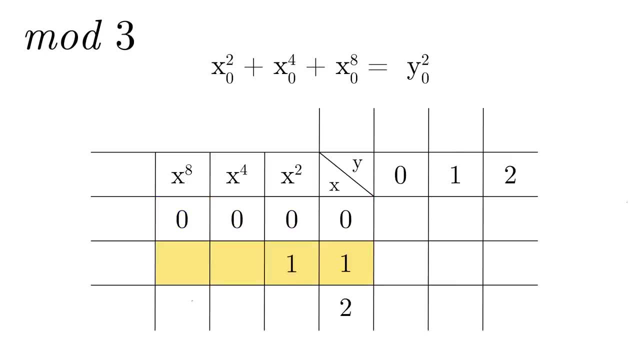 If x is 1, then x squared is 1, and so is x to the 4 and x to the 8.. If x is 2, then x squared is 4, but remember, we're working mod 3, and 4. mod 3 is just 1.. 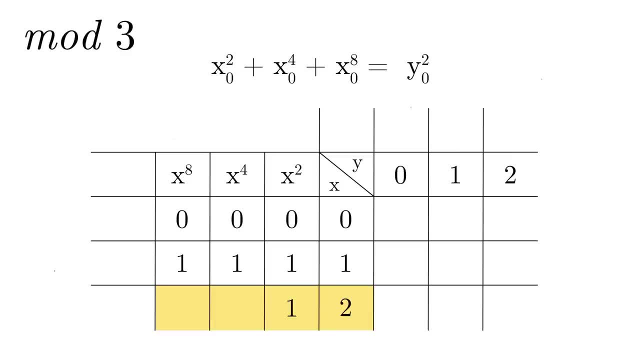 To find x to the 4, we can just square x squared so that also equals 1.. And squaring again x to the 8 equals 1.. Now we can sum up: x squared plus x to the 4 plus x to the 8 to find the left hand side. 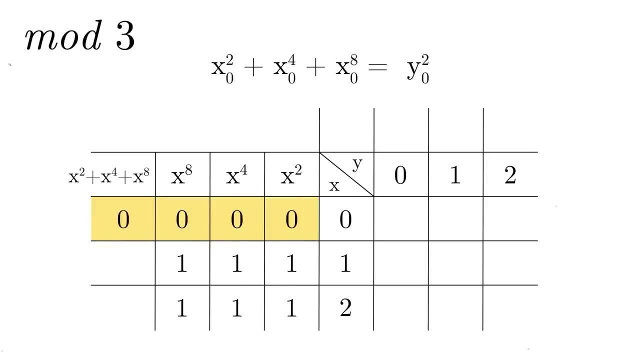 of the equation: If x is 0, then the sum is equal to 0.. If x is 1 or 2, the sum is 3, but again we're working mod 3, so 3 is the same as 0. 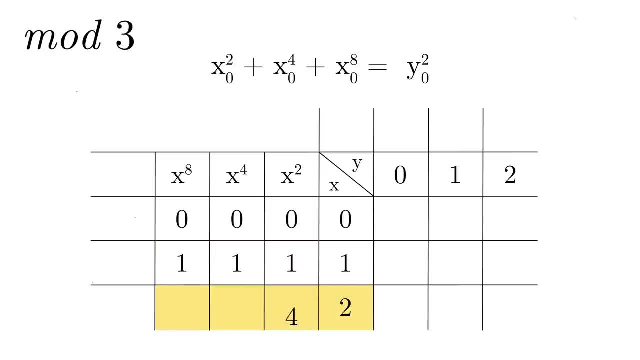 to the 8. If x is 2, then x squared is 4.. But remember, we're working mod 3, and 4. mod 3 is just 1.. To find x to the 4, we can just square x squared, so that also equals 1.. And squaring again. 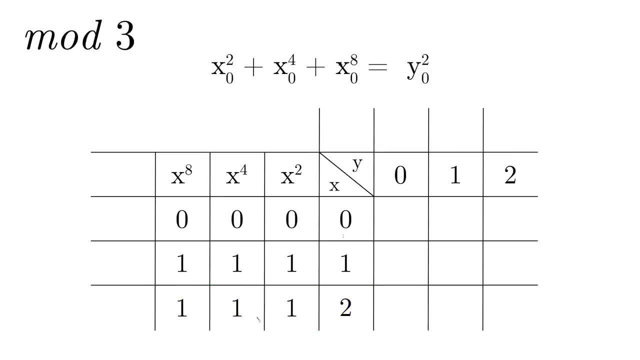 x to the 8 equals 1.. Now we can sum up x squared plus x to the 4, plus x to the 8, to find the left-hand side of the equation. If x is 0,, then the sum is equal to 0.. If x is 1 or 2,, the sum is 3.. 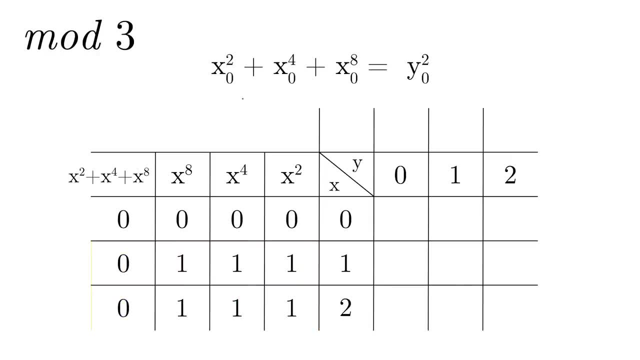 But again we're working mod 3, so 3 is the same as 0.. Now let's calculate y squared. If y is 0, y squared is 0. If y is 1, y squared is 1.. And if y is 2, then y squared is 4, but again 4 mod 3 is 1.. 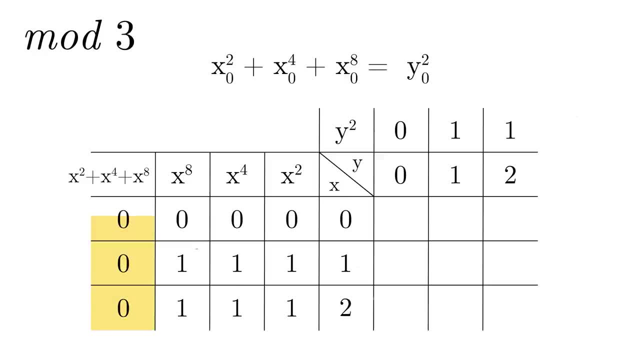 Now, since for all values of x, the left-hand side of the equation is 0, and since we now have a formula of everything that needs to satisfy x and y, we just draw half y and then find 2 for both sides and it eventually comes out boring. Now let's discuss the union of x, y and z and its limitations. So if y is 0,, y is 1, and if y is 2, then y squared is 0.. And if y is 2,, then y squared. 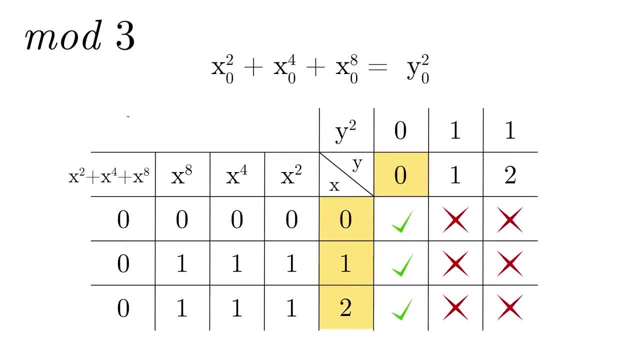 is 4.. But again, 4 mod 3 is 1.. Now, since for all values of x, the left-hand side of the equation is zero, the only value of y that satisfies, So we have three potential solutions that satisfy our equation, mod 3.. 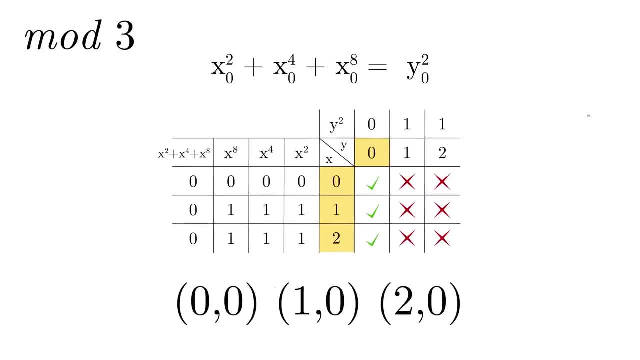 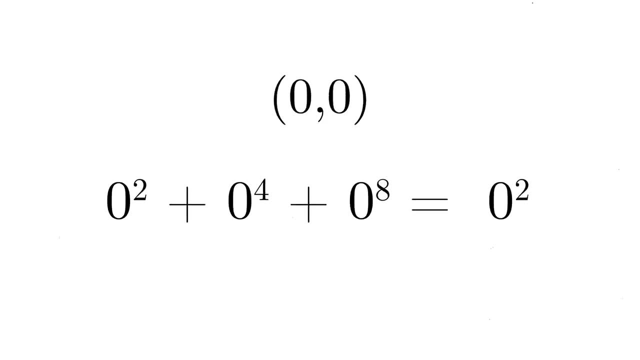 We've got 0, 0,, 1, 0, and 2, 0.. Now we shouldn't be surprised to find 0, 0 as a solution, since x equals 0 and y equals 0 does satisfy the equation. 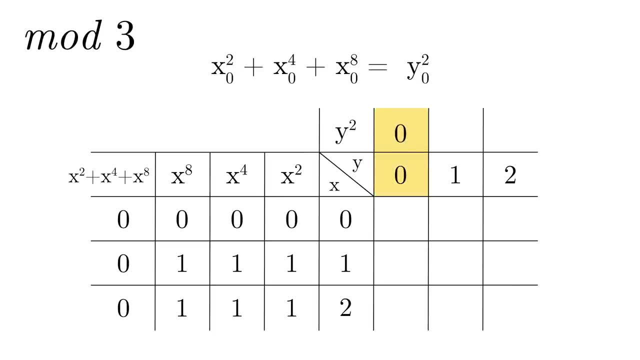 Now let's calculate y squared. If y is 0, y squared is 0.. If y is 1, y squared is 1.. And if y is 2, then y squared is 4, but again, 4 mod 3 is 1.. 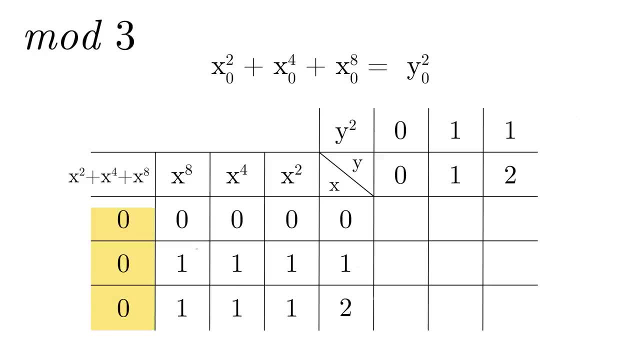 Now, since for all values of x, the left hand side of the equation is 0, the only value that satisfies the equation is: y equals 0. But x can be 0,, 1, or 2.. So we have three potential solutions that satisfy our equation, mod 3.. 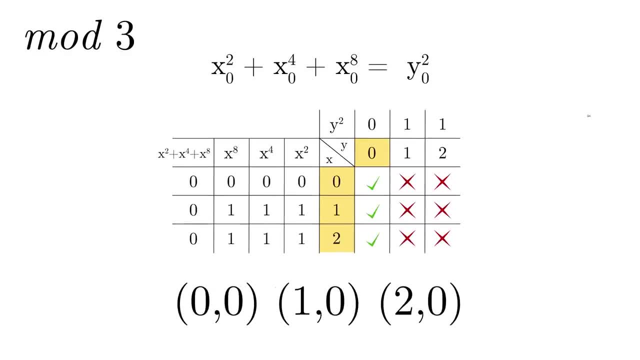 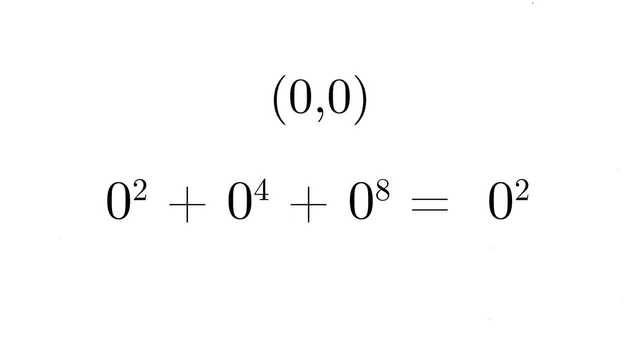 We've got 0, 0,, 1, 0, and 2, 0.. Now we shouldn't be surprised to find 0, 0 as a solution, since x equals 0 and y equals 0 does satisfy the equation. 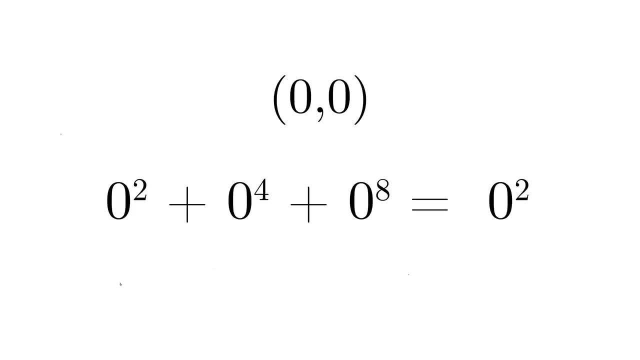 But squares of 0 size don't really count as solutions to Diophantus' geometric problem, So let's try to expand on one of the other solutions. I'll pick 1, 0.. This means x0 equals 1, and y0 equals 0 satisfies the equation mod 3.. 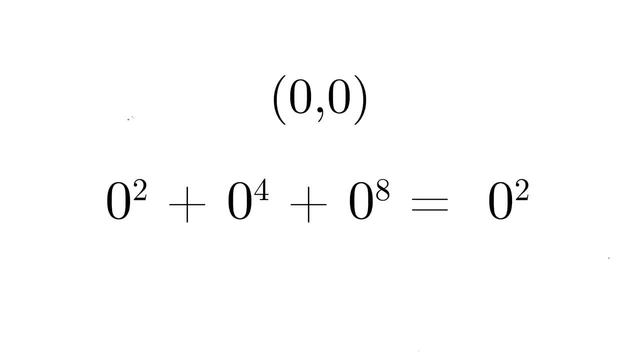 But squares of 0 size don't really count as solutions to Diophantis' geometric problem, So let's try to expand on one of the other solutions. I'll pick 1, 0.. This means x0 equals 1 and y0 equals 0 satisfies the equation mod 3.. 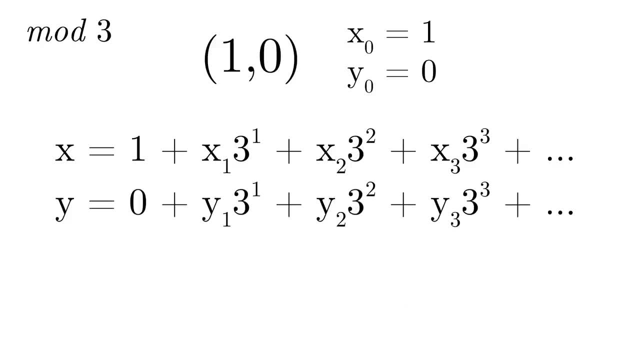 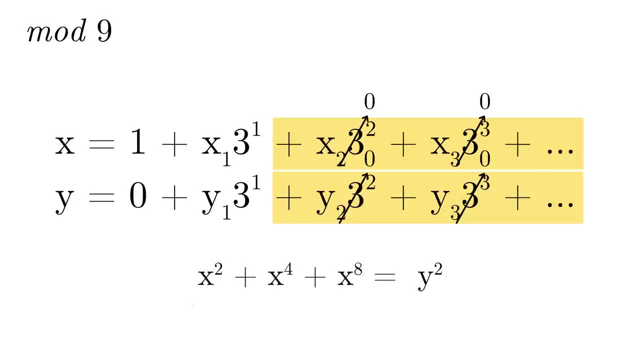 Now let's try to find x1.. And we'll do this by solving the equation mod 9.. All of the terms higher than x1 have a factor of 9 in them, so they're all 0 mod 9.. So we're left with this expression. 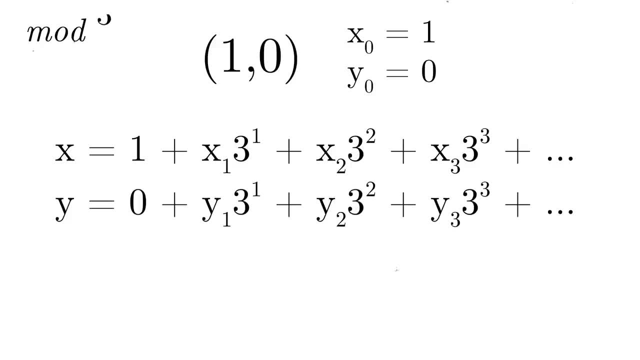 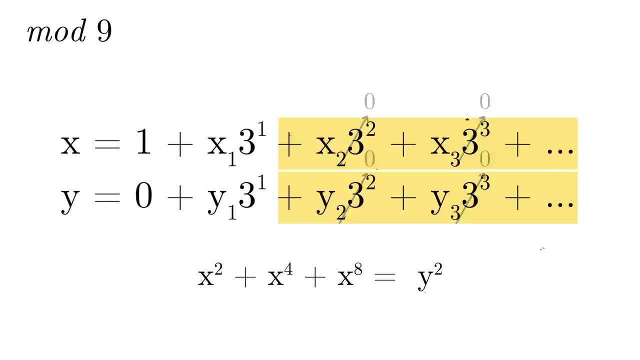 Now let's try to find x1,, and we'll do this by solving the equation mod 9.. All of the terms higher than x1 have a factor of 9 in them, so they're all 0 mod 9.. So we're left with this expression. 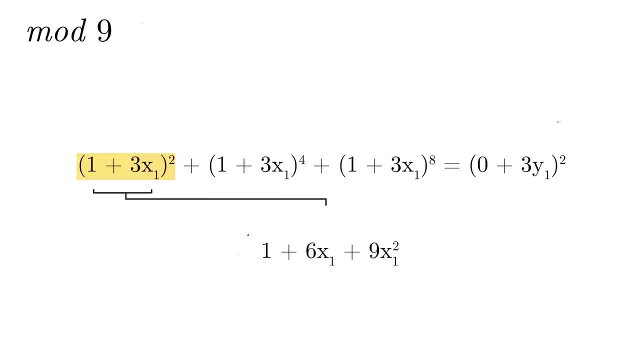 Expanding out the first term, we have 1 plus 6x1 plus 9x1 squared, But again, since we're working mod 9, the last part is 0.. The next term is just the first term squared, so that equals 1 plus 12x1 plus 36x1 squared. 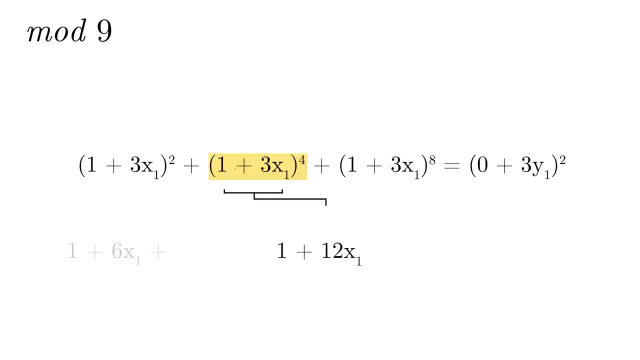 But 36 is 9 times 4,, so that's 0 mod 9.. And 12 mod 9 is 3, so we have 1 plus 3x1.. The final term is just that squared. so 1 plus 6x1 plus 9x1 squared. 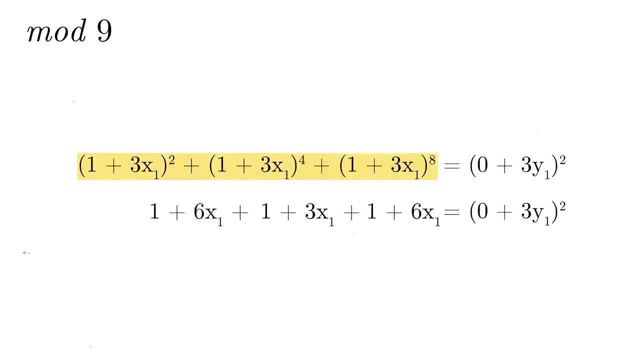 Again, the last part is 0.. So on the left-hand side We have 3 plus 15x1.. And on the right-hand side we have 0 plus 9y1 squared, which is also 0 because it contains. 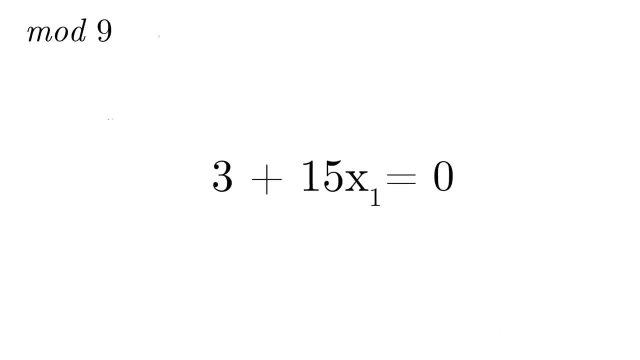 a factor of 9.. So 3 plus 15x1 equals 0.. Now remember, since we're working mod 9, the 0 on the right-hand side represents any multiple of 9.. So in this case, if x1 equals 1, then 3 plus 15 equals 18,, which is a multiple of 9.. 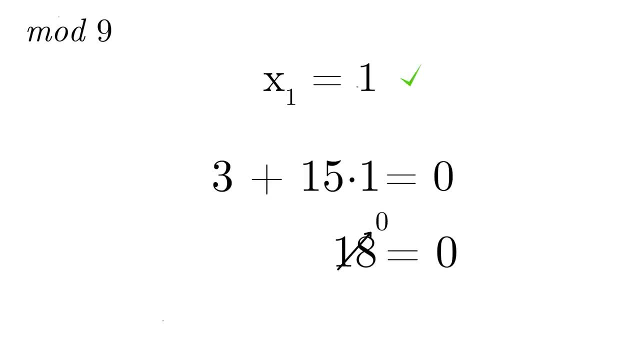 So it's 0.. So x1 equals 1.. And x equals 1 is a solution to the equation. Let's find one more term of the expansion by solving the equation mod 27.. Again, all the terms with 3 raised to the power of 3 or higher contain a factor of 27,. 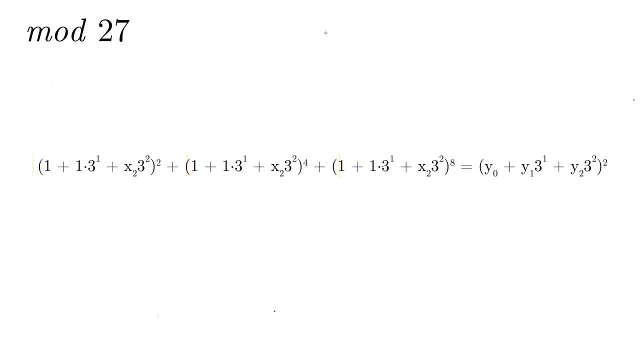 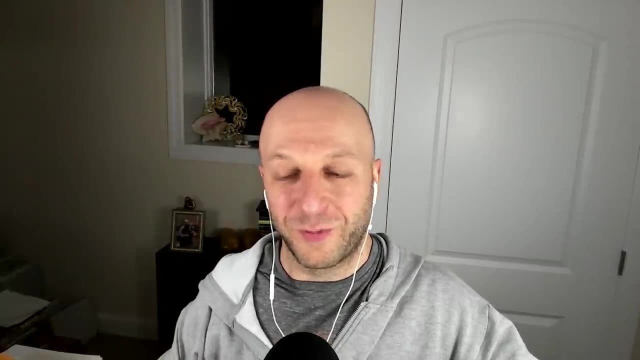 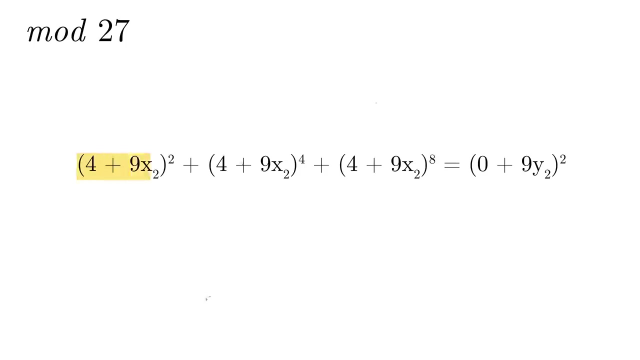 so they're 0, leaving only this expression. But we know x0 and x1 are equal to 1.. But right now we've learned nothing about y1.. Because when we square, anything can happen with a good solution in y, so we can simplify to this. expanding again, we get 16 plus 18 x2. 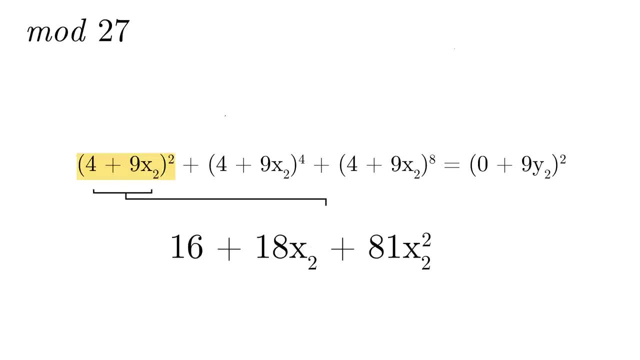 plus 81 x squared, but 81 is 27 times 3, so that's 0.. the next term is the square of the first, so 256 plus 576 x2 plus 324 x2 squared, but 324 is 27 times 12, so that's 0. and since we're working mod, 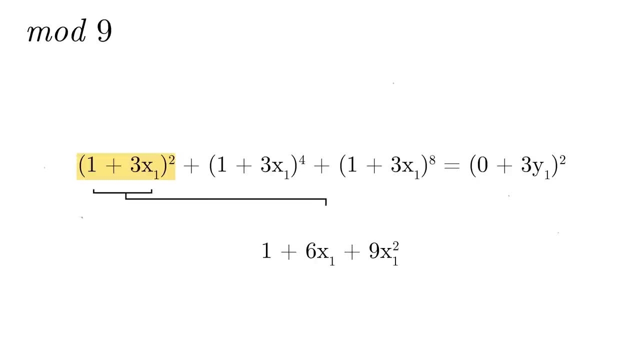 Expanding out the first term, we have 1 plus 6x1 plus 9x1 squared. But again, since we're working mod 9, the last part is 0.. The next term is just the first term squared. 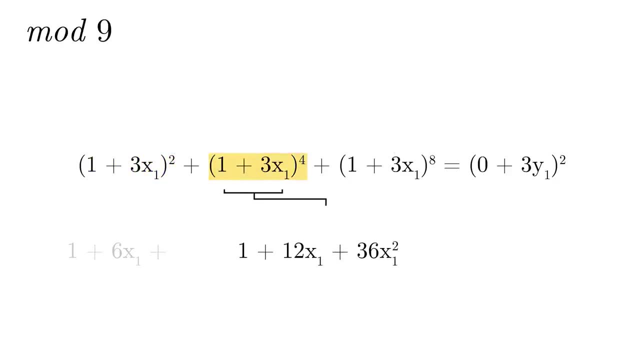 So that equals 1 plus 12x1 plus 36x1 squared. But 36 is 9 times 4, so that's 0 mod 9.. And 12 mod 9 is 3, so we have 1 plus 3x1.. 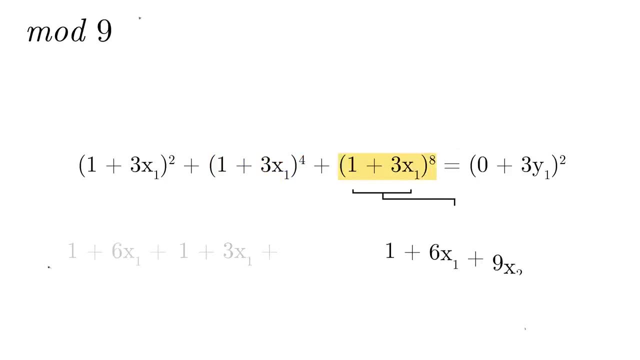 The final term is just that, squared. So 1 plus 6x1 plus 9x1. squared Again, the last part is 0.. So on the left-hand side we have 3 plus 15x1.. And on the right-hand side we have 0 mod 9.. 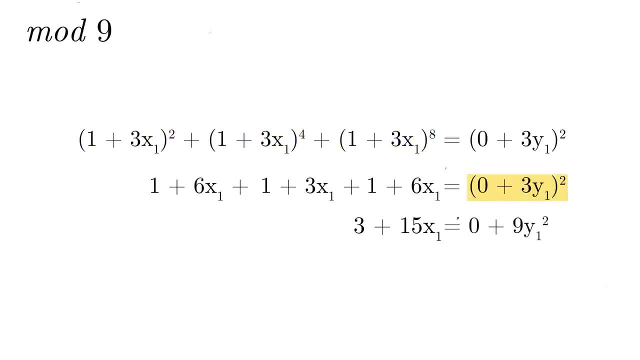 So we have 0 plus 9y1 squared, which is also 0 because it contains a factor of 9.. So 3 plus 15x1 equals 0.. Now remember, since we're working mod 9, the 0 on the right-hand side represents any multiple of 9.. 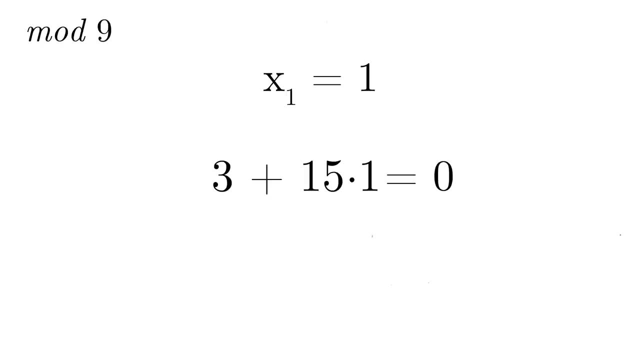 So in this case, if x1 equals 1, then 3 plus 15 equals 18,, which is a multiple of 9.. So it's 0.. So x1 equals 1 is a solution to the equation. Let's find one more term of the expansion. 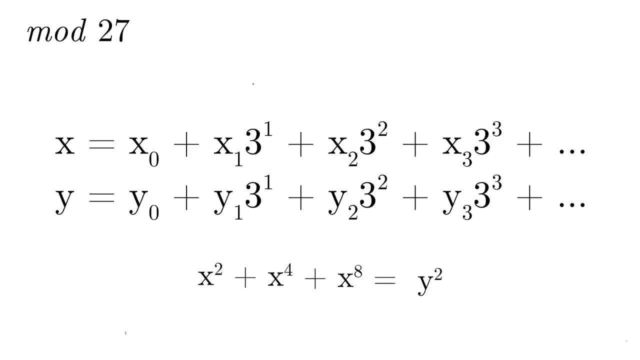 by solving the equation mod 27.. Again, all the terms with 3 raised to the power of 3 or higher contain a factor of 27.. So they're 0, leaving only this expression. But we know x0 and x1 are equal to 1.. 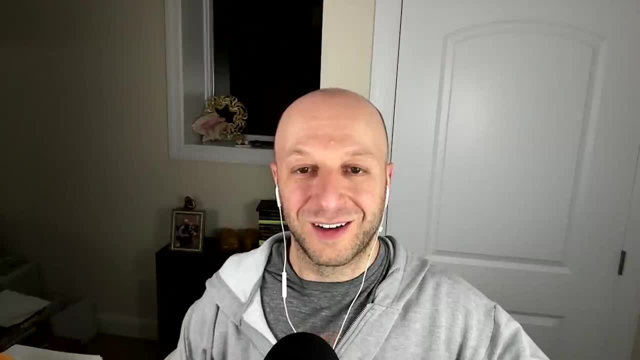 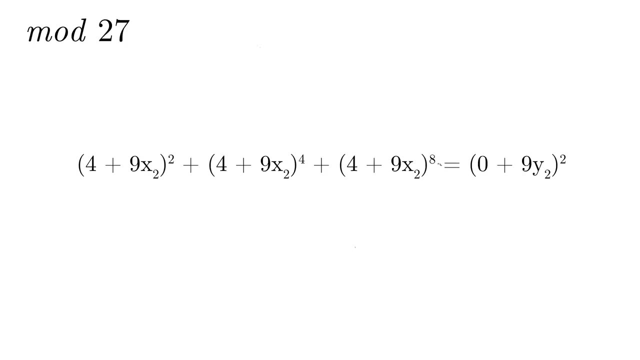 But right now we've learned nothing about y1.. Because when we square, anything can happen: If we find a good solution in x, it'll come with a good solution in y. So we can simplify to this Expanding again. 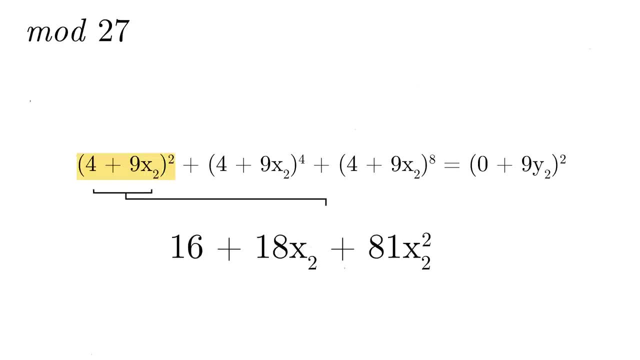 we get 16 plus 18x2 plus 81x2.. But 81 is 27 times 3.. So that's 0.. The next term is the square of the first, So 256 plus 576x2 plus 324x2 squared. 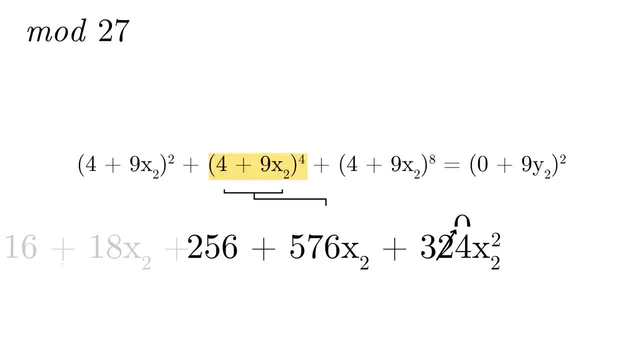 But 324 is 27 times 12.. So that's 0.. And since we're working mod 27, we can simplify this down: 576 is 9 more than a multiple of 27.. And 256 is 13 more than a multiple of 27.. 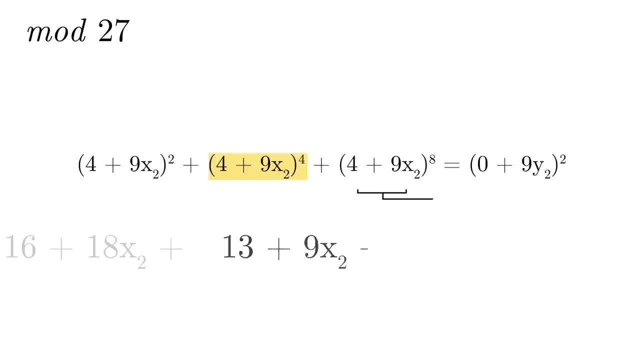 So we're left with 13 plus 9x2.. And the last term is just that squared. So 169 plus 234x2 plus 81x2 squared, Which reduces to 7 plus 18x2.. The right hand side reduces to 0 plus 81y squared. 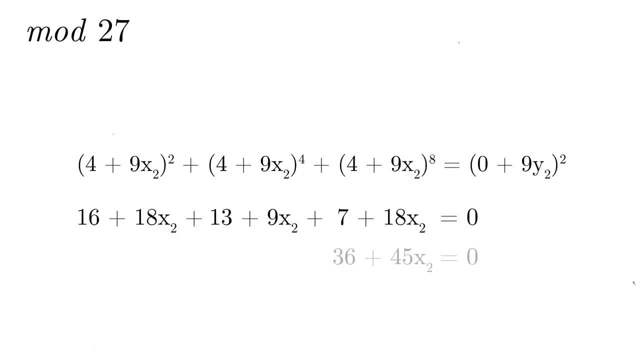 Which is again 0.. So we have 36 plus 45x2 equals 0.. Which mod 27, is the same as 9 plus 18x2.. So 9 plus 18x2 equals 0. So x2 must be equal to 1.. 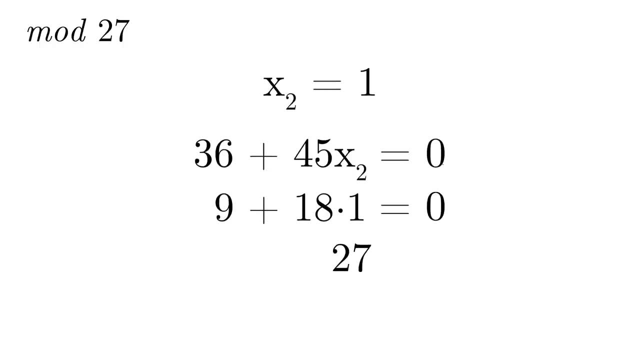 9 plus 18 is 27.. Which mod 27 is 0. So what we've discovered is the first three coefficients in our expansion are all 1.. And in fact, if you kept going with modulus 81,, 243, and so on, 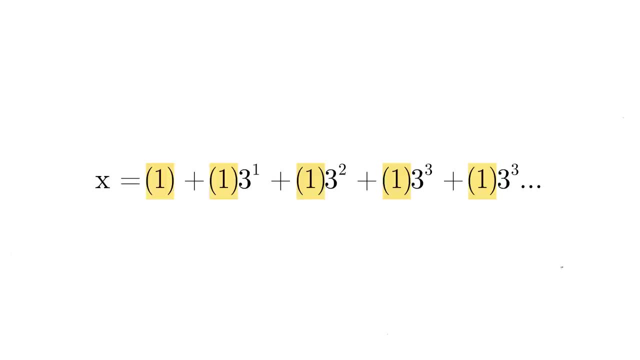 you would find that all of the coefficients are 1.. So the number that solves Diophantus' equation about the squares is actually a 3-adic number where all the digits are 1s. But how do we make sense of this? 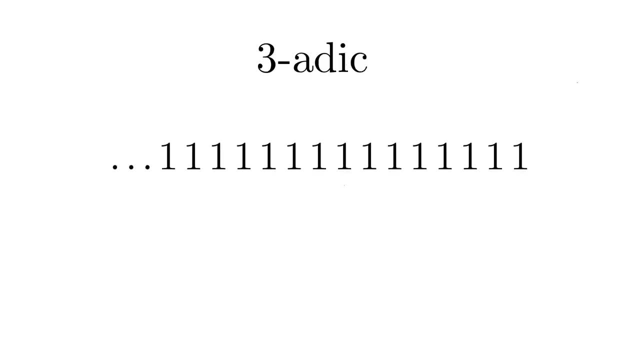 What does this number equal? And, of course, this number makes no sense at all, At least not as a real number. Well, remember that this is just another way of writing: 1 times 3 to the 0 plus 1 times 3 plus 1 times 3 squared, plus 1 times 3 cubed, and so on. 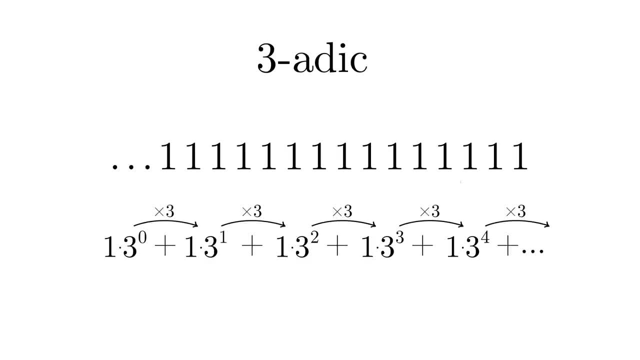 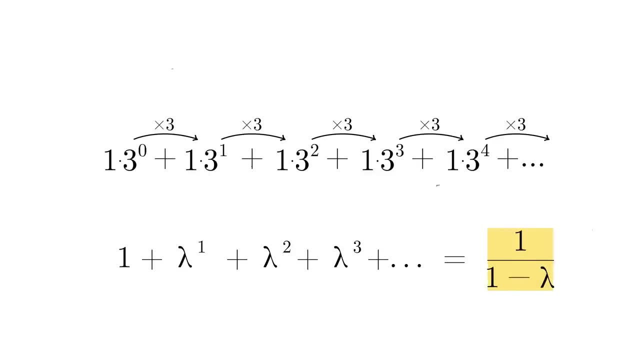 So each term is just 3 times the term before it. This is a geometric series, The sum of an infinite geometric series. you can use the equation 1 over, 1 minus lambda, where lambda is the ratio of one term to the previous one. 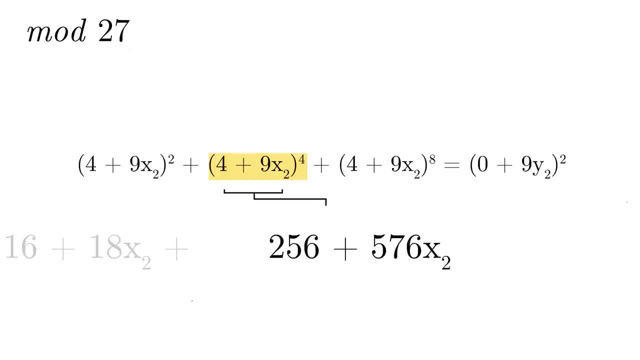 27. we can simplify this down: 576 is 9 more than a multiple of 27, and 256 is 13 more than a multiple of 27, so we're left with 13 plus 9 x2, and the last term is just that squared. so 169 plus 234 x2 plus. 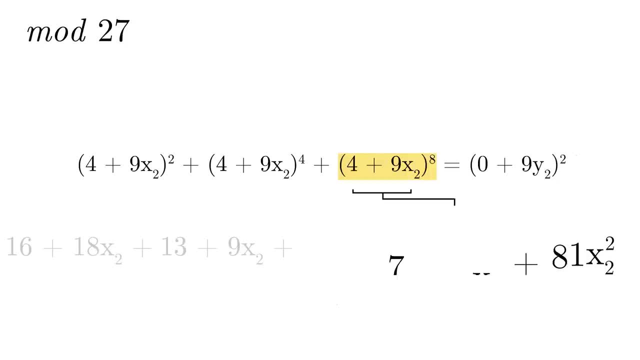 81 x2 squared, which reduces to 7 plus 18 x2. the right hand side reduces to 0 plus 81 y squared, which is again zero. so we have 36 plus 45 x2 equals 0, which mod 27 is the same as 9 plus 18 x2 equals 0.. so x2 must be. 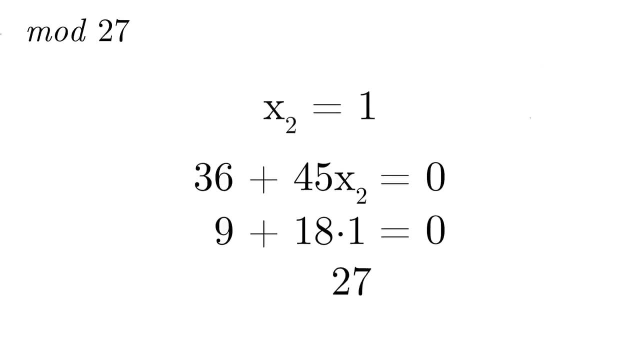 equal to 1.. 9 plus 18 is 27, which mod 27 is 0.. so what we've discovered is: the first three coefficients in our expansion are all 1 and in fact, if you kept going with modulus 81, 243 and so on, you would find: 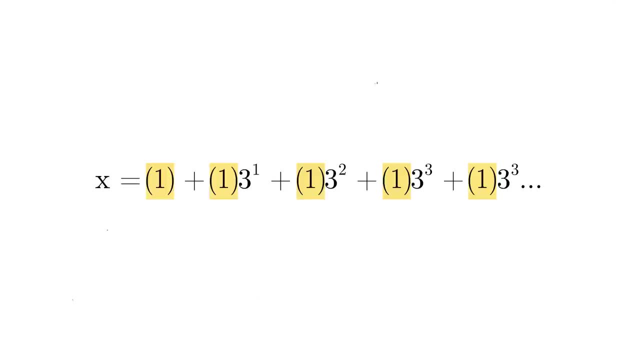 that all of the coefficients are 1.. so the number that solves diaphantis's equation about the squares is actually a three-adic number where all the digits are ones. but how do we make sense of this? what does this number equal? and of course, this number makes no sense at all, at least not as a 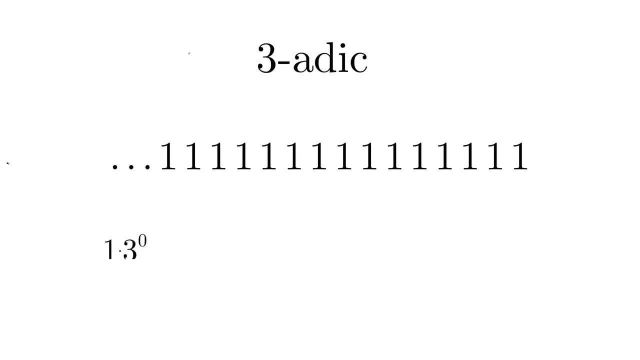 real number. well, remember that this is just another way of writing: 1 times 3 to the 0, plus 1 times 3 plus 1 times 3 squared, plus 1 times 3 cubed, and so on. so each term is just three times the term before it. this is a geometric series and to find the sum: 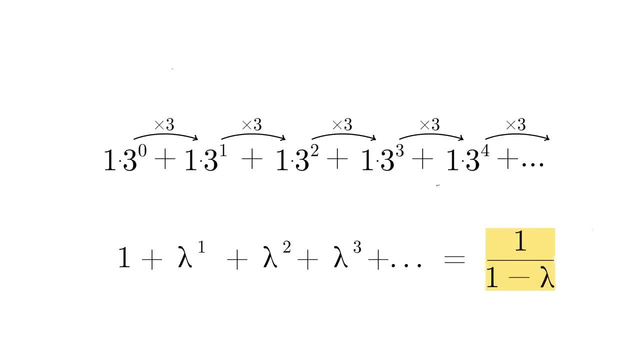 of an infinite geometric series. you can use the equation 1 over, 1 minus lambda, where lambda is the ratio of one term to the previous one, so in this case it's three. now i know, for this to work, lambda is meant to be strictly less than one, because otherwise the terms keep growing and 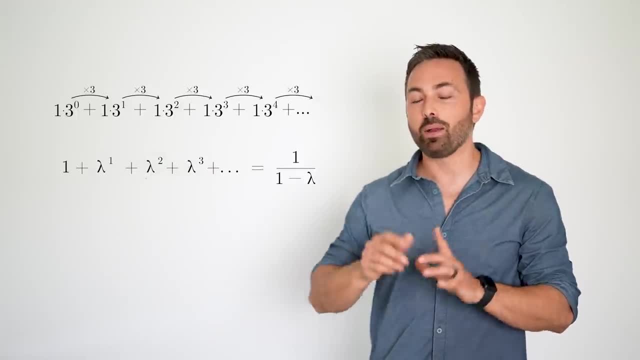 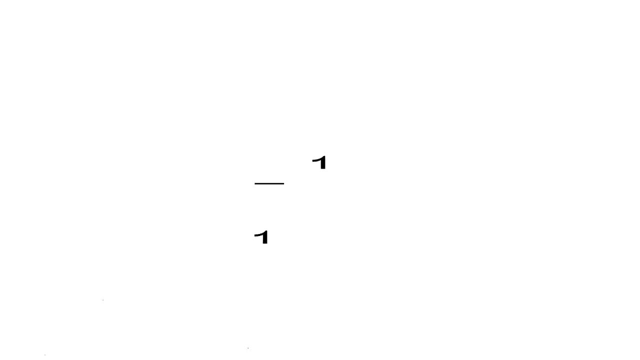 the sum doesn't converge, it just diverges to infinity. i promise i'll come back to this, but for now let's just say that lambda equals 3 and see what happens. well then we have 1 over 1 minus 3, which is negative a half. so if we believe this formula, then x equals negative a half should be. 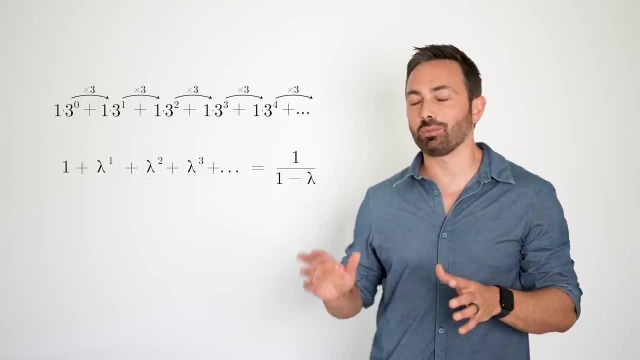 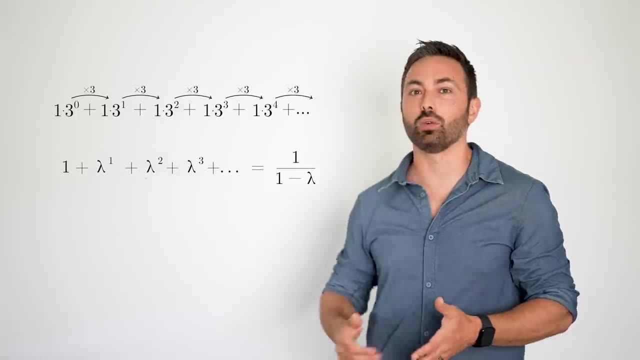 So in this case it's 3.. Now I know, for this to work, lambda is meant to be strictly less than 1, because otherwise the terms keep growing and the sum doesn't converge, It just diverges to infinity. I promise I'll come back to this. 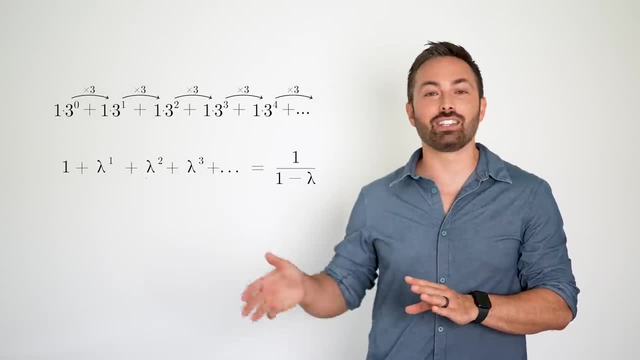 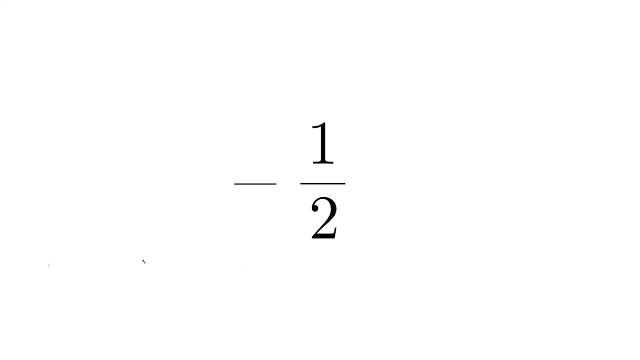 But for now let's just say that lambda equals 3 and see what happens. Well then we have 1 over 1 minus 3, which is negative 1 half. So if we believe this formula, then x equals negative 1 half should be a solution to our original equation. 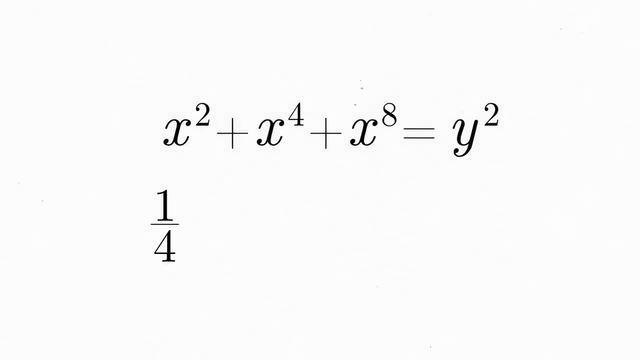 If we sub it in, we get x. squared is a quarter, x to the 4 is a 16th and x to the 8 is 1 over 256.. Let's put all of these over a common denominator, So a quarter becomes 64 over 256.. 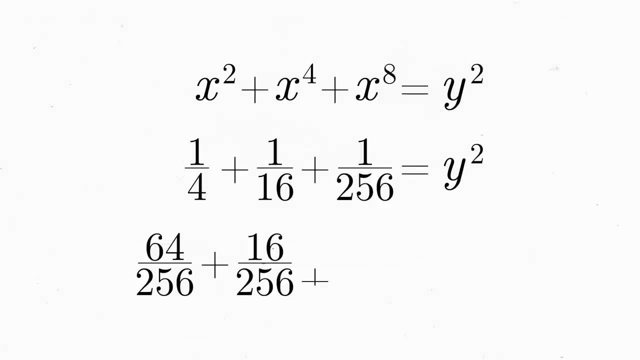 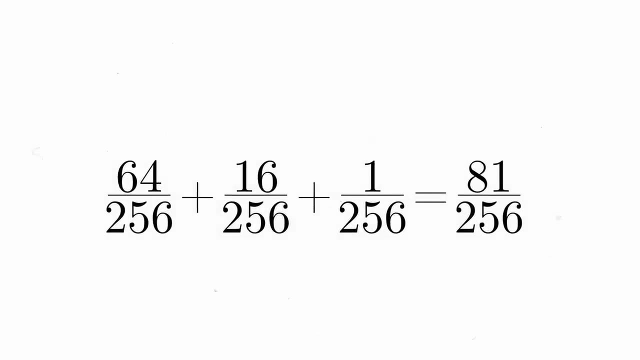 A 16th is 16 over 256.. And if we add them all together we get 81 over 256, which is indeed the area of a square with sides of length 9 16ths. We have found a rational solution to Diophantus' sum of squares problem. 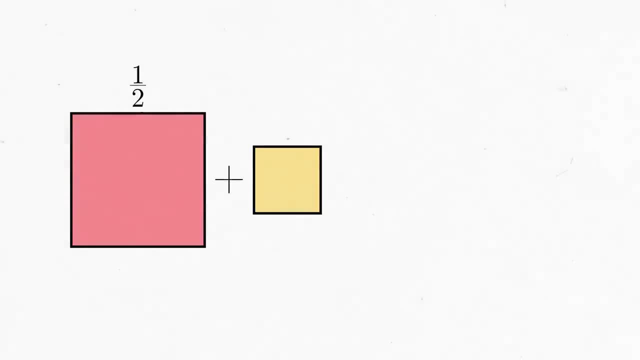 The first square has sides of length 1- half. The second has sides of length a quarter. The third has sides of length 1- 16th, And all three squares together make a square with sides of length 9- 16ths. To find this solution, 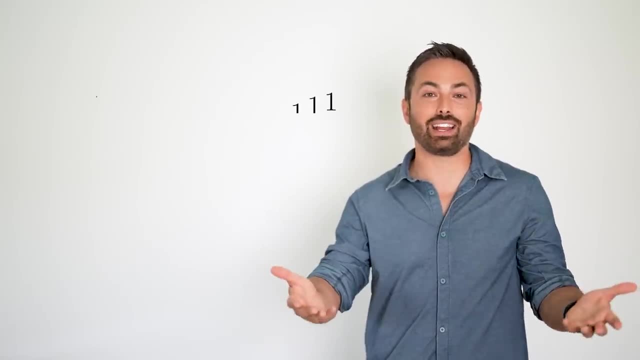 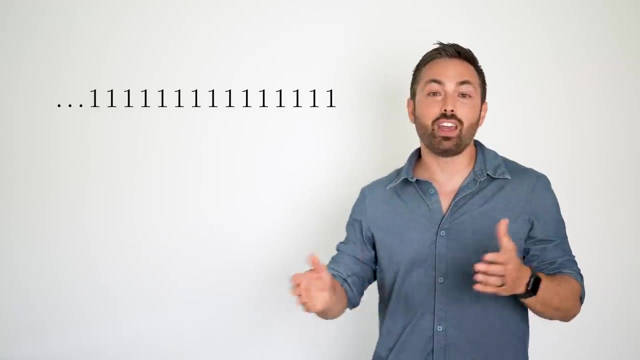 we used new, seemingly absurd numbers, p-adic, infinite digits going off to the left of the decimal point, implying an infinite expansion of increasing powers of 3.. Then we used the geometric series formula to find that an infinite string of 1s in 3-adic notation is actually negative 1 half. 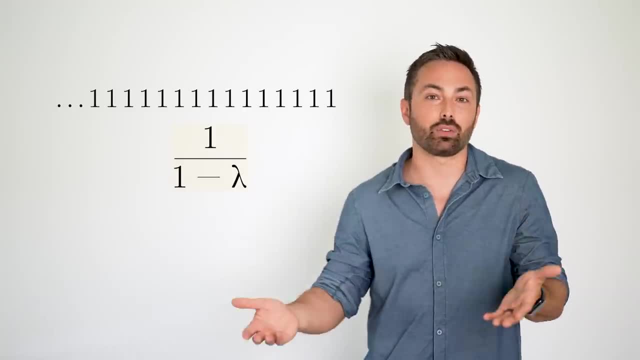 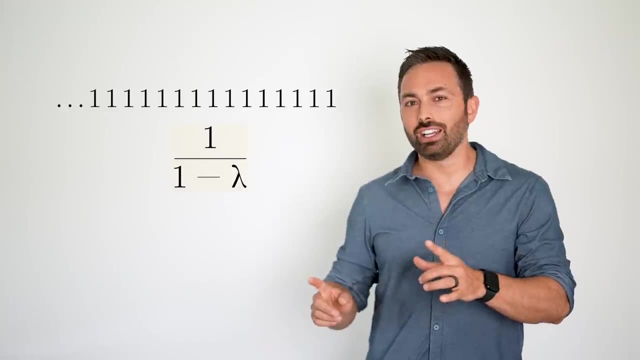 This works, even though the ratio of each term to the previous one is 3.. So, by common sense, the series shouldn't have converged. It should have blown up to infinity. So the real question is: how did this work? Well, the key idea is that the geometry of the p-adics 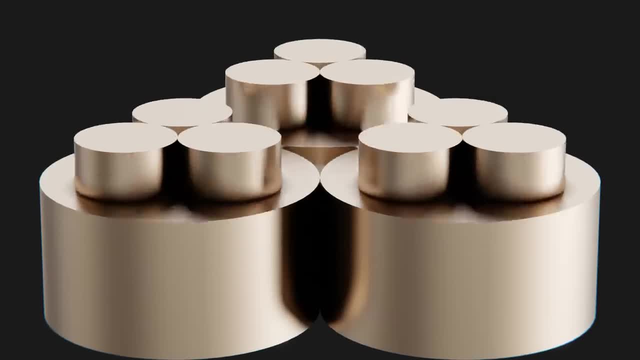 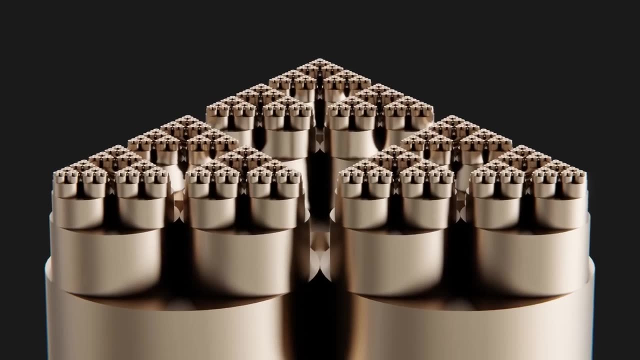 is totally different from that of the real numbers. In fact, they don't exist on a number line at all. One way to visualize them is with something like a growing tree. For the 3-adic integers we've been working with three base cylinders. represent the units digit. 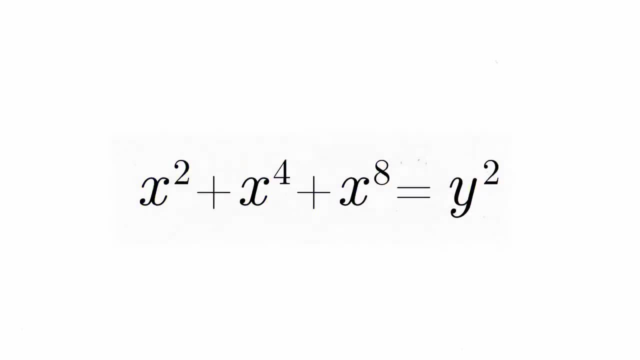 a solution to our original equation. if we sub it in, we get x squared is a quarter, x to the 4 is a 16th and x to the 8 is 1 over 256.. let's put all of these over a common denominator, so a quarter. 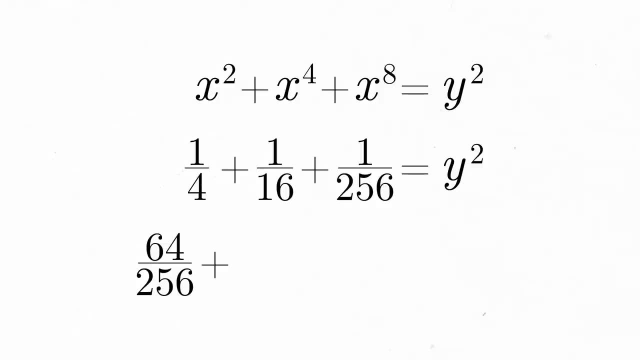 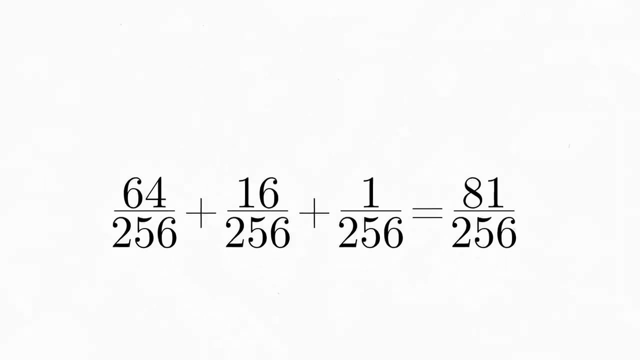 becomes 64 over 256. a 16th is 16 over 256 and if we add them all together, we get 81 over 256, which is indeed the area of a square with sides of length 9- 16.. we have found a rational solution. 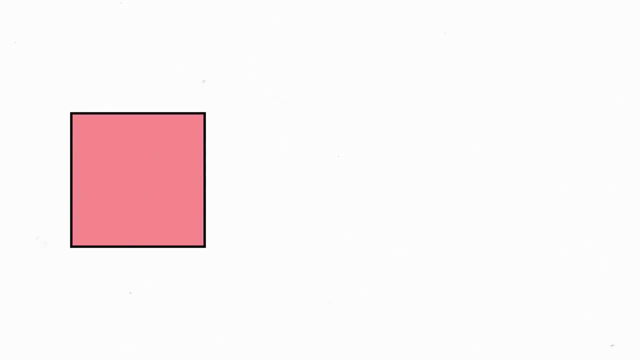 to diaphantis's sum of squares problem. the first square has sides of length one half, the second has sides of length a quarter, the third has sides of length one quarter and the fourth has sides of length a quarter. the third has sides of length a quarter. the third has sides of length a quarter. 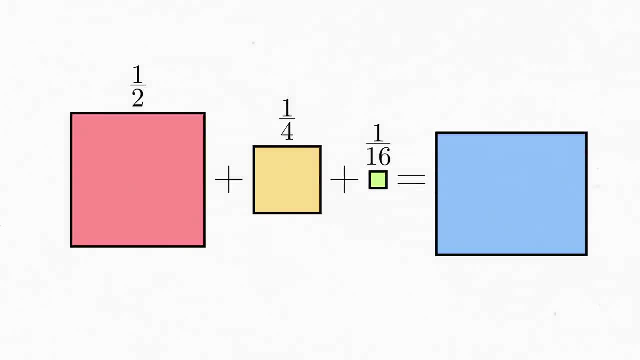 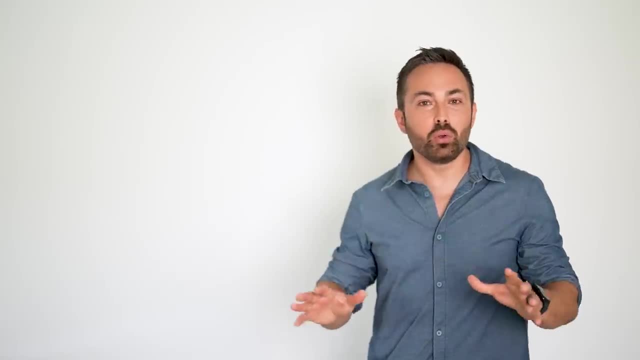 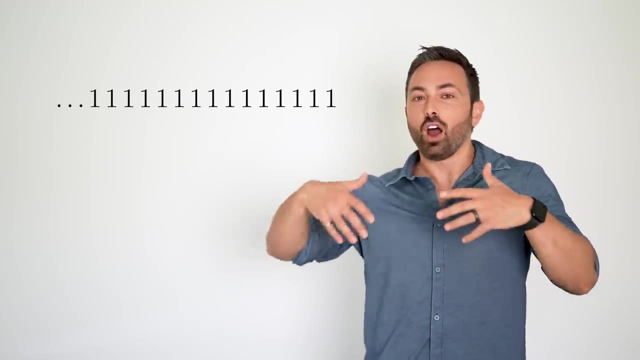 of length 1- 16th, and all three squares together make a square with sides of length 9- 16ths. To find this solution we used new, seemingly absurd numbers, p-adic infinite digits, going off to the left of the decimal point, implying an infinite expansion of increasing powers of three. 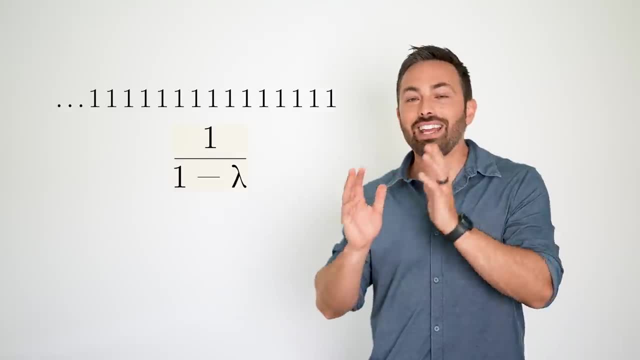 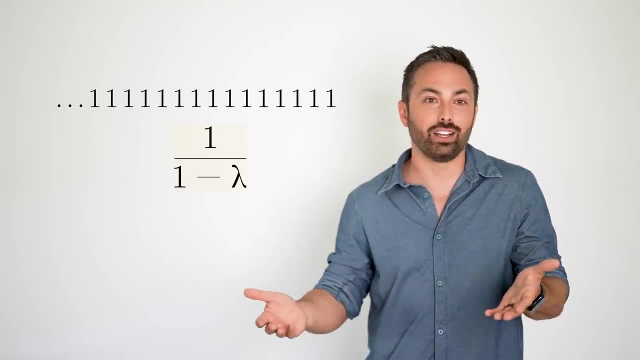 Then we used the geometric series formula to find that an infinite string of ones in three-adic notation is actually negative a half. This works even though the ratio of each term to the previous one is three. So by common sense the series shouldn't have converged. it should have. 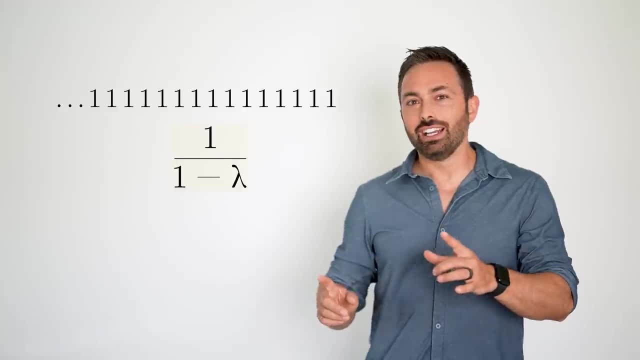 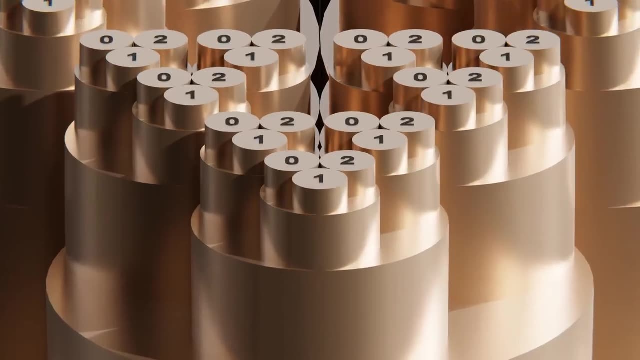 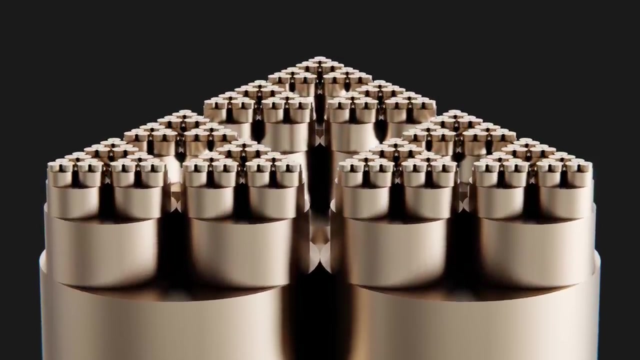 blown up to infinity. So the real question is: how did this work? Well, the key idea is that the geometry of the p-adics is totally different from that of the real numbers. In fact, they don't exist on a number line at all. One way to visualize them is with something like a growing tree. 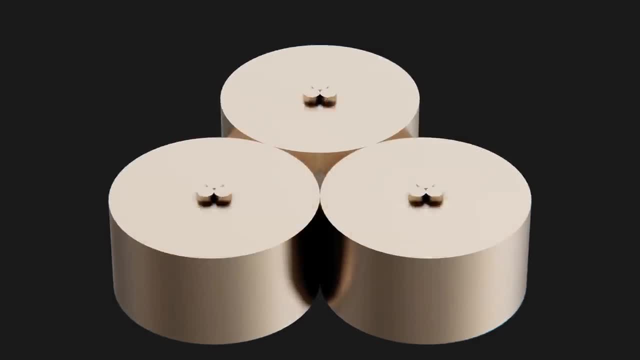 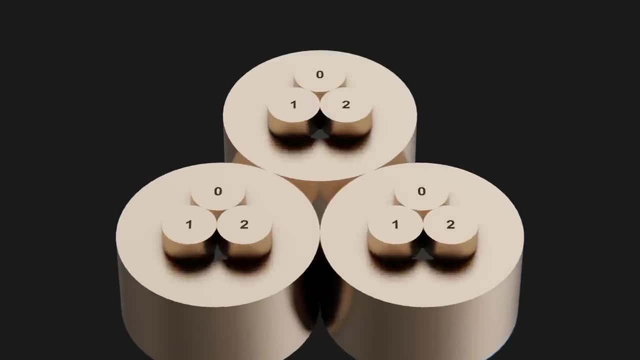 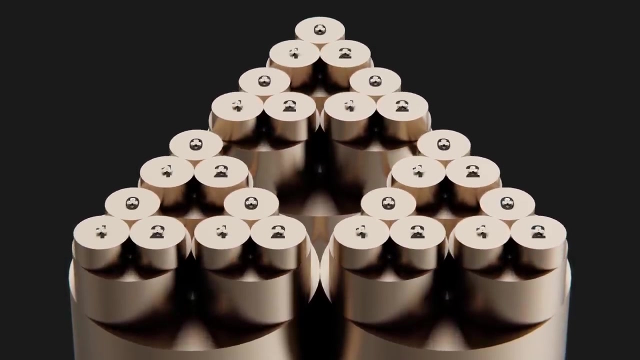 For the 3-adic integers we've been working with three base cylinders. represent the units digit or a x naught being 0,, 1, or 2.. Above each cylinder is a trio of shorter cylinders corresponding to the 3's digit or x1.. And we continue in this way forever, making an infinite triply branching tree. 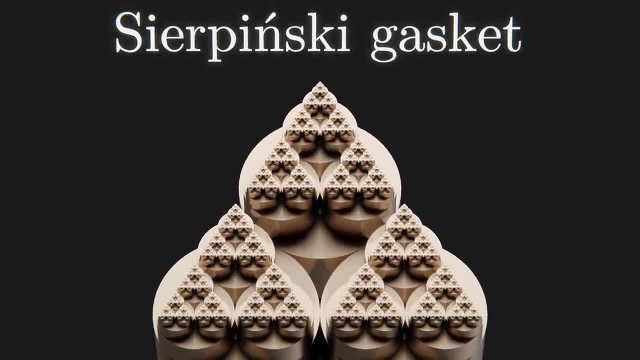 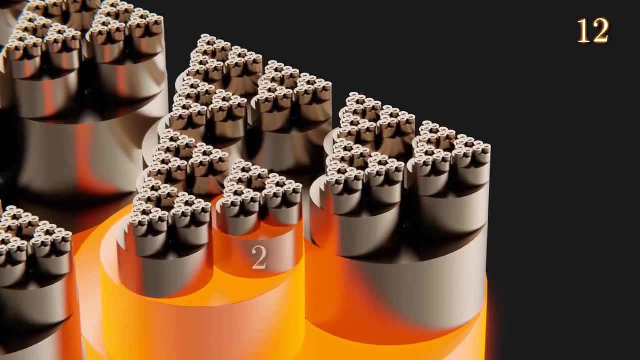 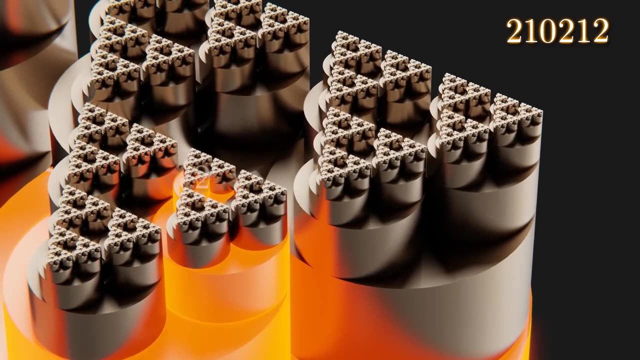 Looking down from above, it looks like a Sierpinski gasket. Each 3-adic number is represented here as a stack of infinite cylinders that get shorter and narrower as they go up, And this actually reflects the relative contributions each successive cylinder makes to the value of the. 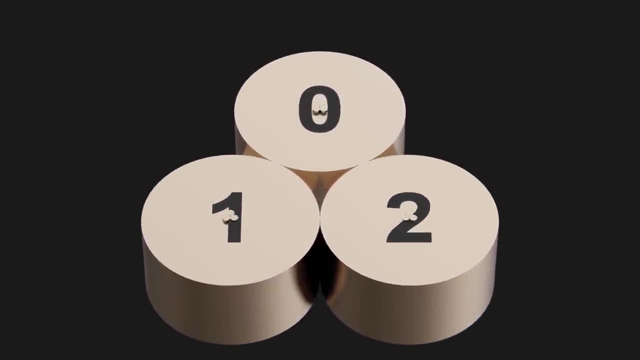 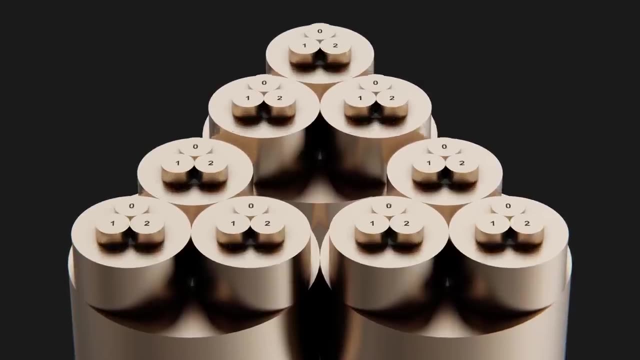 or x-naught being 0,, 1, or 2.. Above each cylinder is a trio of shorter cylinders corresponding to the 3s digit or x1. And we continue in this way forever, making an infinite triply branching tree. 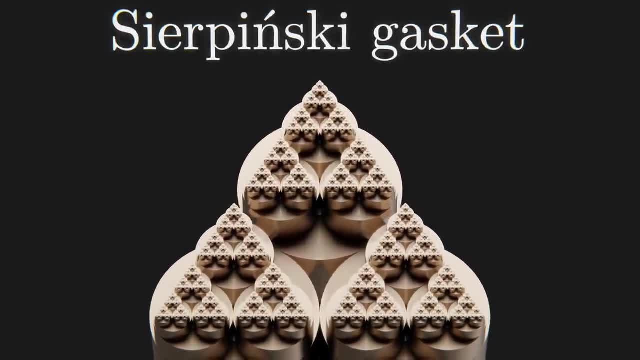 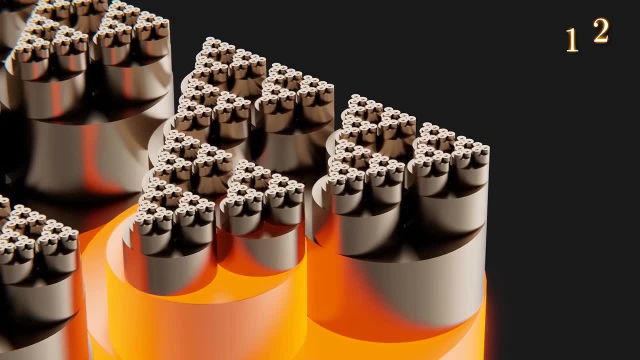 Looking down from above, it looks like a Sierpinski gasket. Each 3-adic number is represented here as a stack of infinite cylinders that get shorter and narrower as they go up, And this actually reflects the relative contributions each successive cylinder makes. 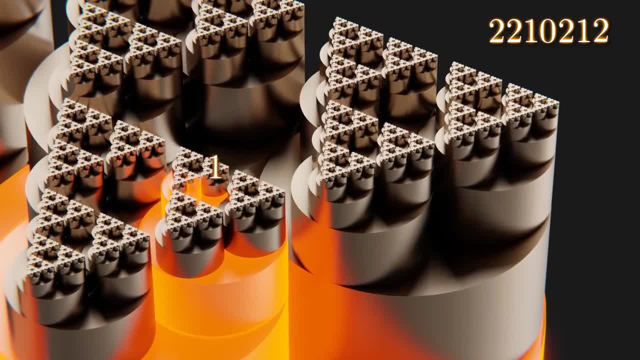 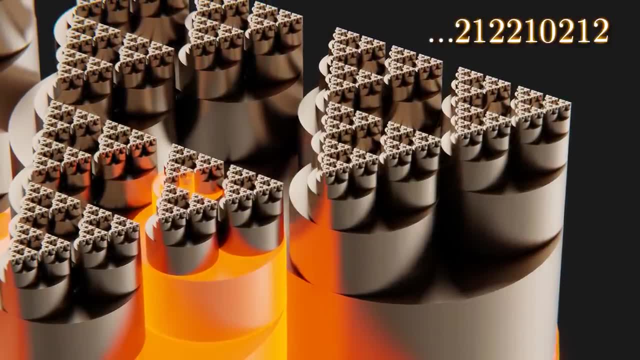 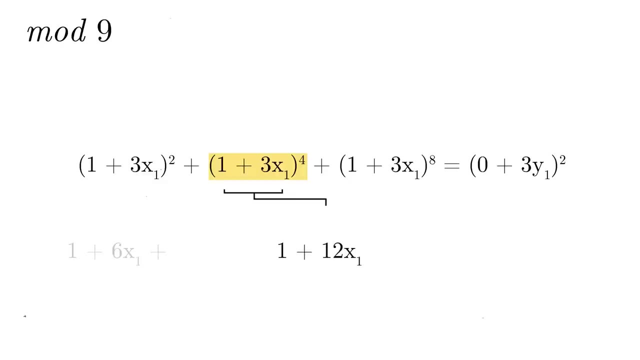 to the value of the 3-adic number. Contrary to what you'd expect, the coefficients multiplying higher powers of 3 actually make finer and finer adjustments. So when we calculated successive coefficients to solve Diophantus' squares problem, we were actually zooming in more and more accurately on the solution. 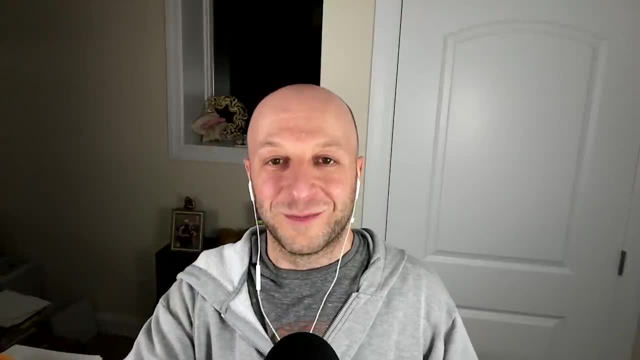 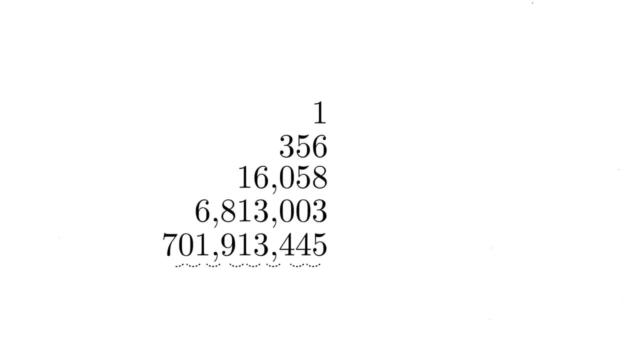 This is the feeling of slowly zooming in on the value of a number. Normally we think of the size of a number as being determined, approximately at least, by how many digits it has to the left of the decimal point. But here all the numbers have infinitely many digits. 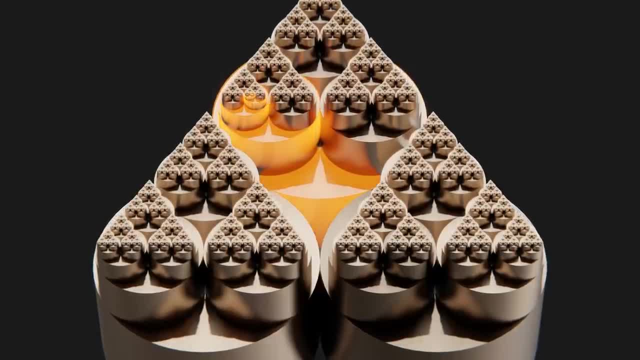 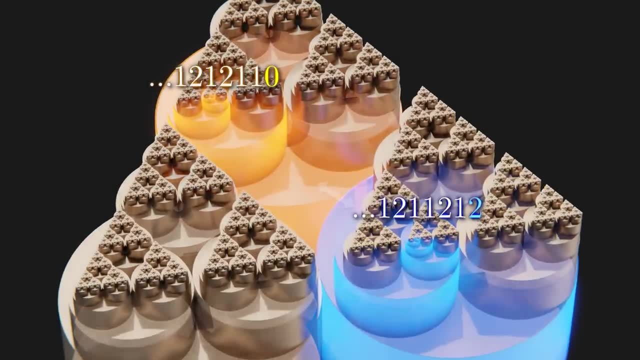 So people realize that to determine the distance between two numbers we need to look at the lowest level of the tower where they disagree. If two numbers differ in the unit's place, we say their separation is 1.. But if they differ in the 27's place, 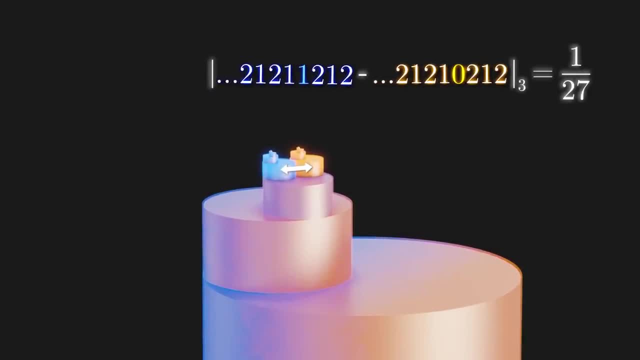 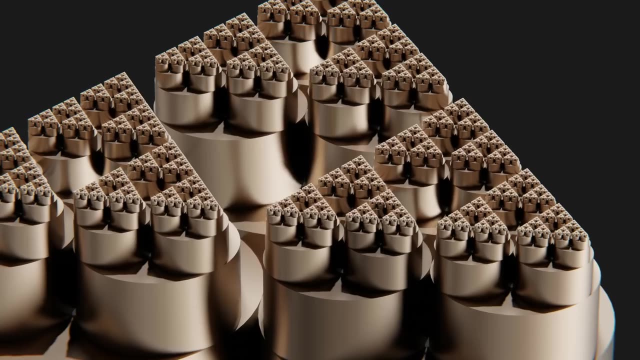 we say they differ not by 27,, but by 1 over 27.. In the world of piatics, what we're used to thinking of as big is small, and vice versa. If we have a number, let's say s1,. 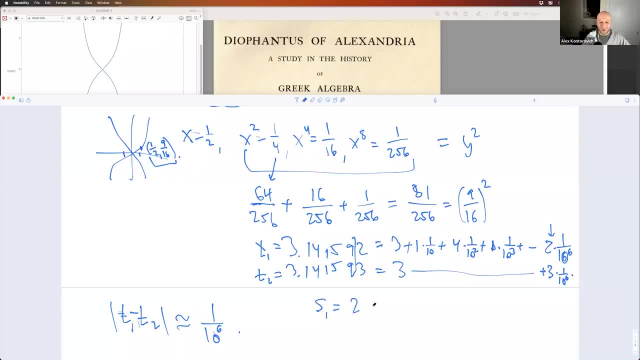 which will be some sequence like 2 times 1, plus 1 times 3, plus 0 times 3, squared plus 1 times 3, cubed, plus 2 times 3 to the fourth, and so on. we'll be close to another number with a similar expansion. 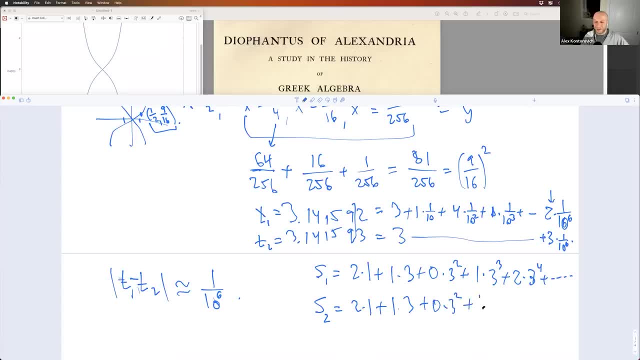 except at the, let's say, 3 to the third place. I change a digit And then it doesn't matter what I do after that. The digits can be all the same or all different. These two numbers will say that their distance. 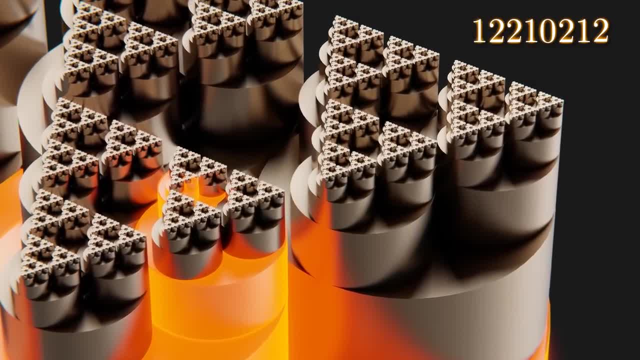 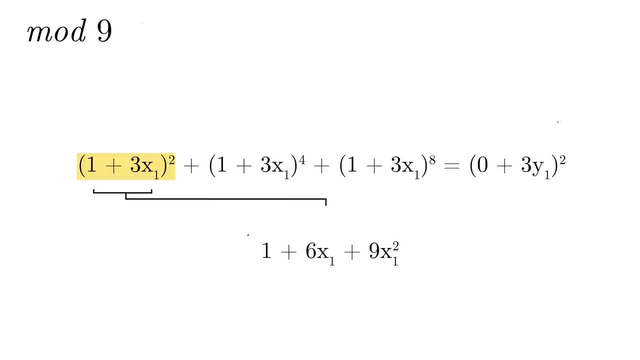 3-adic number. Contrary to what you'd expect, the coefficients multiplying higher powers of 3 actually make finer and finer adjustments. So when we calculated successive coefficients to solve Diophantus's squares problem, we were actually zooming in more and more accurately. 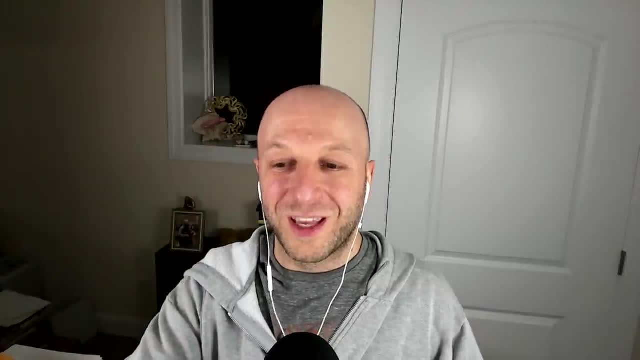 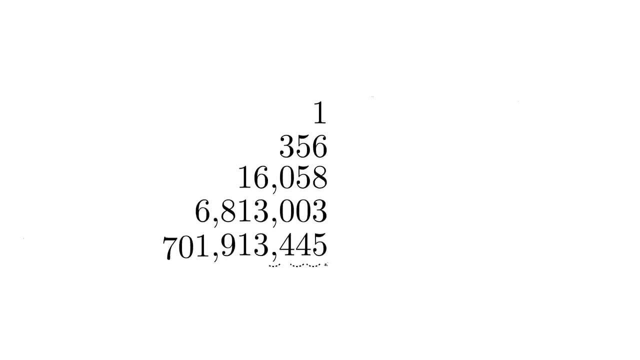 on the solution. This is the feeling of slowly zooming in on the value of a number. Normally we think of the 3-adic number as the value of a number, but in reality it's the value of a number. We don't think of the size of a number as being determined, approximately, at least, by how many. 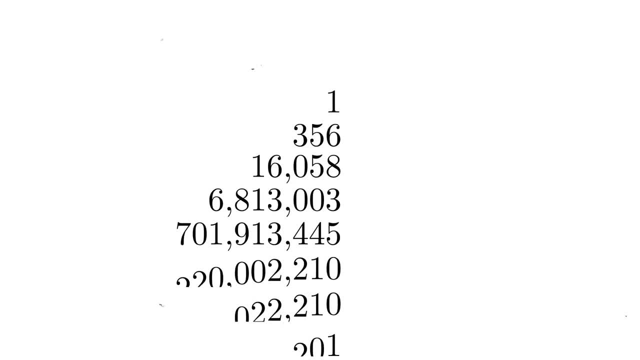 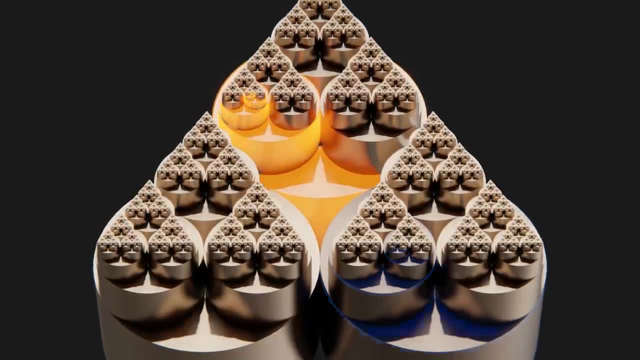 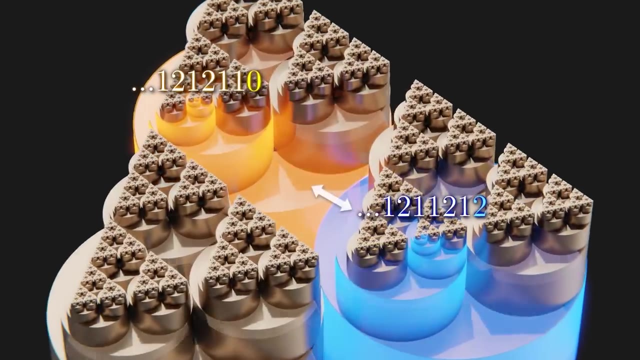 digits. it has to the left of the decimal point, But here all the numbers have infinitely many digits. So people realize that to determine the distance between two numbers we need to look at the lowest level of the tower where they disagree. If two numbers differ in the unit's place. 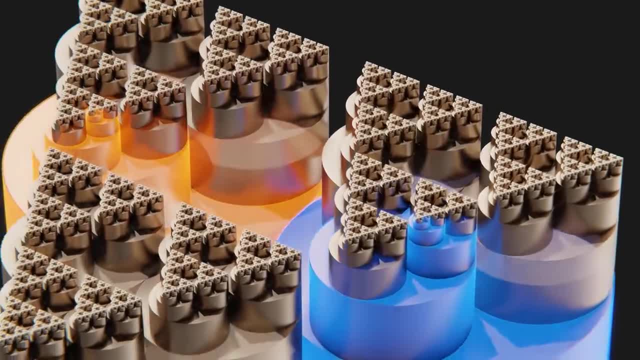 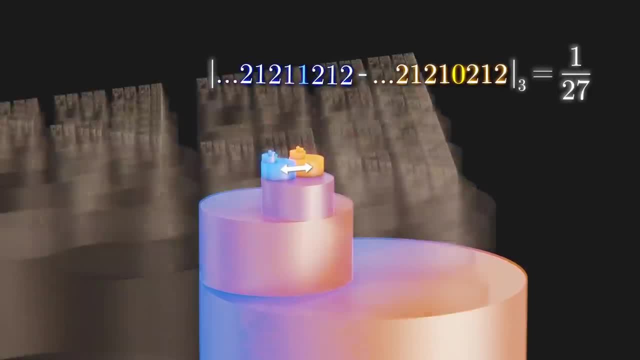 we say their separation is 1.. But if they differ in the 27's place, we say they differ not by 27,, but by 1 over 27.. In the world of piatics, what we're used to thinking of as big is small. 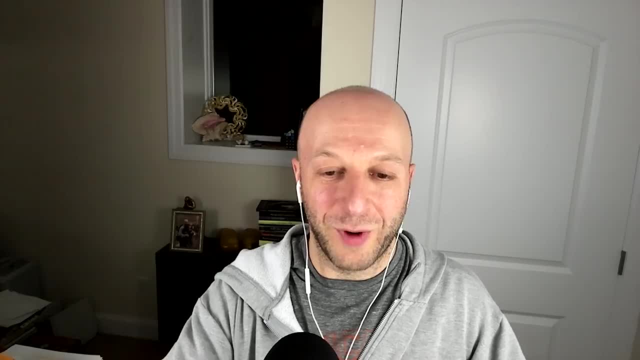 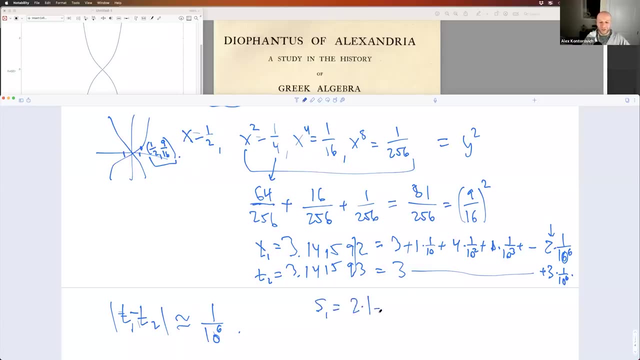 and vice versa. If we have a number, let's say s1, which will be some sequence like 2 times 1, plus 1 times 3, plus 0 times 3, squared plus 1 times 3, cubed, plus 2 times 3 to the fourth. 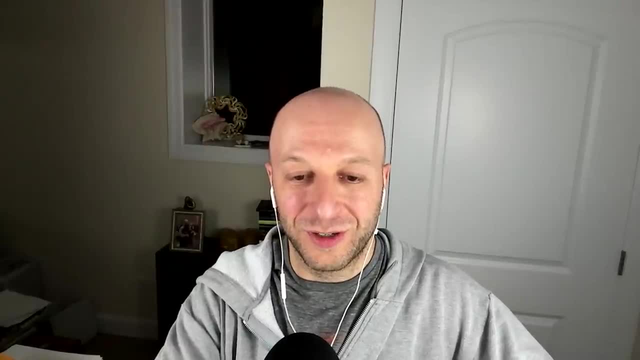 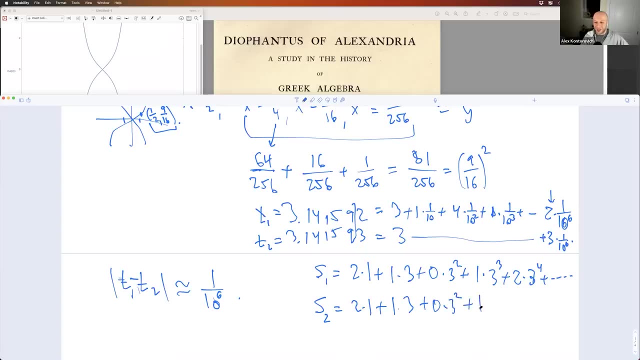 plus 1 times 1, plus 1 times 3 squared, and so on. We'll be close to another number with a similar expansion, except at the, let's say, 3. to the third place, I change a digit And then. 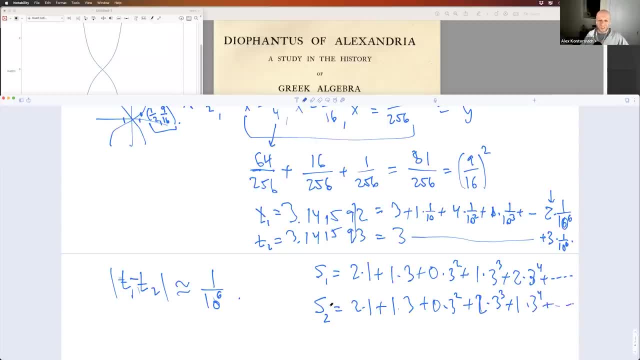 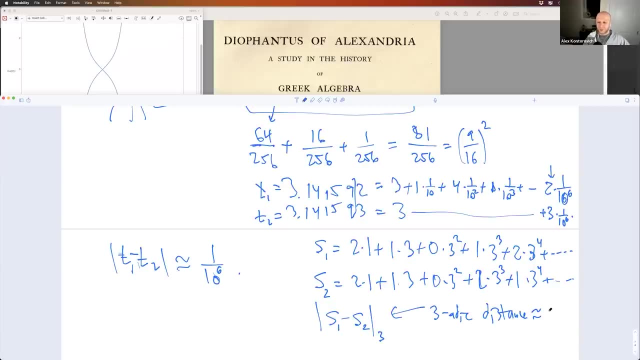 doesn't matter what I do after that. The digits can be all the same or all different. These two numbers will say that their distance, their three-adic distance, is roughly of size, the first place where they go wrong. So this will be 3 to the minus 3.. 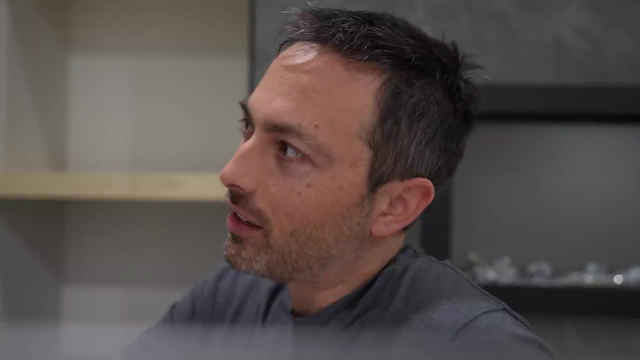 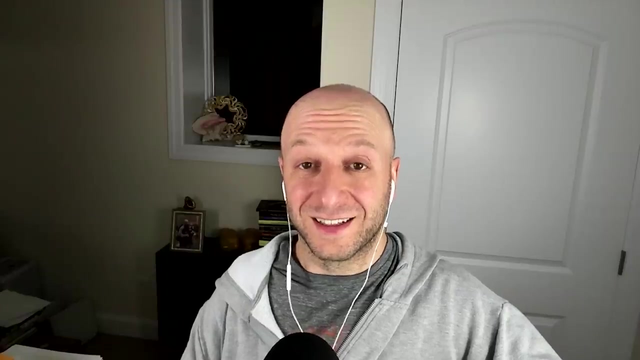 Am I supposed to think of the as kind of like: the bigger they are, the smaller the number is that they're multiplying, or something Exactly In the three addicts. we want numbers to be close when they agree up to large powers of three. 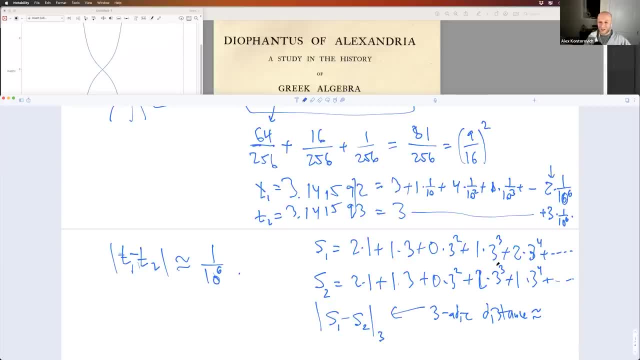 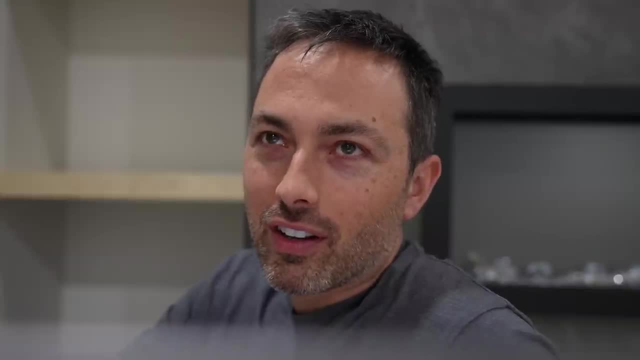 their threeadic distance is roughly of size, the first place where they go wrong. So this will be 3 to the minus 3.. Am I supposed to think of the 3's as kind of like the bigger they are, the smaller the number is? 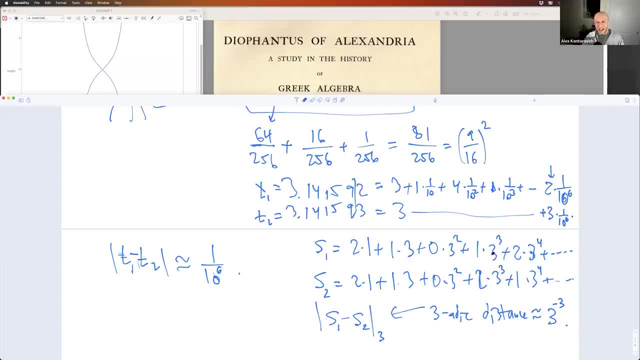 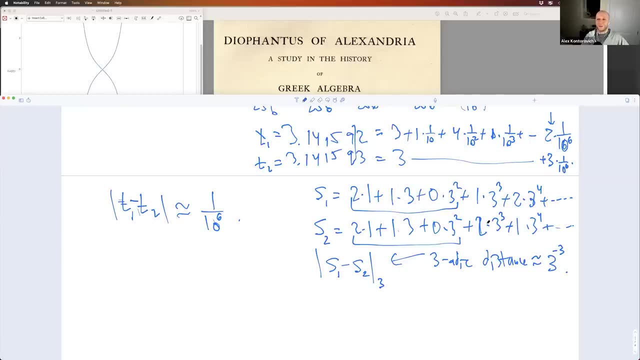 that they're multiplying or something Exactly In the three addicts. we want numbers to be close when they agree up to large powers of 3. So that if they agree up to 10 threeadic places, then this has a distance like 3 to the minus 10.. 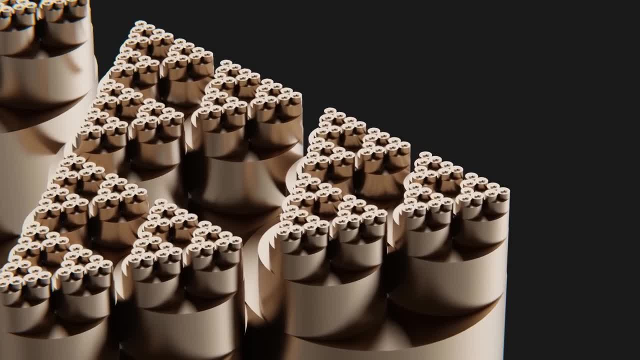 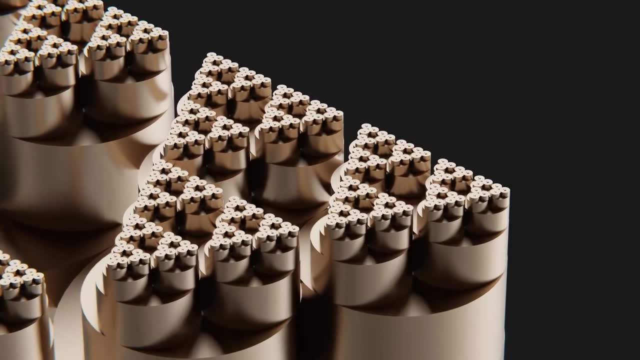 It turns out that if you do this crazy thing- swap big and small- all the other laws of mathematics work in the usual way. This is why the geometric sum worked out, even though we thought it would blow up to infinity. You have to open your mind to other notions of size. 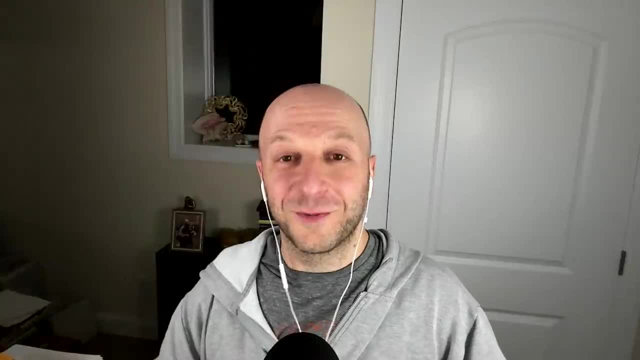 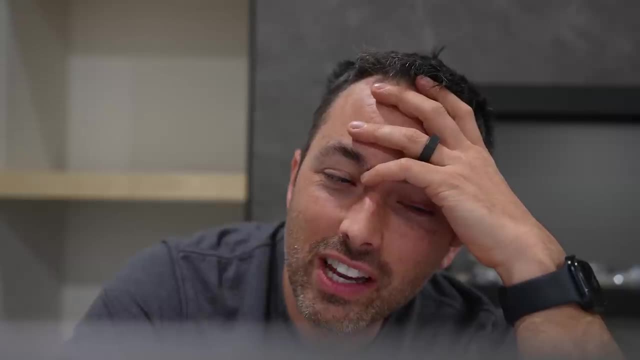 And when you do this, whole other world appears And it's a very useful world. Just like negative numbers became useful, Just like square roots of negative numbers became useful, This feels even crazier than negative numbers or square roots of negatives, Just because it's less familiar. 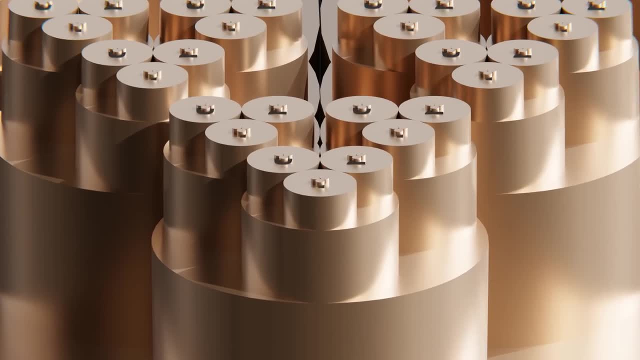 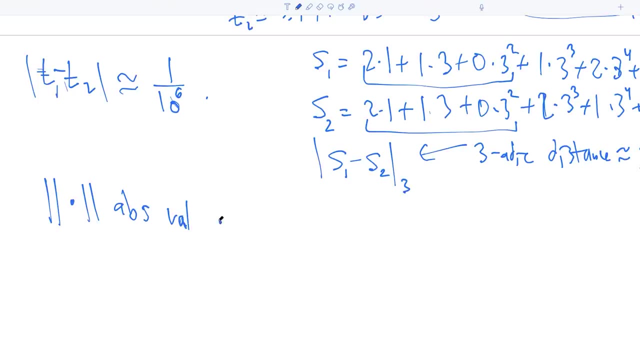 And you can prove this notion of size fits the criteria you would want for an absolute value. What do we want an absolute value to be? It should be non-negative. So the absolute value of any number, x, should be non-negative And the absolute value should be 0. 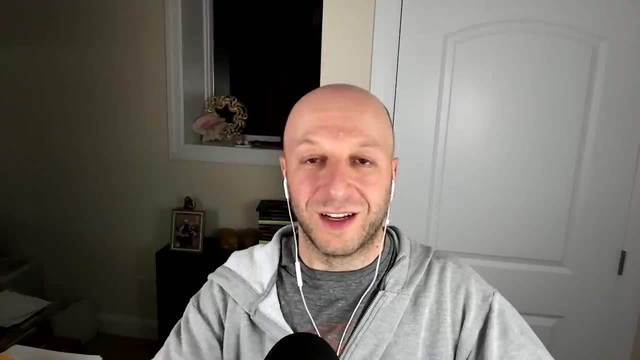 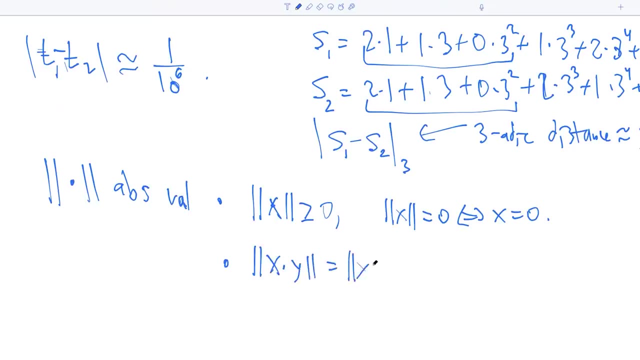 if, and only if, that number is itself 0. That's called positive definite. It should be multiplicative. If I take x times y and I multiply those two, that should be the same as the absolute value of x times the absolute value of y. 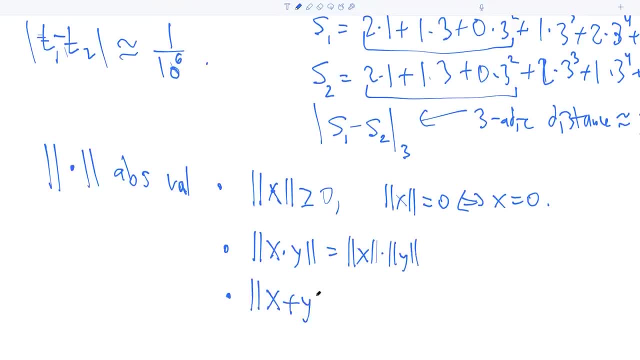 And I want one more property, which is that if you add x and y, should that be the same as the absolute value of x? No, But it should be at most the sum right. This is the triangle inequality. So we have multiplicativity, positive definiteness. 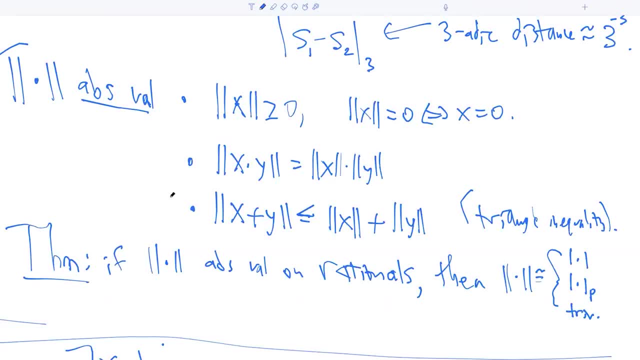 and the triangle inequality. You give me only these three very abstract things, and I can prove that your function is in fact the usual absolute value, or one of these p-adic absolute values, or the thing that gives 0 to 0 and 1 to everything else. 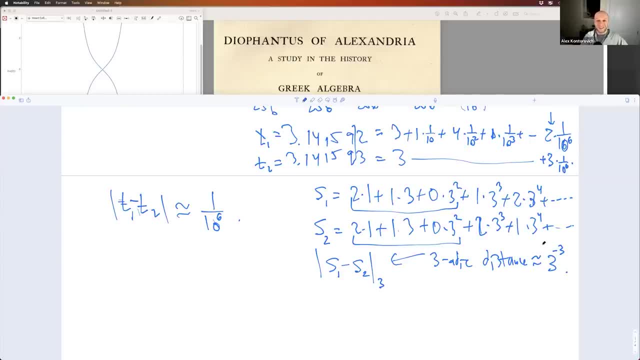 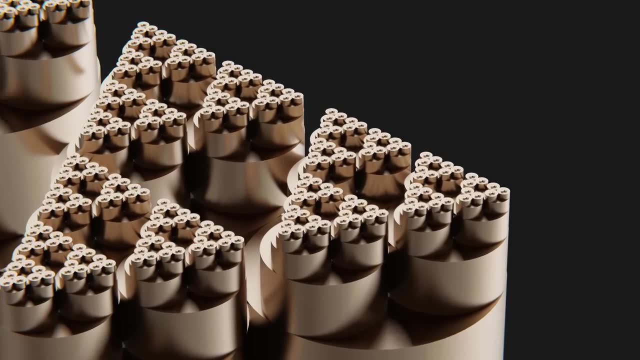 So that if they agree up to 10, three addict places, then this has a distance like three to the minus 10.. It turns out that if you do this crazy thing- swap big and small- all the other laws of mathematics work in the usual way. 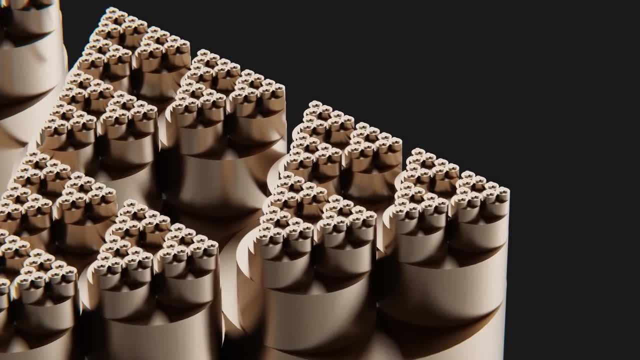 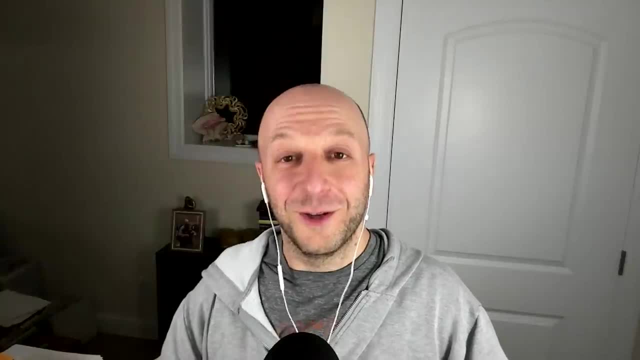 This is why the geometric sum worked out, even though we thought it would blow up to infinity. You have to open your mind to other notions of size And when you do this, whole other world appears And it's a very useful world, Just like negative numbers became useful. 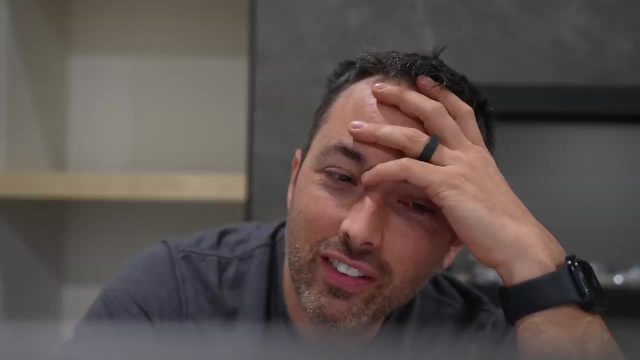 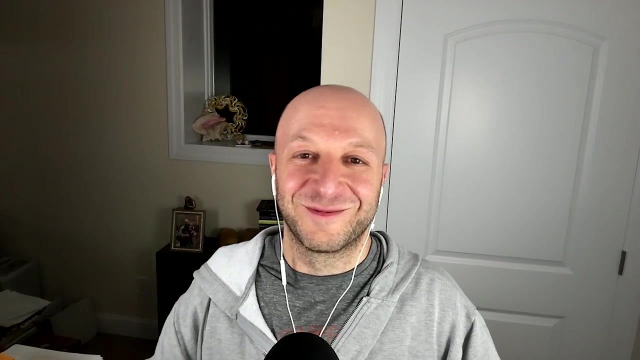 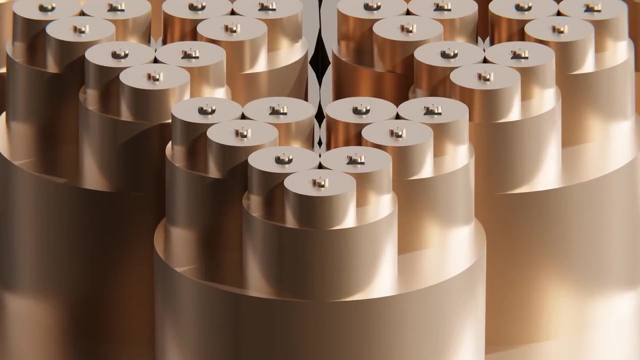 just like square roots of negative numbers became useful. This feels even crazier than negative numbers or square roots of negatives, Just because it's less familiar And you can prove this notion of size fits the criteria you would want for an absolute value. What do we want an absolute value to be? 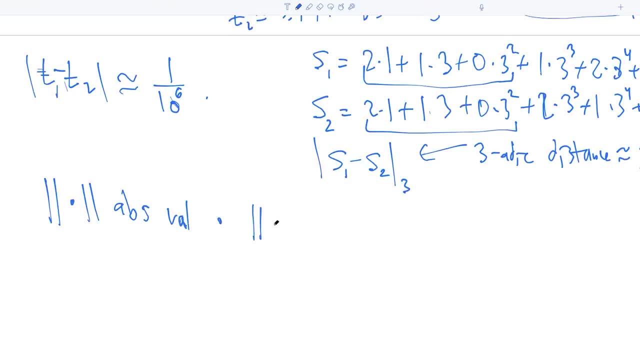 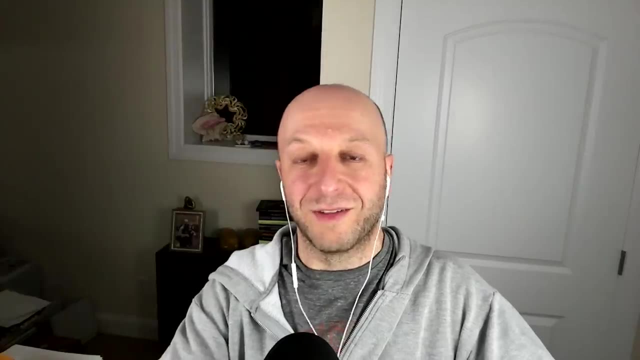 It should be non-negative. So the absolute value of any number, X, should be non-negative, and the absolute value should be zero if, and only if, that number is itself zero. So that's called positive definite. So it should be multiplicative. If I take X times Y and I multiply those two. 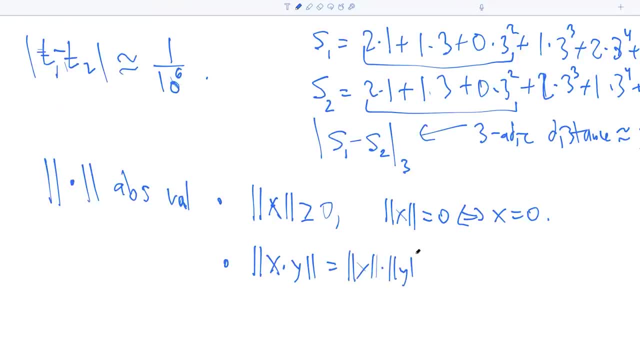 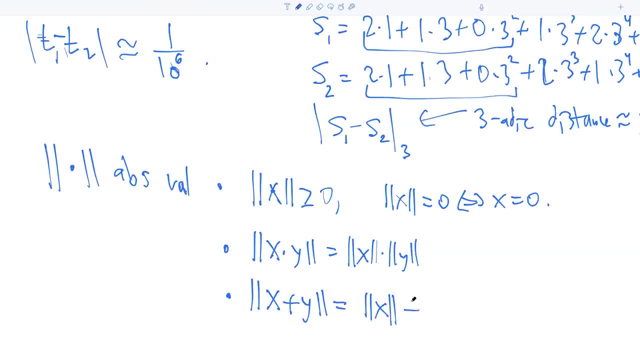 that should be the same as the absolute value of X times the absolute value of Y. And I want one more property, which is that if you add X and Y, should that be the same As the absolute value of X plus the absolute value of Y? 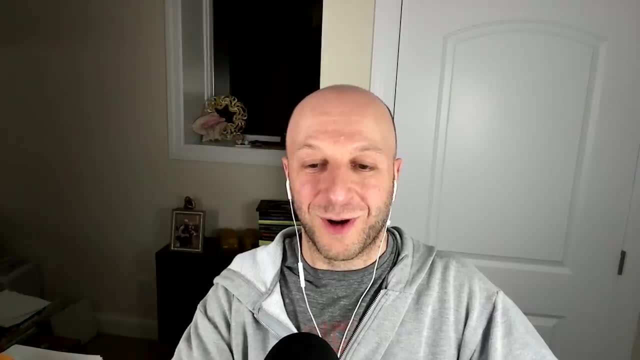 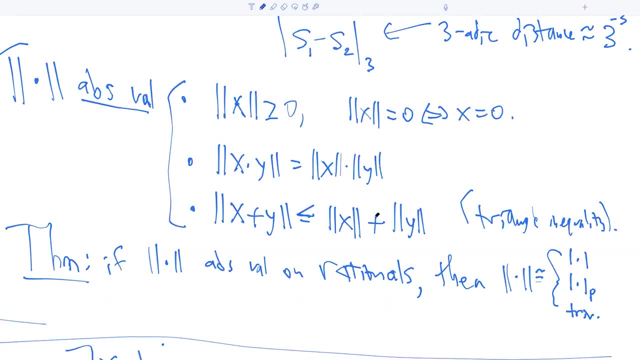 No, but it should be at most the sum right. This is the triangle inequality. So we have multiplicativity, positive definiteness and the triangle inequality. You give me only these three very abstract things and I can prove that your function is in fact. 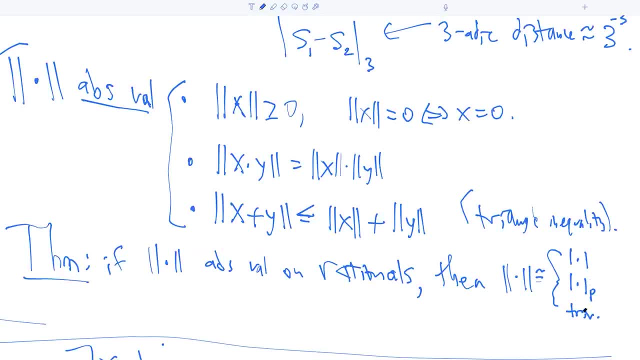 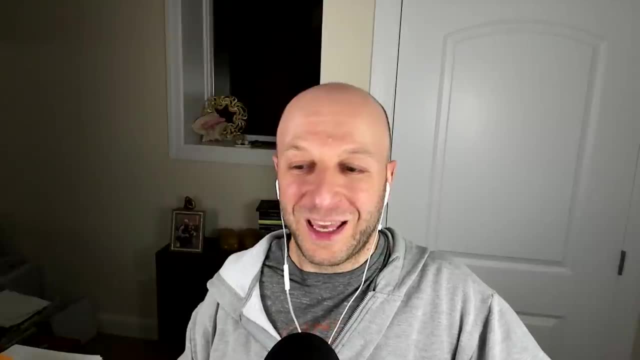 the usual absolute value, or one of these p-adic absolute values, or the thing that gives zero to zero and one to everything else. So that's the trivial absolute value. These are the only games you can play on the rational numbers. They give you absolute values that behave the way we want them to. 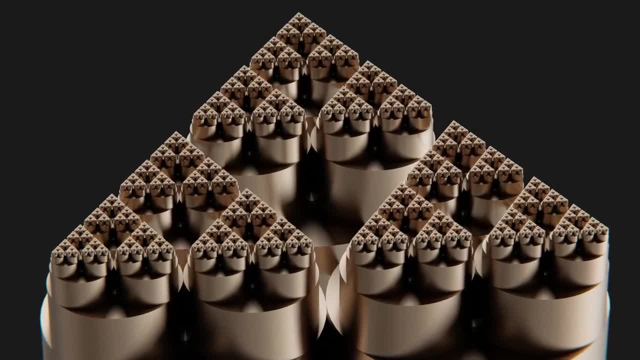 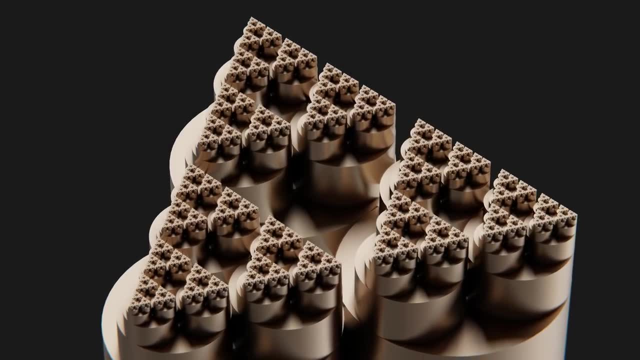 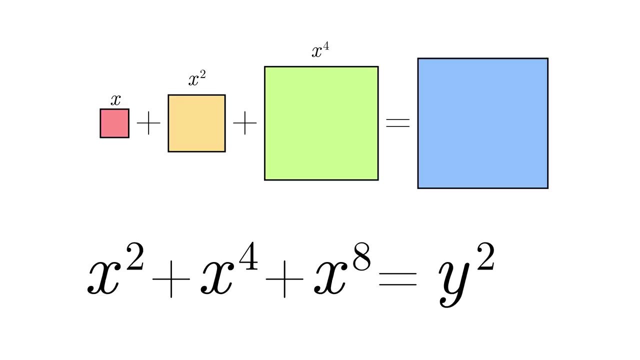 This geometry makes the p-adics much more disconnected when compared to the real numbers, And this is actually useful for finding rational solutions to an equation. There are many fewer p-adic solutions in a neighborhood of a rational solution If we tried the same strategy of solving Diophantis' squares problem. 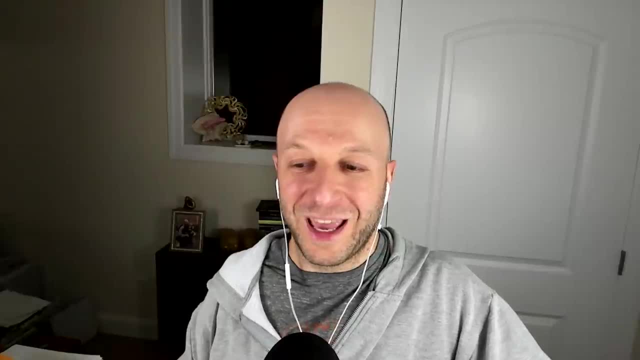 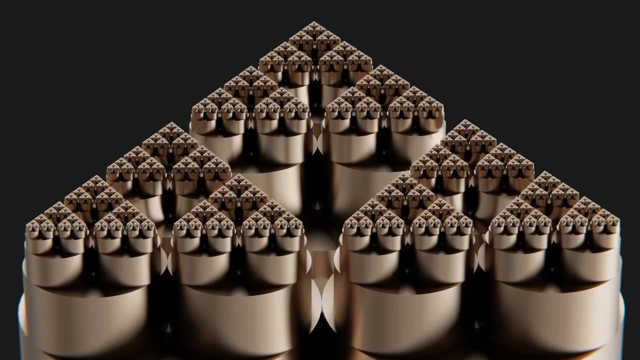 So that's the trivial absolute value. These are the only games you can play on the rational numbers that give you absolute values that behave the way we want them to. This geometry makes the p-adics much more disconnected when compared to the real numbers. 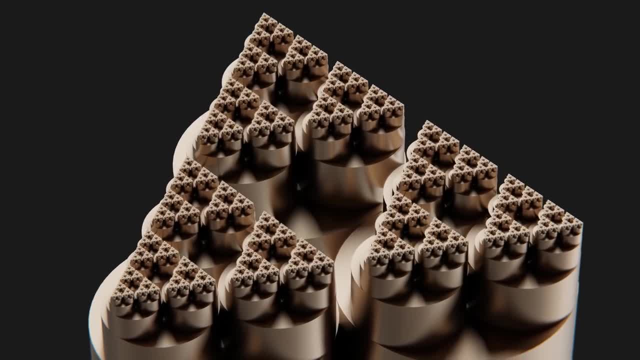 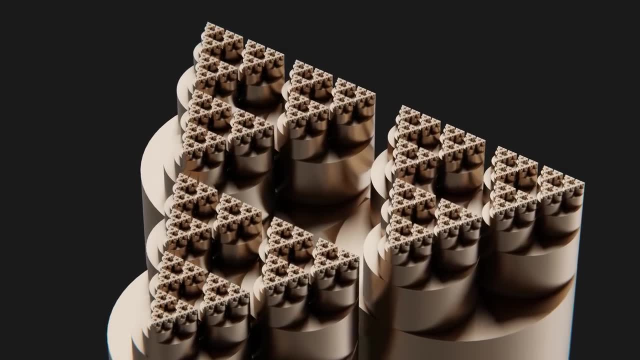 And this is actually useful for finding rational solutions to an equation. There are many fewer p-adic solutions in a neighborhood of a rational solution If we tried the same strategy of solving Diophantus' squares problem digit by digit in the real numbers. 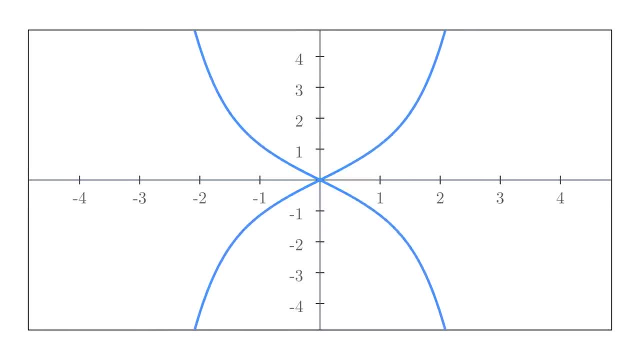 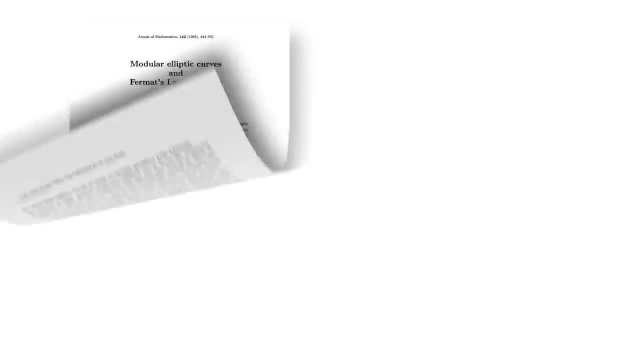 it would be doomed to fail because there are simply too many real solutions all over the place. They get in the way In a groundbreaking pair of papers in 1995, one by Andrew Wiles and another by Wiles and Richard Taylor. 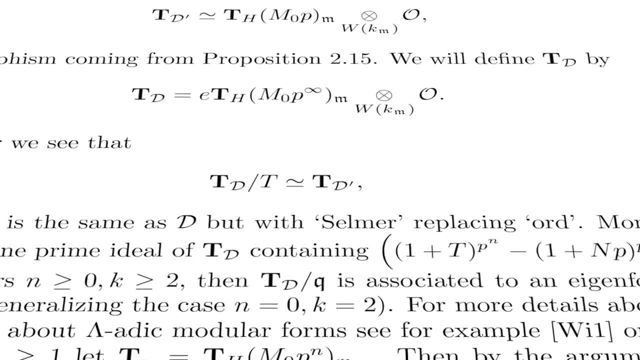 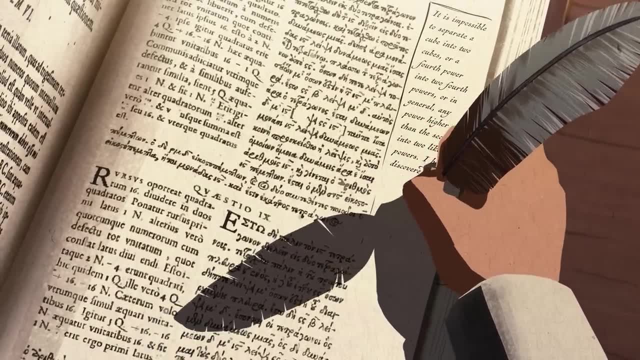 they finally proved Fermat's Last Theorem, But the proof could not possibly have been the one Fermat alluded to in the margin, because it made heavy use of p-adic numbers. Wiles' proof of Fermat's Last Theorem. 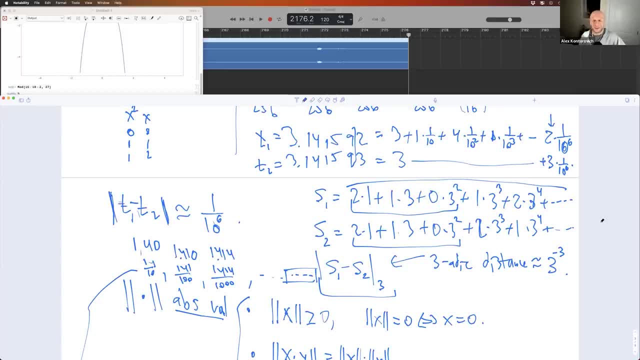 used the prime 3, and then at some point he got stuck with the prime 3, and he had to switch to the prime 5.. And this is literally called the 3-5 trick. There was something that worked for the prime 3. 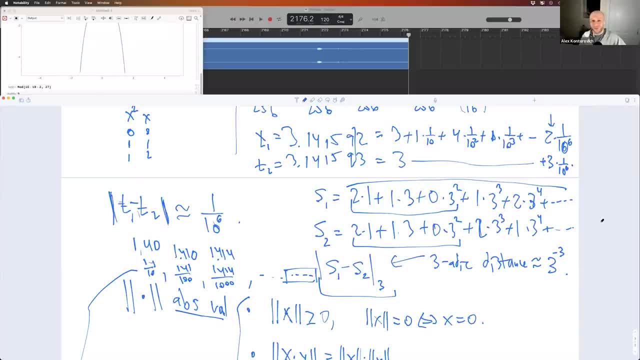 most of the time, but sometimes it didn't work, and when it didn't work for the prime 3, it did work for the prime 5.. Each prime gives you a completely unrelated number system, just like these number systems are unrelated to the real numbers. 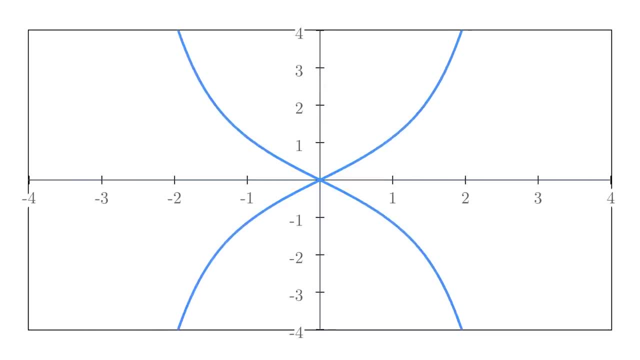 digit by digit in the real numbers, it would be doomed to fail because there are simply too many real solutions all over the place. They get in the way In a groundbreaking pair of papers in 1995, one by Andrew Wiles and another by Wiles and Richard Taylor. 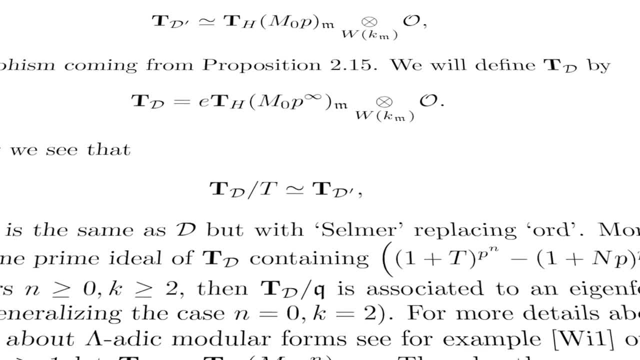 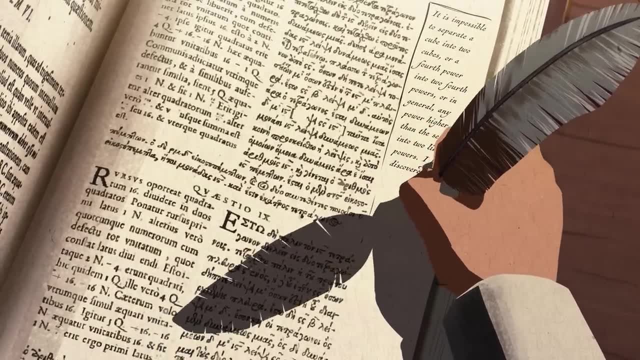 they finally proved Fermat's Last Theorem, But the proof could not possibly have been the one Fermat alluded to in the margin, because it made heavy use of p-adic numbers. Wiles' proof of Fermat's Last Theorem used the prime 3. 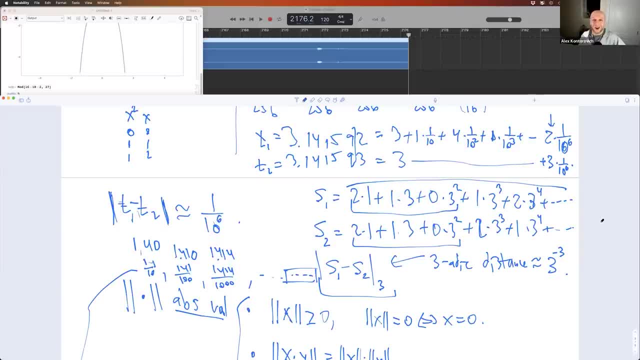 and then at some point he got stuck with the prime 3 and he had to switch to the prime 5. And this is literally called the 3-5 trick. There was something that worked for the prime 3 most of the time, but sometimes it didn't work. 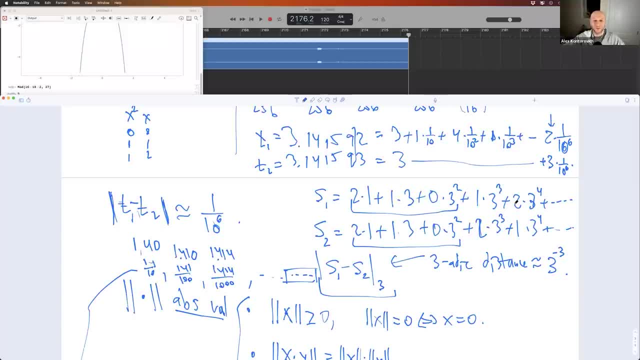 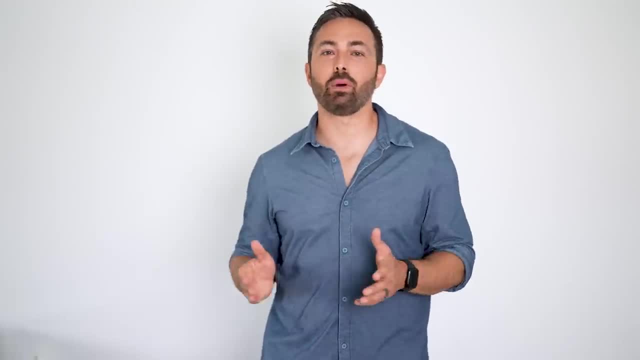 and when it didn't work for the prime 3, it did work for the prime 5.. Each prime gives you a completely unrelated number system, just like these number systems are unrelated to the real numbers. There is a great quote, I like, by a Japanese mathematician. 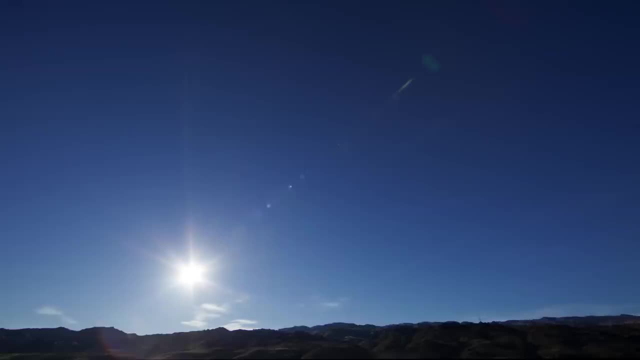 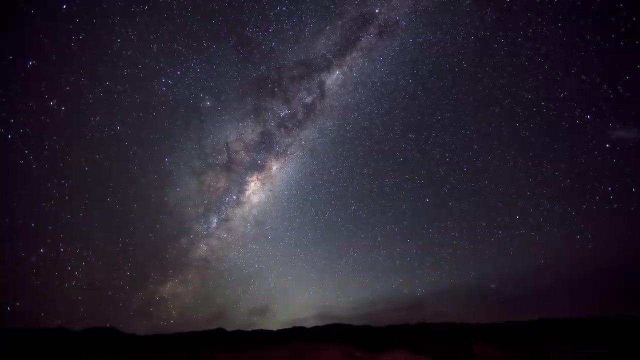 Kazuya Kato. He says Real numbers are like the sun and the p-adics are like the stars. The sun blocks out the stars during the day and humans are asleep at night and don't see the stars, Even though they are just as important. 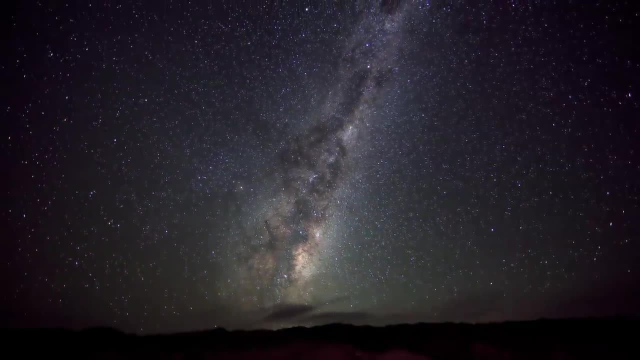 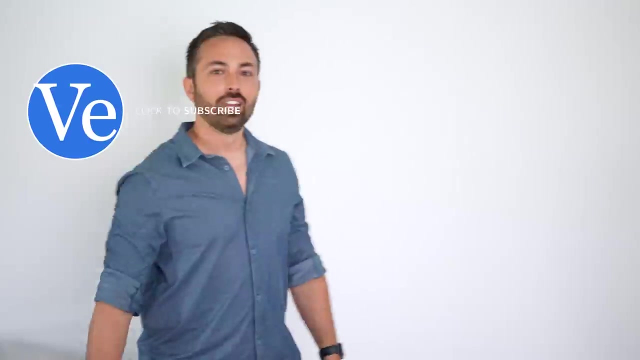 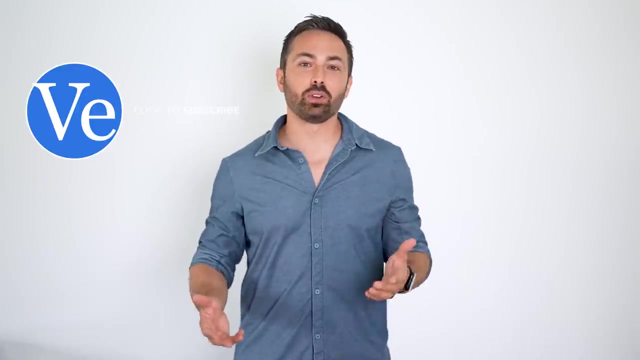 Well, I hope this video has revealed at least a glimpse of those stars to you. The discovery of p-adic numbers is a great reminder of just how much we have yet to discover in mathematics, Not to mention science, computer science and just about every technical field. 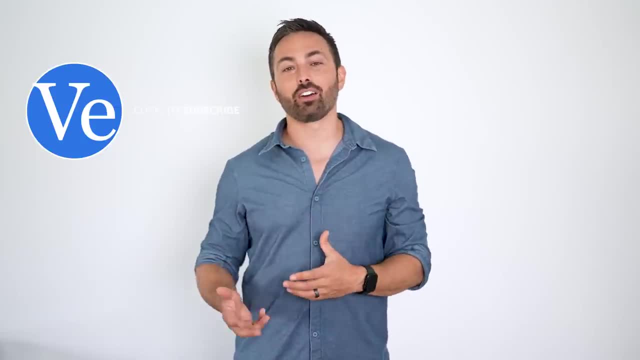 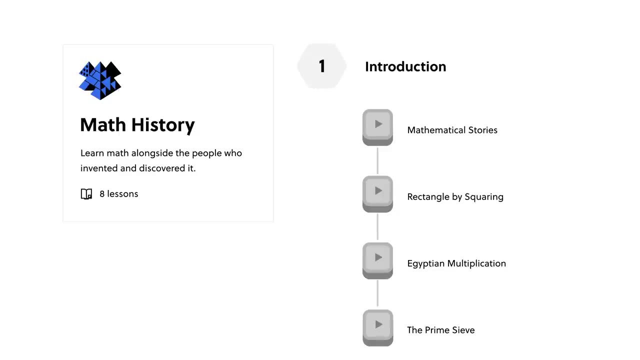 They inspire us to find new connections and even make discoveries ourselves. If you were inspired by the stories of Diophantus, Fermat and Hensel and you're looking for more content like this, look no further than the math history course from this video's sponsor, Brilliantorg. 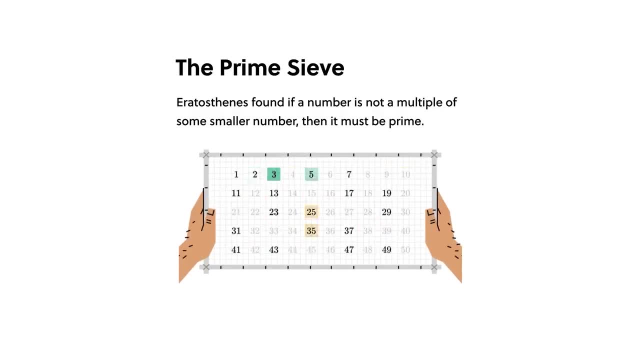 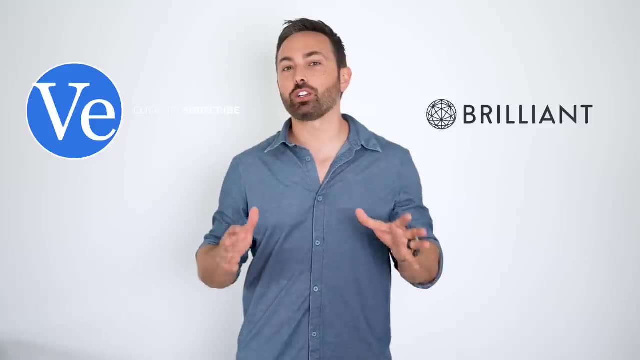 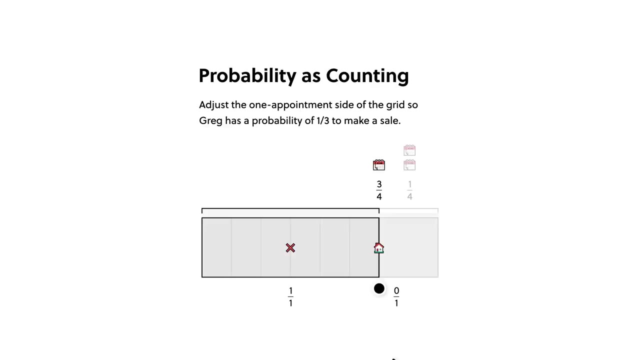 Brilliant's course introduces you to the minds behind some of the most fascinating discoveries in mathematics, while giving you a deeper understanding of the concepts they pioneered, all of which enable our modern technologies. Brilliant actually has thousands of bite-sized lessons on everything from math and science to data programming and computer science. 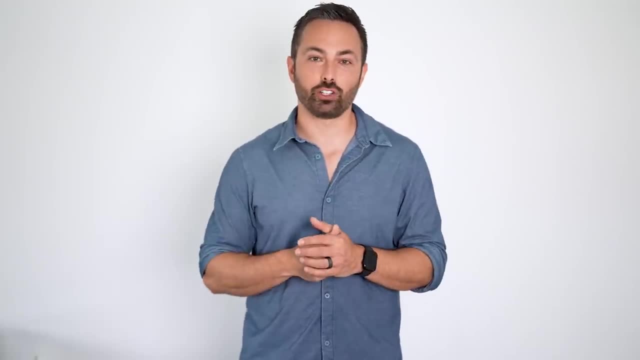 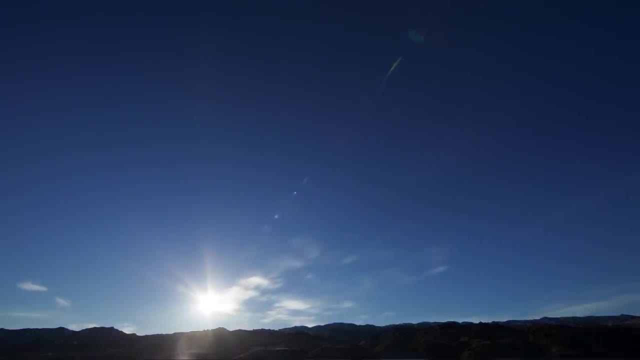 There is a great quote I like by a Japanese mathematician, Kazuya Kato. He says: Real numbers are like the sun and the p-atics are like the stars. The sun blocks out the stars during the day and humans are asleep at night. 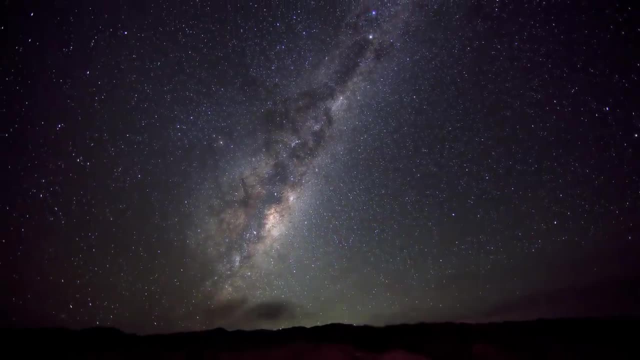 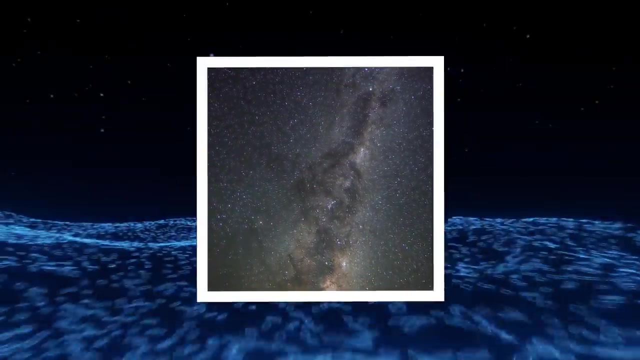 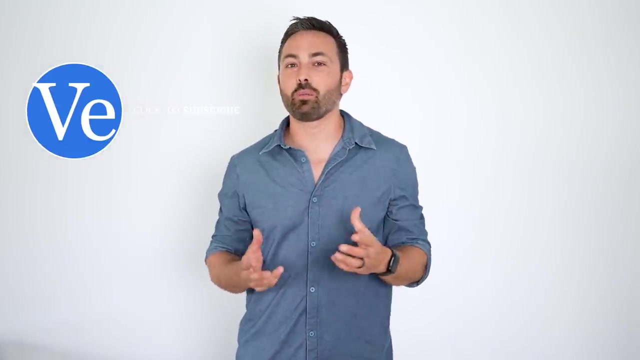 and don't see the stars, even though they are just as important. Well, I hope this video has revealed at least a glimpse of those stars to you. The discovery of p-adic numbers is a great reminder of just how much we have yet to discover in mathematics.